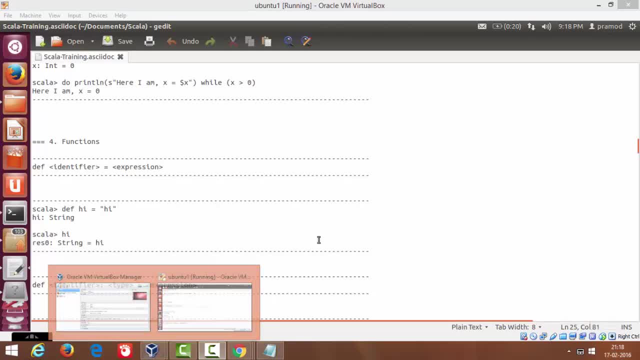 Okay, let's do a recap on what all we did. We said that. why functional programming? Functional programming is nothing but immutability. Immutability is very good for parallel programming. We saw that the discrepancies happen because there is parallel programming and mutable state. 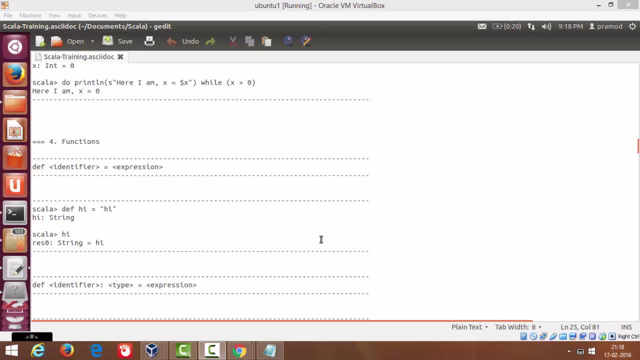 Whenever there is a mutable state, you need to put a lot of logs and all to maintain the concurrency in your programming. So that's a tougher thing, And if you maintain immutability then it's become much easier. And immutability means here functional programming, And Scala is a good at functional programming And also it is a pure object oriented programming. 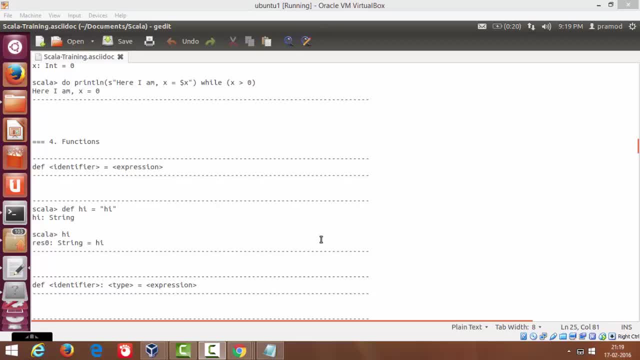 So we need to. That's what is all about the functional programming, and Scala is functional programming language. Scala is also type inferred means it will infer the type for you. You need not specify the type. Even though you want to specify the type, you can give it at the last. Whenever you are declaring an identifier or you are declaring a function, defining a function, the return type or the data types will always come at the end. 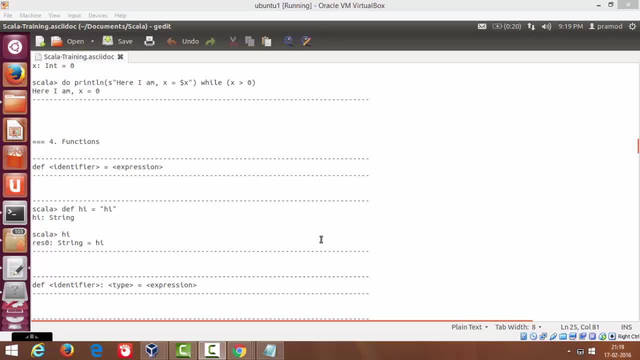 Last. Then we saw it is statically typed language. That's because the data type is always inferred and it knows what data type is, what identifiers or functions is all about And based on that it can resolve most of the errors at the compile time itself. Syntactic errors or some runtime errors in some other language could be resolved at the compile time itself. That's a big gain. 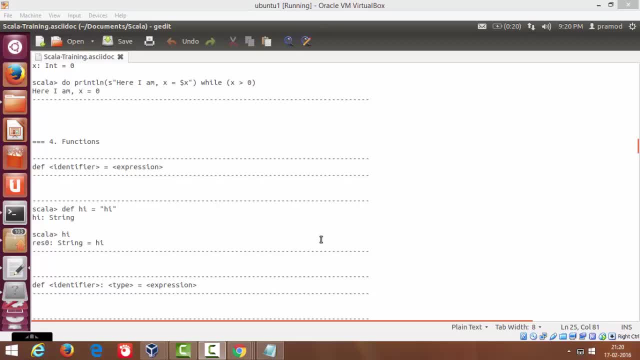 On programming languages. Then we saw normal variables, how everything like basic data types. Then we saw val, then we saw var. Val means constant And Scala, as I said, by default supports immutability. It means all the Scala collections are by default immutable. 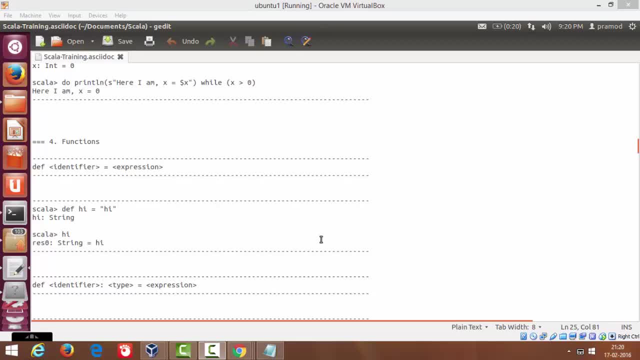 You have to explicitly ask for it. Even val is immutable. That is, whenever you declare any private variable in a class, that is by default immutable. If you don't specify val or var for members of a class, those are all by default immutable. That's what makes Scala languages immutable. 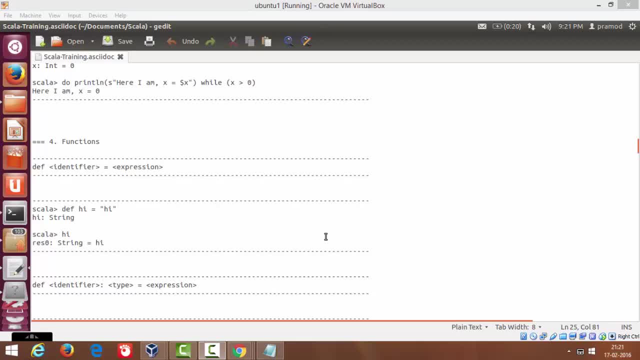 Then we saw normal basic data types like int, w, etc. Double strings. Then we saw if conditions for comprehensions. We also said that the for comprehensions are much more powerful than for loops in any other languages because underneath it is executed, implemented using higher order functions. 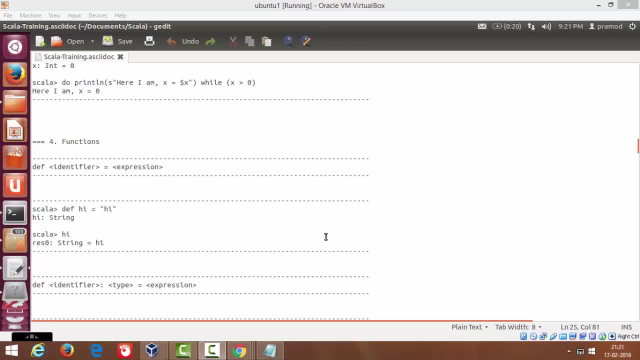 Just remember as of now, because we will cover more of higher order functions later. But just remember that, for comprehensions are underneath implemented with Higher order functions And we also saw how pattern matching is done in Scala. Even it is much more powerful than the switch cases in other other languages. 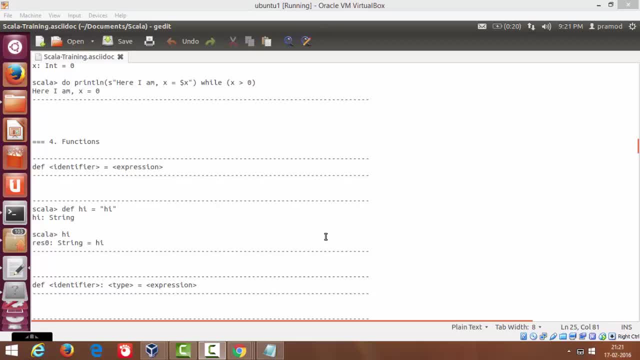 You can pattern match on literals. We can pattern match on variable binding. We can pattern match on underscores. Those are underscores and variable bindings are the wildcard pattern matching. So you can also have, once you have Variable binding, we can have pattern guards, which are nothing but if conditions on the pattern matching. 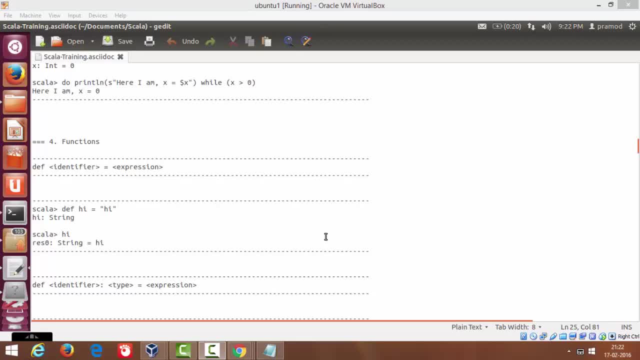 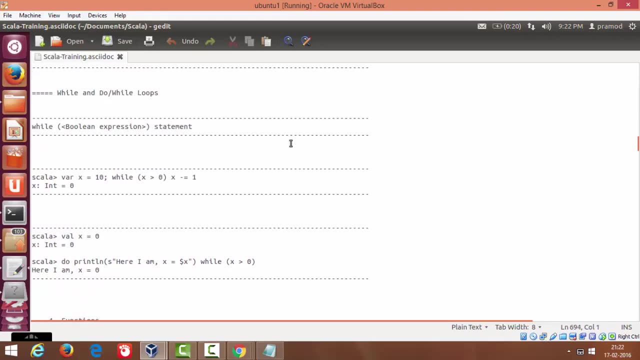 So these are things we saw in our previous sessions. We also saw if else conditions- If at all, there is only if condition. we saw that the return value is always any. I hope we covered all those things right. We were supposed to start from functions, right. 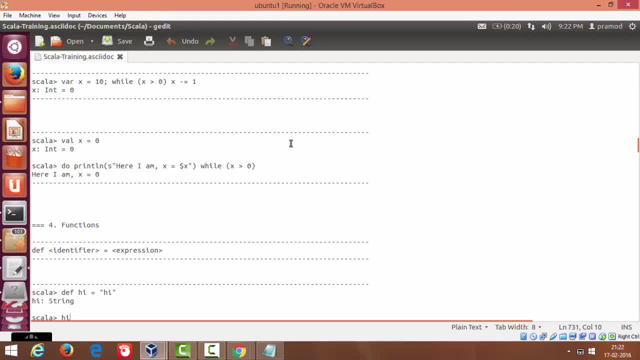 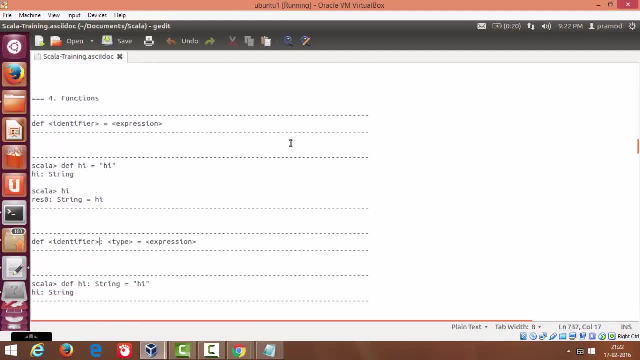 Let's go with simple functions. And one more thing in functions is: functions are called first class citizen Scala. What that means is all functions in Scala are implemented as objects Are implemented using classes, and all functions are treated as a result. All functions are objects. 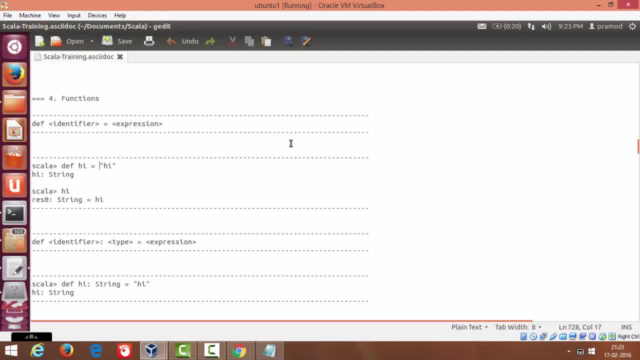 So whenever all functions are objects, objects can be assigned to any other objects, so functions could be assigned to any other variables identifiers. functions could be passed as a parameter to another function. function could be returned from a function functions body that is called function. literal could be passed as a very passed as a parameter to a functions. 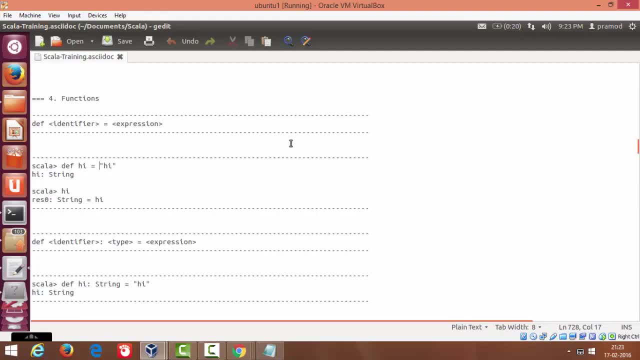 So all these could be possible. That's because functions are implemented as classes, which results in function objects. So let's see how a simple function looks like. This is our simple function. Def is the keyword, Then we have the function name. 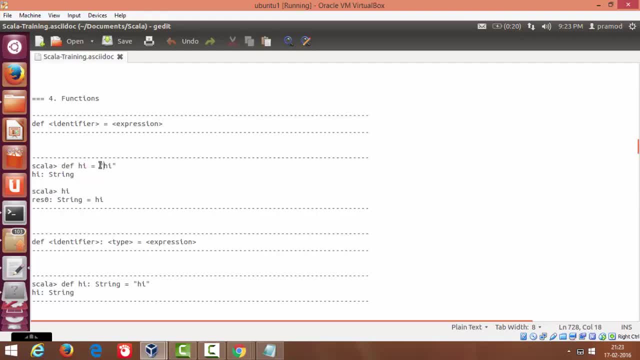 Then we have equal to sign. Then this here is the body of the function. You can have a single line body or usually multiline body. So we can. We can get rid of If it is a single expression. we can get rid of the open bracket and close bracket. 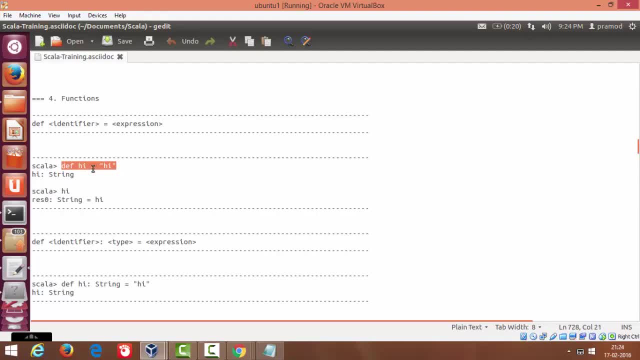 This is a simple definition of a function, and the function name and the body is differentiated by the equal to sign. The equal to sign comes because we say that in Scala everything is an expression, So you have to always return something from an expression. 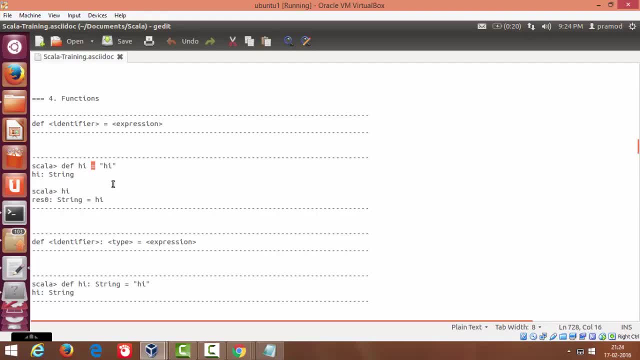 And we are assigning those return values, Return value to something else. So this is how a function syntax looks like. We have a def keyword, identifier, Any name, The data type has to be specified, Otherwise it means it's not mandatory to specify because this is the return data type of the function. 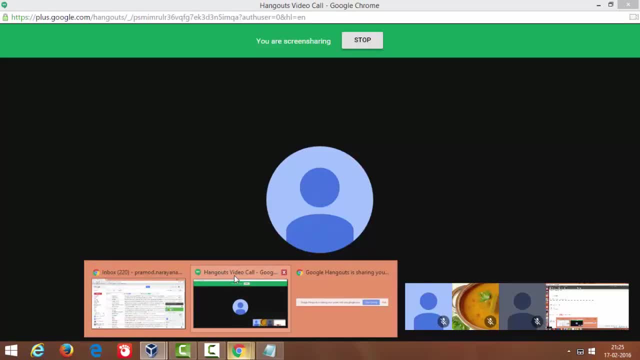 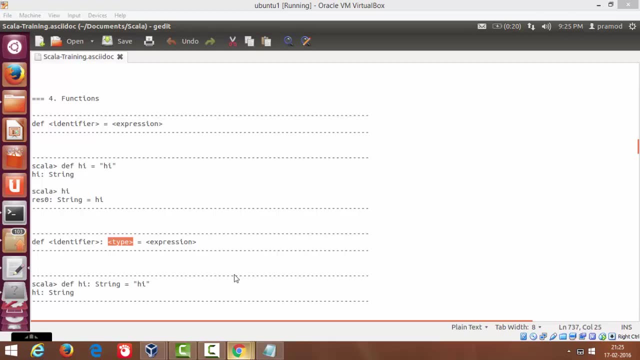 Yeah, Any questions? No, Okay, This is the return type of the function, which is optional because the return type is always inferred from the function, inferred from the body of the function, Whatever is the last expression in the body of the function. 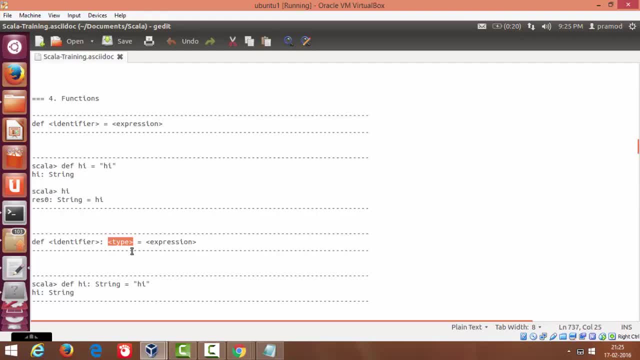 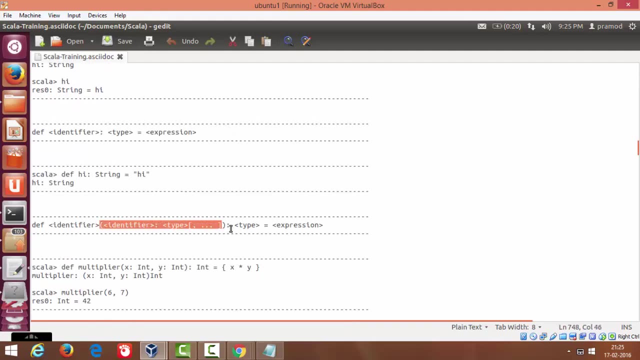 After evaluating that expression, Whatever is the data type, That is the data type, Return data type of the function. So these are parameters, related functions. You can pass the parameter. If we are not specifying any parameter, you need not specify open bracket and close bracket. 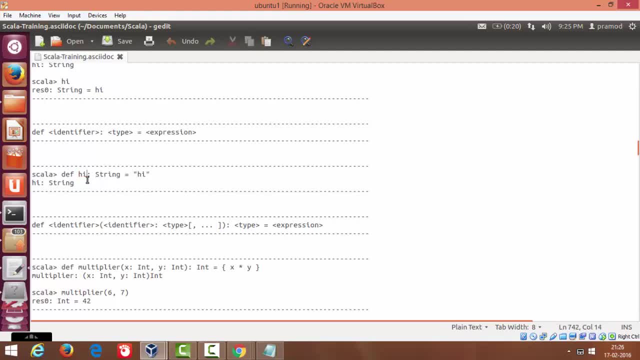 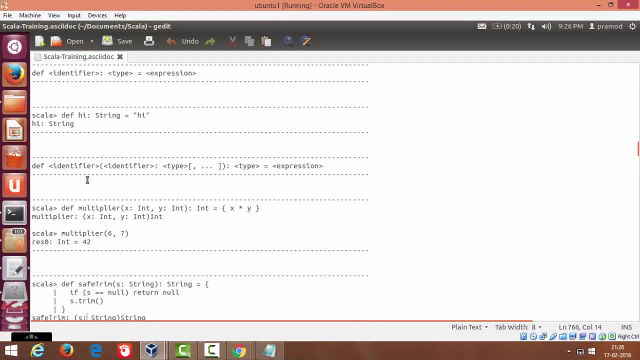 So those are all got rid of. There is also no return statement in the body of the function. Let's take the simple example. We have a def multiplier, We are passing int, xint, yint, and the return type is int and the body is x, star y expression. 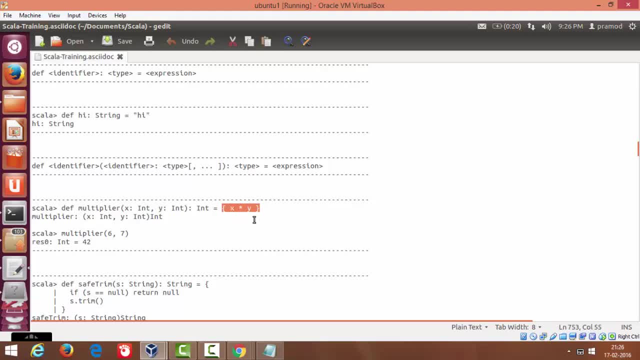 So we see, we are seeing that there is no return keyword here in the body of the function because it's not required. It is redundant, but it could be specified. It's optional. It's better not to specify it. And also, whatever is the last expression in the block that will be evaluated and returned and based on that return data type. 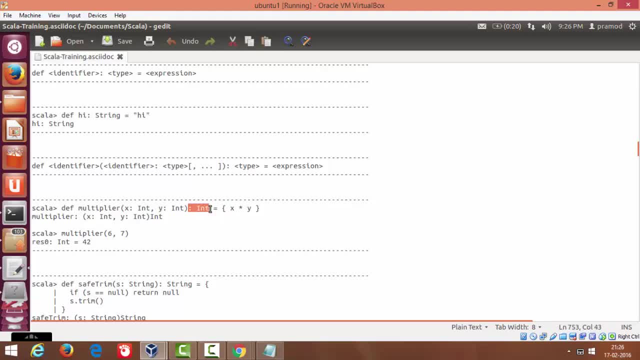 Scala compiler will automatically infer it here. I have given it, but it is not required at all, But whenever we. But these two are redundant, But these two are required always, Otherwise we don't. We cannot differentiate between function overloading. 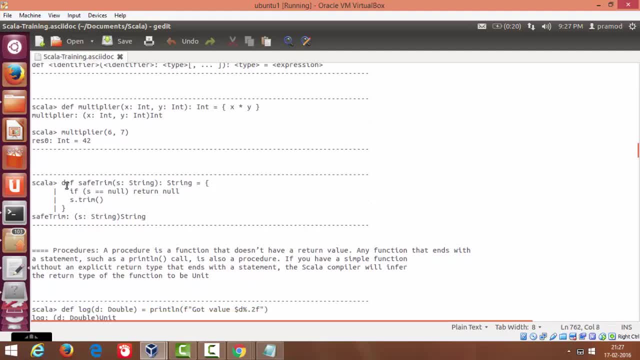 This is one more simple sample example, So these examples will be using later in our higher order function. That's the reason I have put it here. This is a function that takes a string and returns a string And if it is, the string is null and returning null. 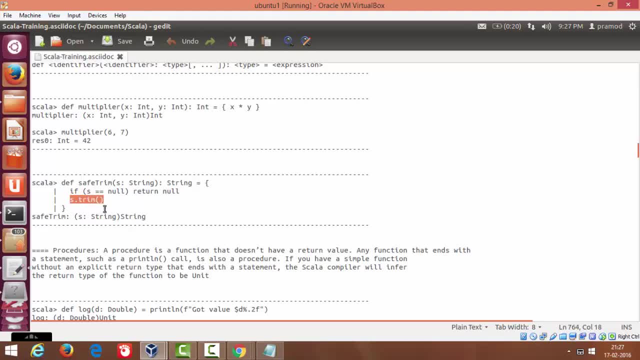 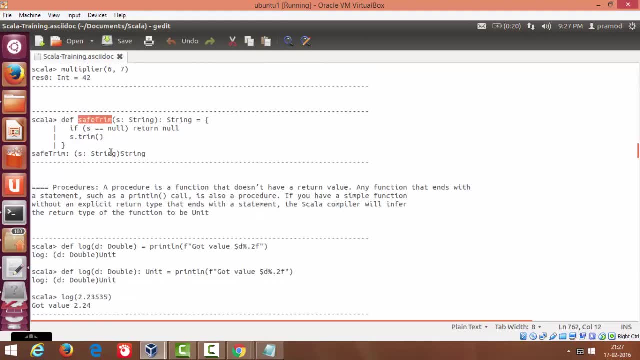 Otherwise we are trimming it and returning whatever is the value, Whatever we pass to the string, To this function. Sorry, Yeah, These are all like just to remember that a procedure is a function that doesn't have a return value, Not much of a significance. probably in interviews that maybe they may be asked. 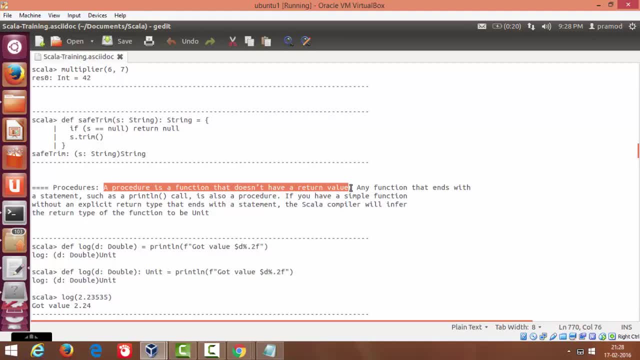 But the procedure is a function that doesn't have a return value. Any function that ends with a statement. As I said, a statement is an expression that does not return anything. So, if at all, a function has the last statement, last expression, as a statement. 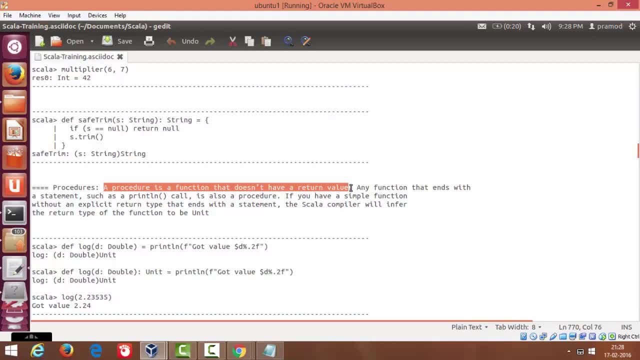 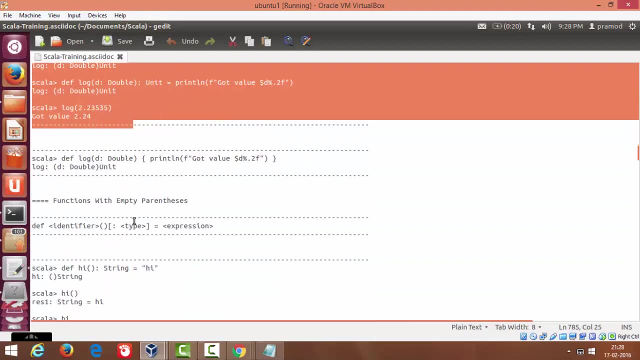 Then that function will be a procedure. Okay, So these are all things not required Means just to remember that Difference between functions and procedures. Yeah, Function with empty parenthesis, These are all optional. That's what we saw in the beginning. 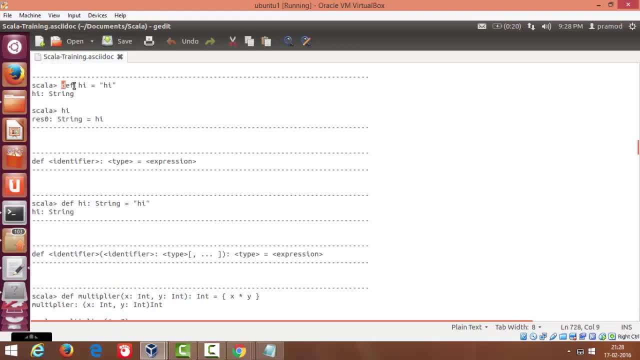 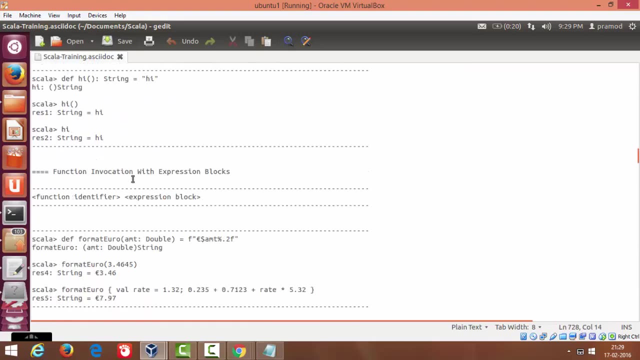 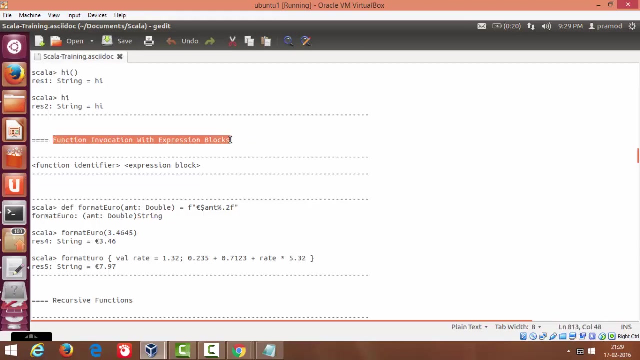 If you see this, This is the function. that doesn't have any parenthesis, It is always optional. You may specify or may not specify, It's one and the same Function: invocation with expression blocks. So, if you see, here We have a function. 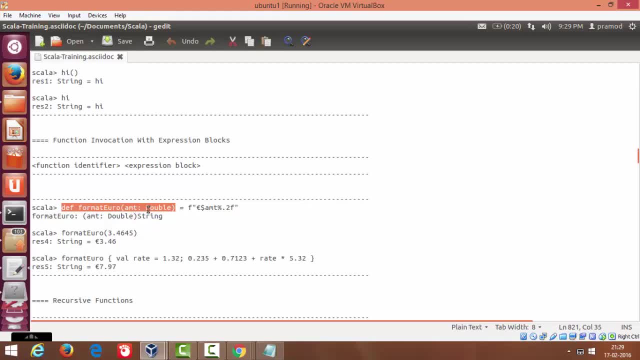 Which takes A parameter. So, instead of Directly passing a parameter to this function while calling this function this way, This is one way of calling the function: We pass the parameter Exact value or some value, Or we Pass an. 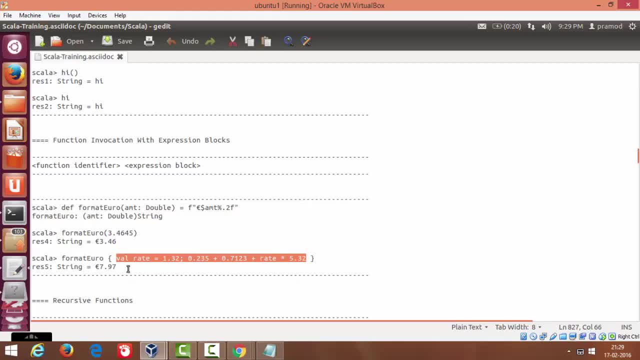 Expression After. whatever this expression is evaluated, The last value will be Passed as a parameter to this function. This is also possible, So whenever we specify an expression, we need to have Open flower back it and close flower back it. Otherwise, this is a normal way of. 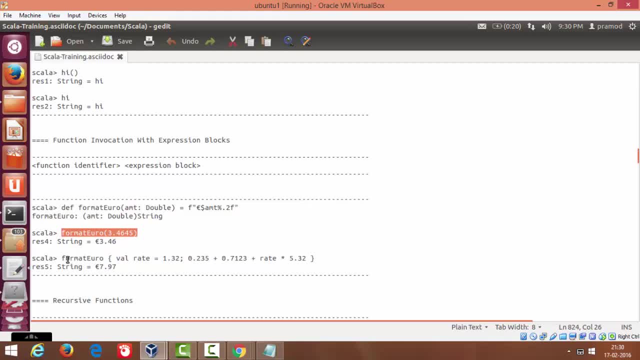 This is the normal way of calling a function, But we can also Pass expression block. It will be evaluated first And whatever is the last expression- Evaluated value of the last expression- that will be Passed as a parameter to the function. 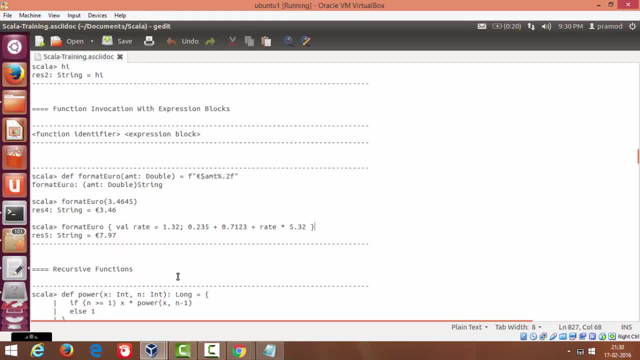 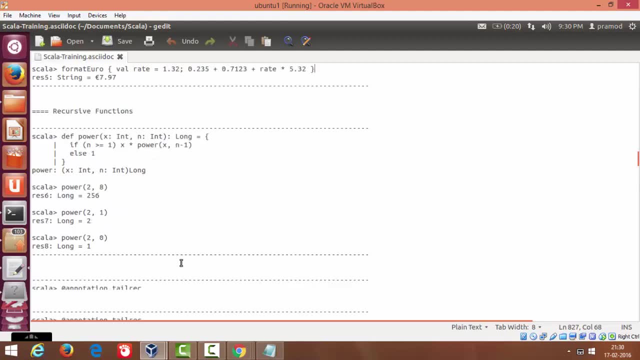 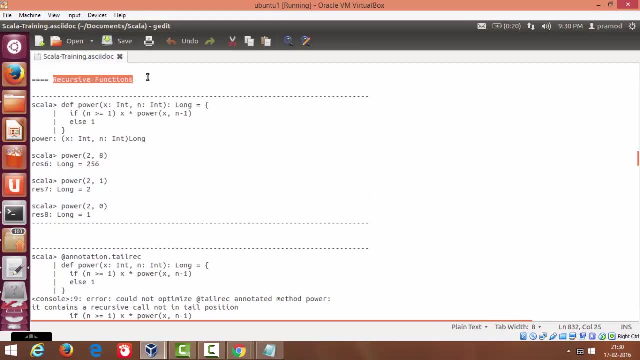 So these syntaxes you will find in the Most of the Scala programs. I think we had Covered recursive programs and all right, Anyway. Yeah, recursive functions Are the normal recursive functions where stacks, Frames, are built upon with every call to the function. 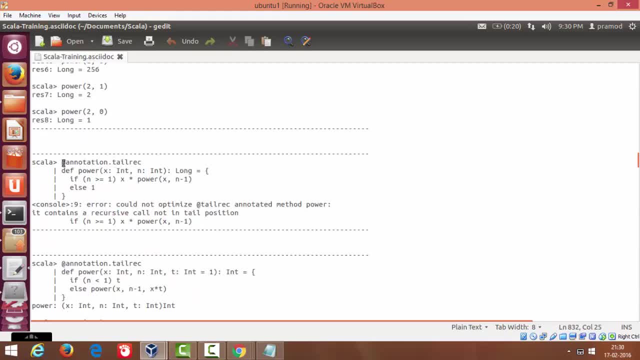 And we saw that By adding tail recursion we can get rid of that Stack frames and Only a single stack frame will be available, Will be used, reused again and again, Provided The last expression in the function is a Call to the same function. 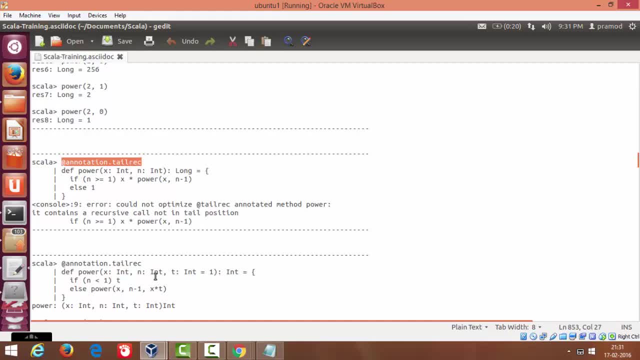 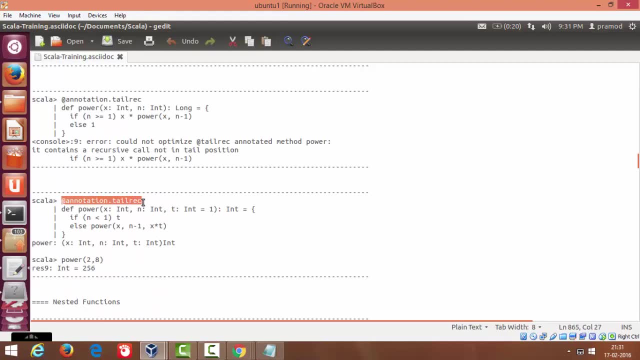 And the tail recursion Annotation Says that It tries to optimize the function. It tries to optimize the recursive function So that it uses only Only a single stack frame. More than one stack frame will not be used. A single stack frame will be. 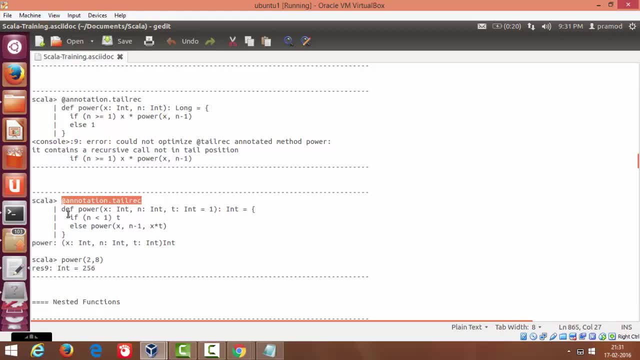 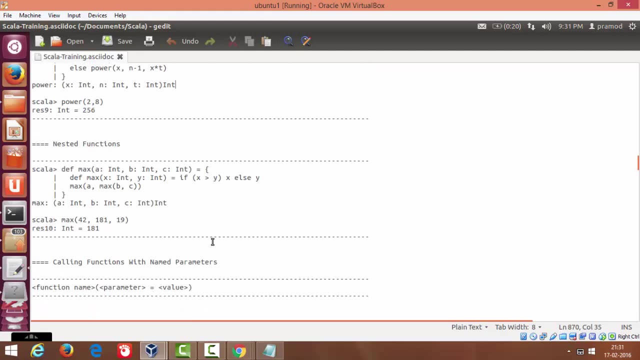 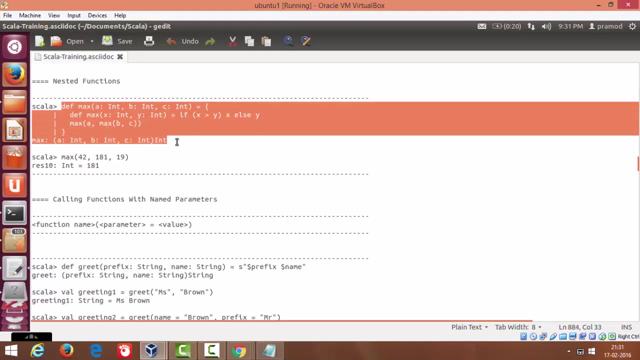 Reused again and again for the Recursive call, provided the last statement In the function, a last expression in the function, Should be called to the same function. I think we did cover all these things. Then we have Nested functions, Which is nothing but function inside a function. 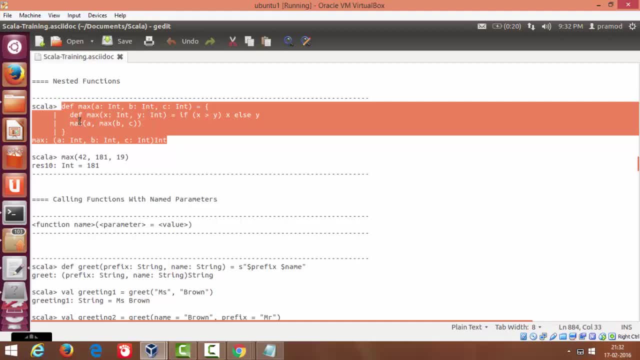 Mostly we will see like java scripts Being written in this Fashion. So here We are defining a function Inside this function. After the definition of that function, We are calling that function. So this is like a private function inside the. 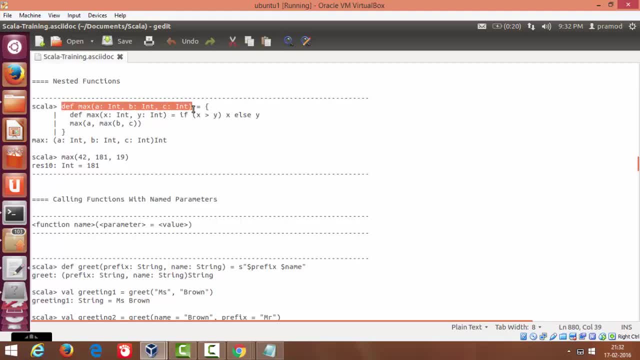 First top level function. So The Nested function Will not be Available to any. It will not be visible to any other function outside the Higher top level function. So these Nested functions are usually Used for Code reusability and private kind of a function. 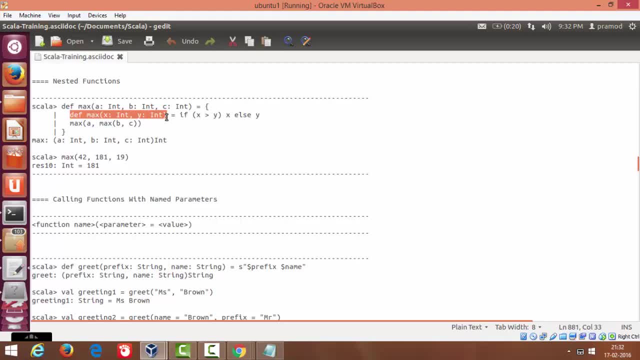 To restrict the scope of the function So that it is not visible Outside the Top level function, And also, and mainly, because You can use Reuse the function. So here, What we are doing is: This is a simple max. 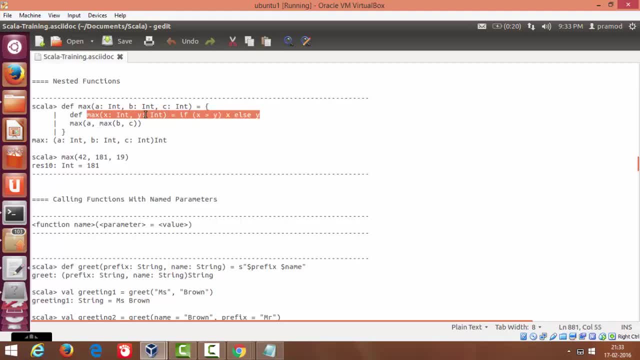 Function definition Right Max of x comma y. It will Give us Whether x is greater than y Than x Or Else y. So it Just gives us the maximum of two values. Now suppose we want maximum Of three values. 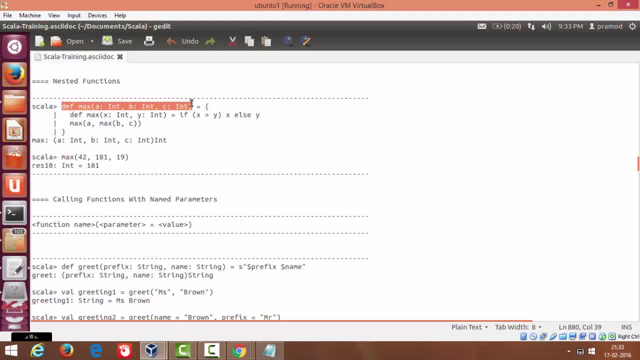 Instead of Rewriting The function With if else, If else Conditions, We can Reuse the Already Return function. So that's What makes Nested function A bit of. It is Mainly used for: 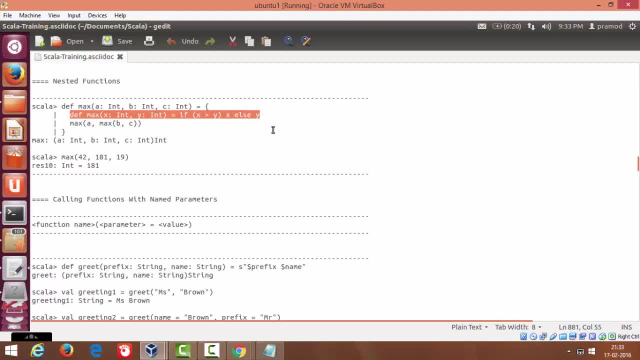 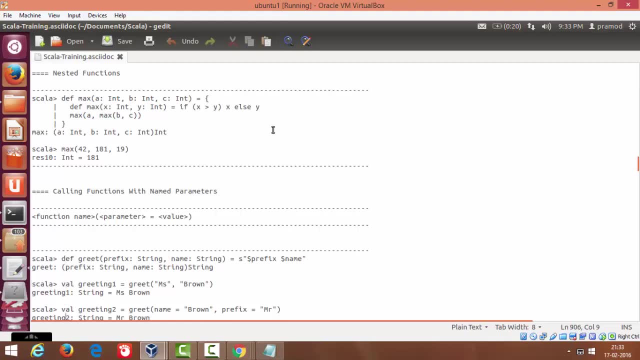 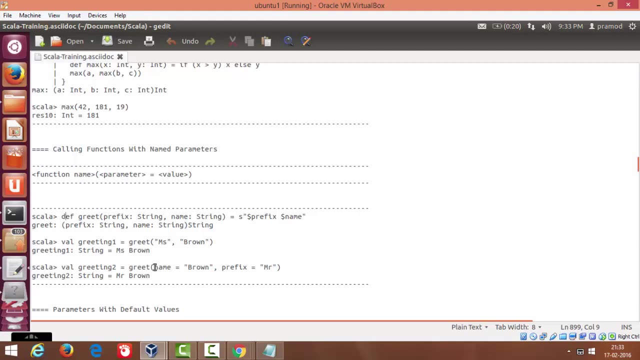 Reusability. I think. Next we had Calling functions With named parameters. These are all Similar to any other Programming Languages. We specify The name Of the Parameter And pass The value We specify. 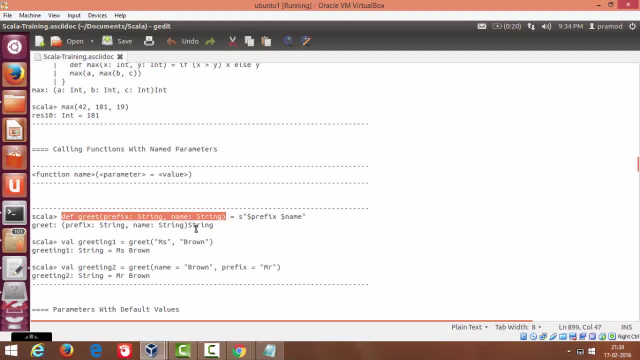 The name Of the parameter, Because in the definition, If you see, We have Two parameters: One is Prefix, One is Name. So we are Calling That function With the By specifying Name Of the parameter. 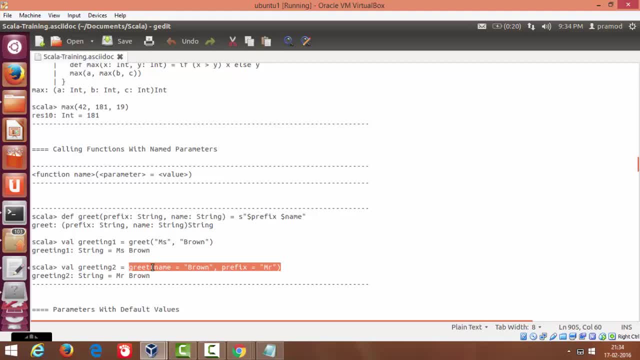 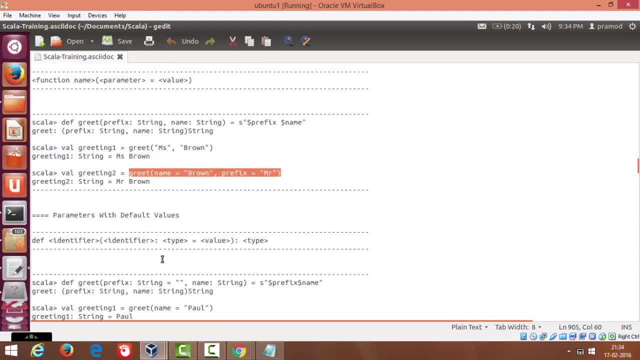 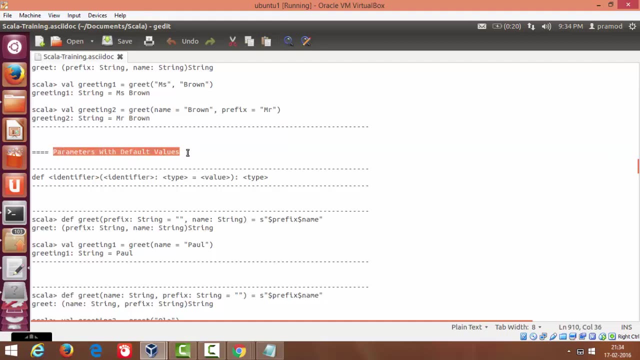 And passing The value To the Name. So Now We can. If we Have The name Of a Parameter, We can Write It In Any Order. That's What makes Named. 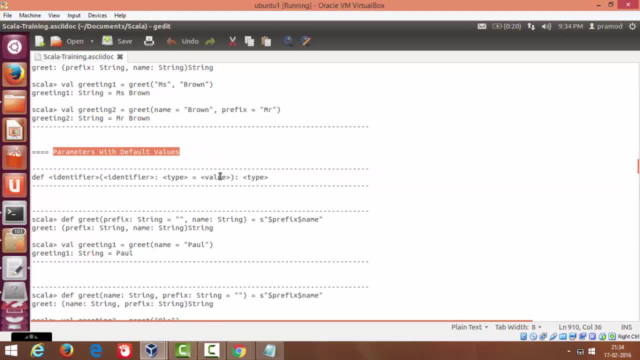 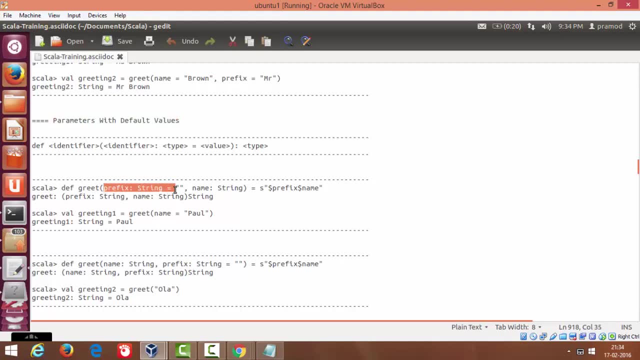 Parameter Very Useful. This Is Next. We have Parameters With Default function will be called. If you see, here is a function greet with parameter prefix of the type string and default value is null string and name is string. So suppose we are. 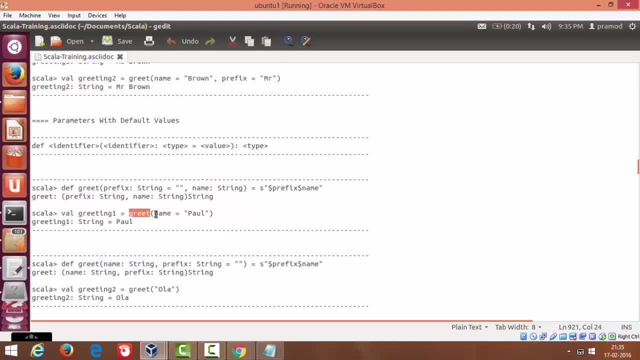 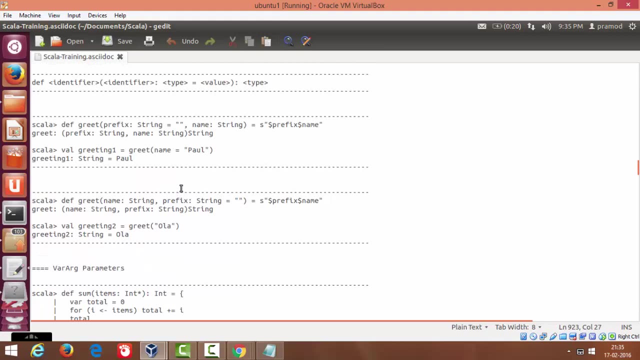 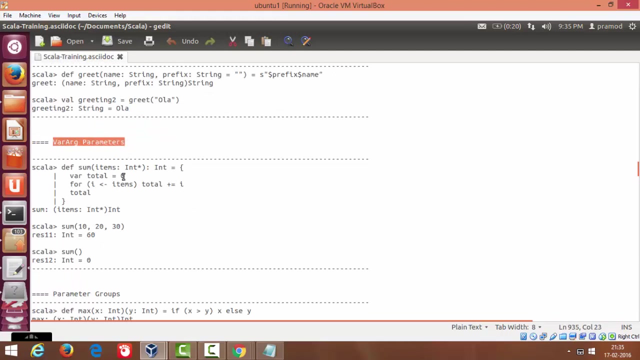 calling here the greet function and we are not passing the first parameter. So by default it will take null string as the prefix. So these are like any other function in different programming languages. Next, we have variable argument parameters. again, variable argument parameters is to pass. 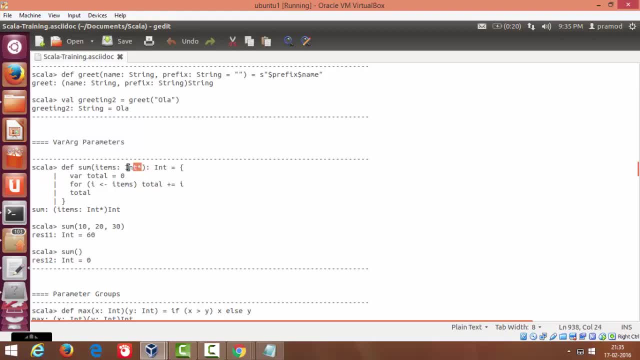 variable number of arguments to a function. So we need to just add a star to the data type, So it will take variable number of arguments. arguments, if you see some, is this is the way it is called. you can call it with any number of parameters. here we are calling with three parameters, but you 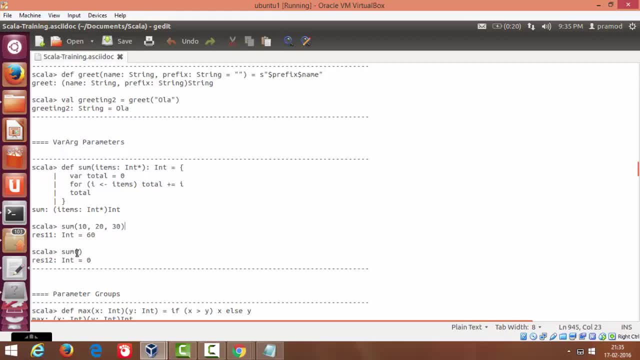 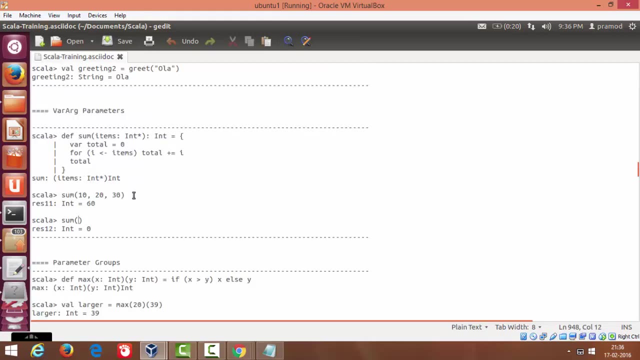 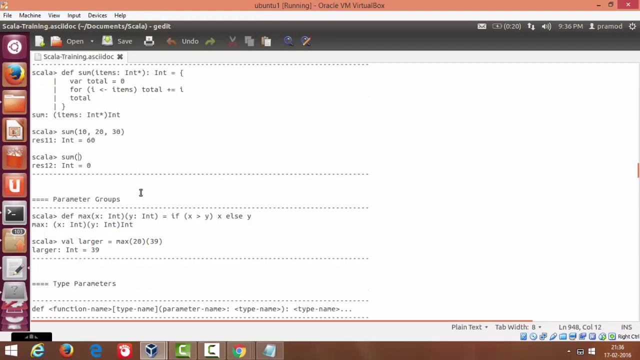 could also call it with with any number of parameters. here we are calling it with with no parameters, so it's just like how we pass arguments to our main function. so that's what? functional? these are the different varieties of functions: how, how and all you can define a function, then we have kuring. this is you. 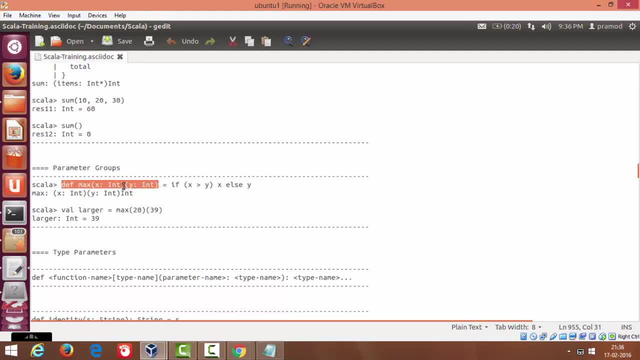 can tell. you might have seen a single parameter group, a single parameter list. we can also specify multiple parameter list, so these will see later what is the use of this. it is again like you may specify while calling the function, you can parameter list and we can give it later. you can pass that missed parameters later somewhere. 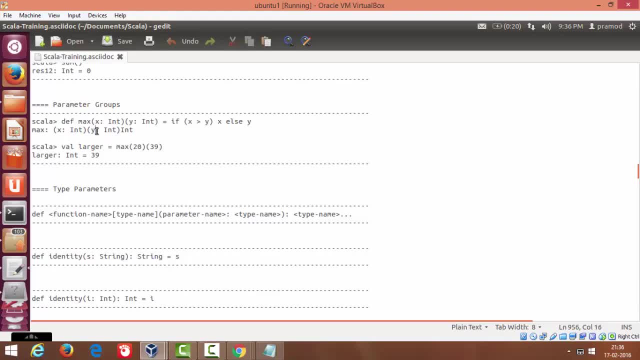 else. so we will see. just remember that this is also a syntax of Scala. we will see more examples of these kinds. why it is used. what is the use of multiple parameters? but just to remember, this is also a valid syntax in Scala, passing multiple parameter list again. 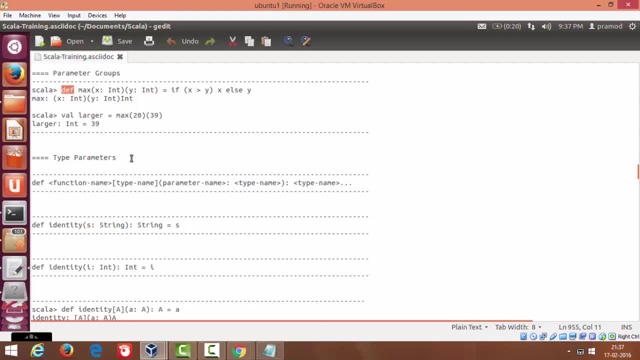 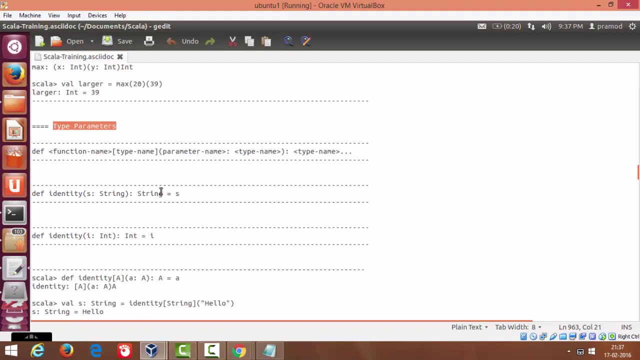 it will be used for reusability of the code. just remember that it will be used for reusability of the code. Next, we have type parameters with respect to functions. Generic parameters with respect to functions is nothing but which will be used for generic. 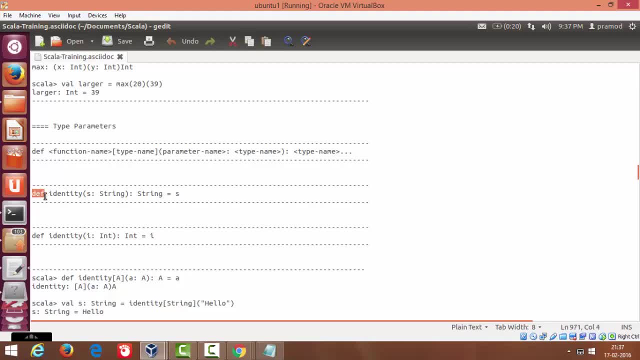 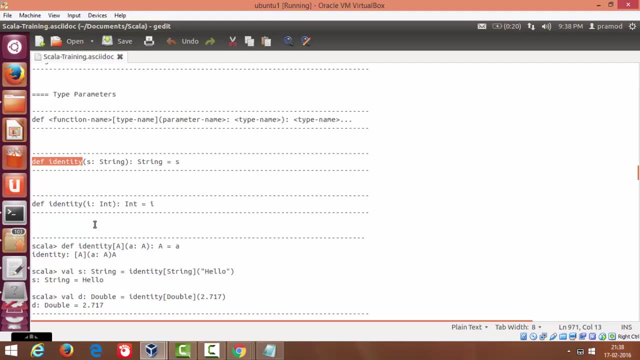 types. Suppose you have a function and you want to pass any data type, It should handle integer data type or double data type or any other data type, just like generics in java. So the way we specify is data type as A, It means any data type, or this A is just a it. 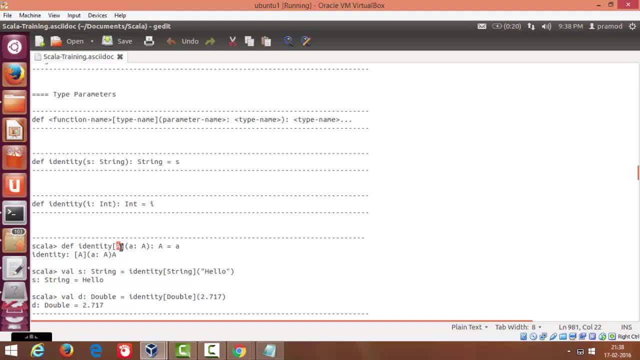 could be any character capital letter. it is a convention, just a convention of specifying a character, bigger character, capital letter, character. You could also say that it could be B, And here it will be B. It means this function: you can pass any data type And capital letters are the way of specifying this type. parameters for functions. 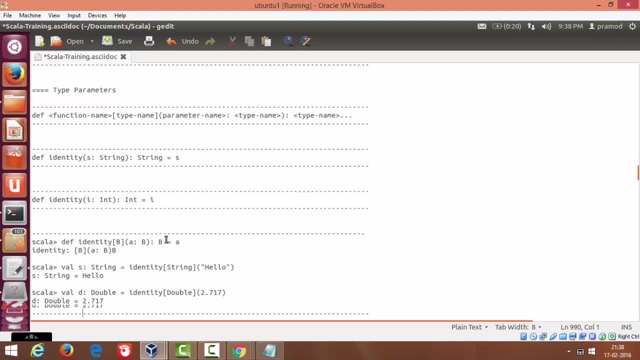 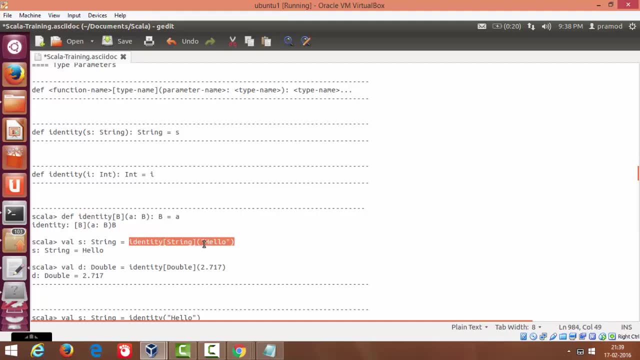 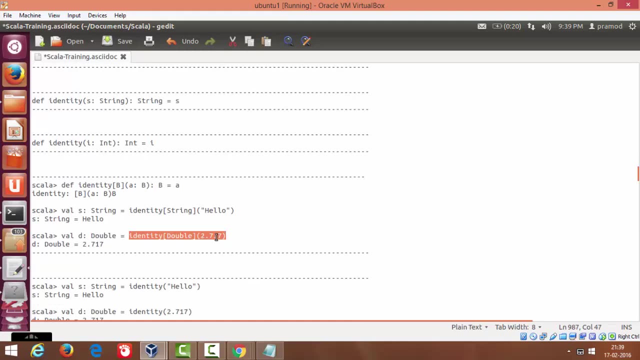 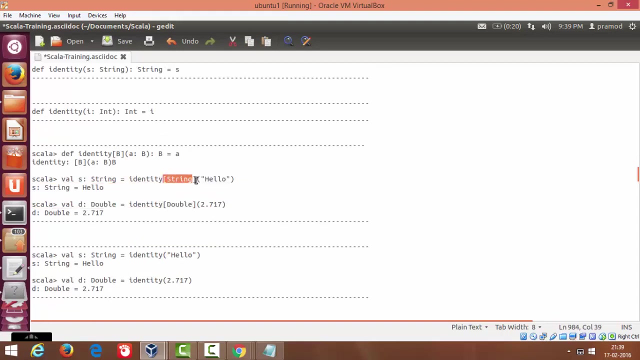 It means, if you see here now, this function could be called with any data type. First we are calling with string data type. Next we are calling with double data type. Also, this data type specifying while calling is again redundant. We can get rid of these things. 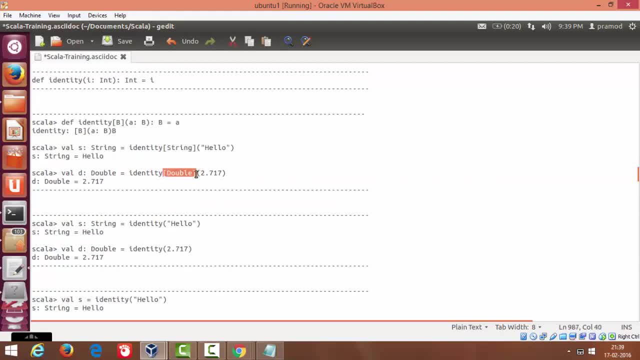 Scala compiler will come to this, Come to know, will infer it for you, So you can directly specify identity as call identity with string and call identity with double. So this syntax means it's a generic function. Mostly when you write libraries or expose your own APIs to others, you want it to be generic. 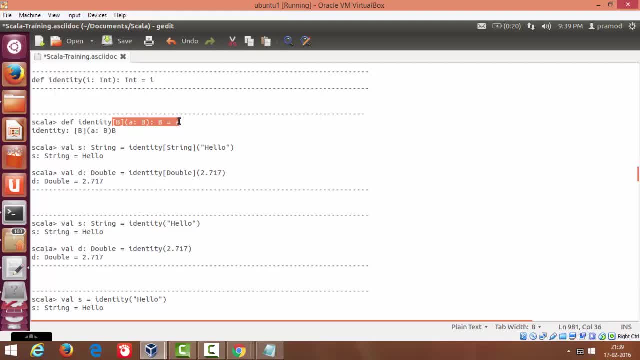 That's where you will be writing a generic API that can, That can take input any data type as the input here. In our case, we are calling it with string and double. We can also call it by integer or any character or an object. 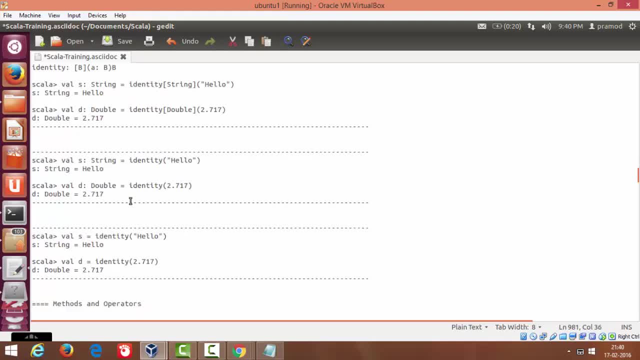 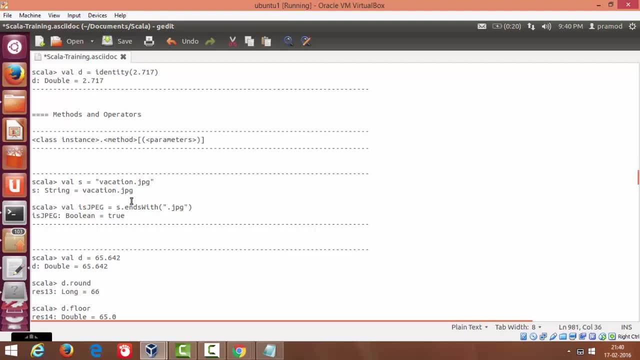 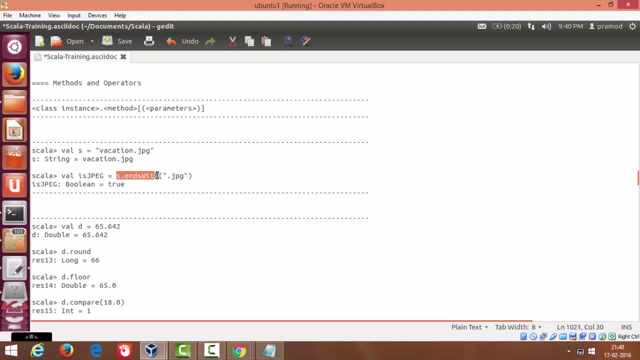 Anything, Yeah, methods and operators are Here. We have an object And we have methods for that. Here in Scala, there is no, nothing like operator. Everything is a method. We don't have plus operators, We don't have minus operator, or we don't have multiplication division operators. 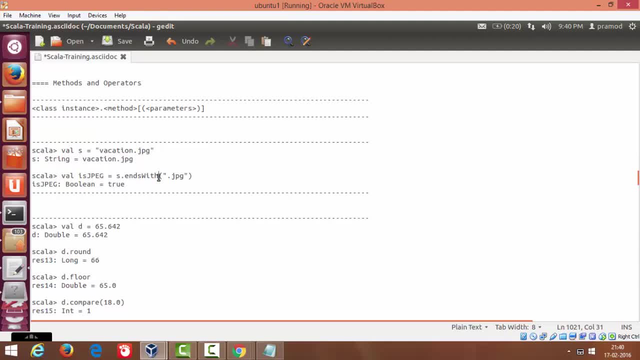 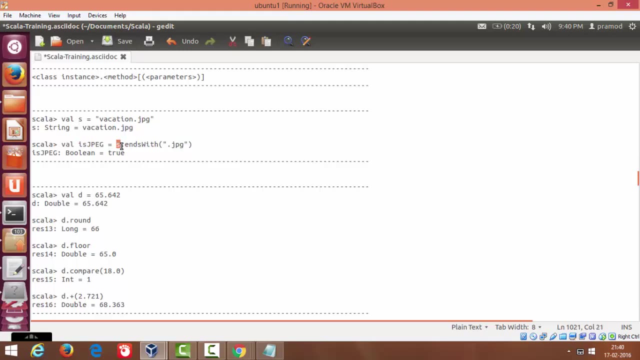 All those symbols are functions On the object, Integer object or double object. So this is nothing but an object And we are calling the method of that object, Just as normal in any Java programming. We have an object and we call method of that object. 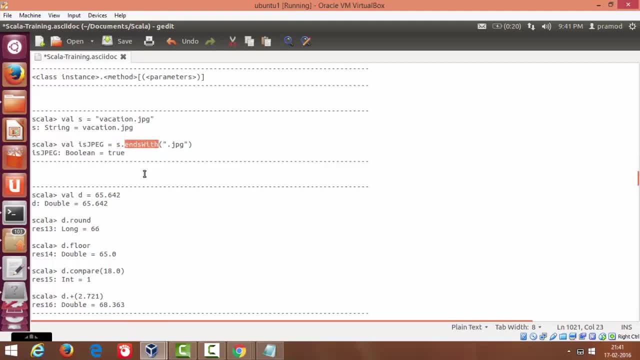 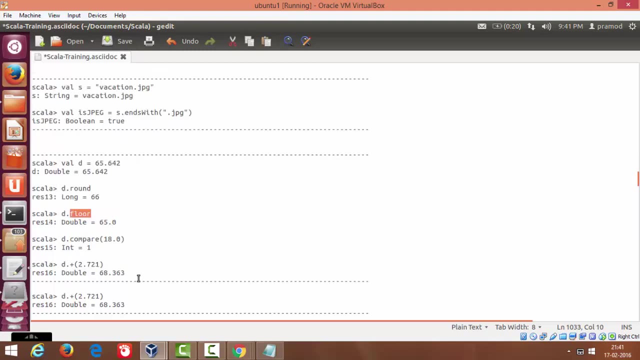 Here the string. A string has a method with ends with method. String is an object and it has an ends with method. Similarly, we have Double dot, round. Round is a method of this object. Floor- again the method of this object. 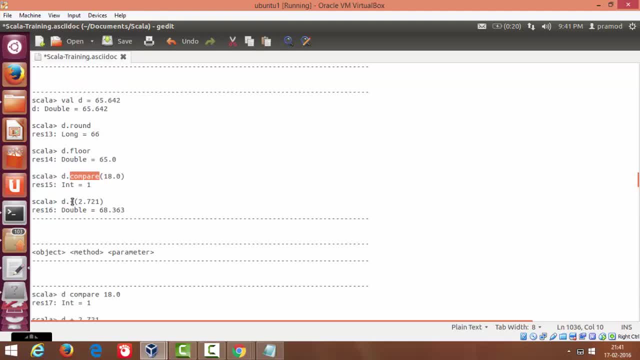 Compare again: method of this object. If you see, this is As I said. plus is not an operator in Scala, It is a function And this is how we call a function. We have this object. Then, using the dot reference, We call the plus method. 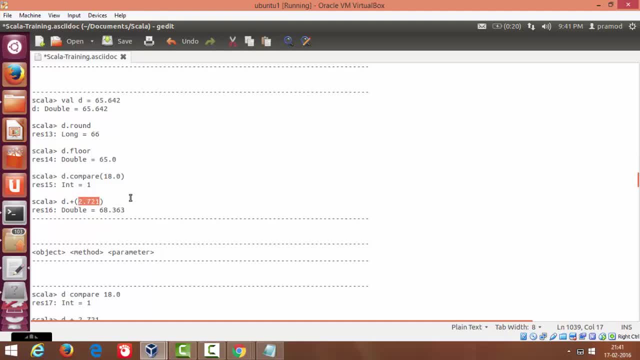 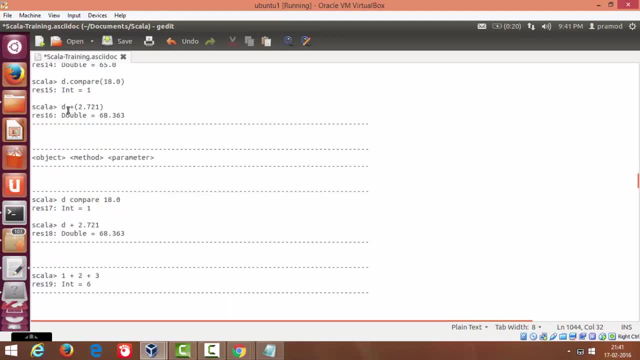 And pass an argument to that function. You can either use the dot parameter Or just give a space and call this way. This is also valid syntax. We have object Space Method of that object And then pass the argument to that object. 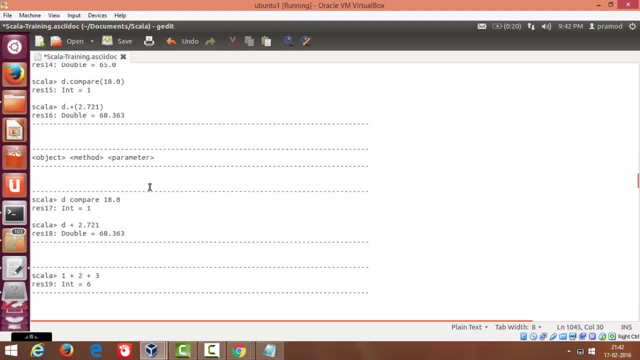 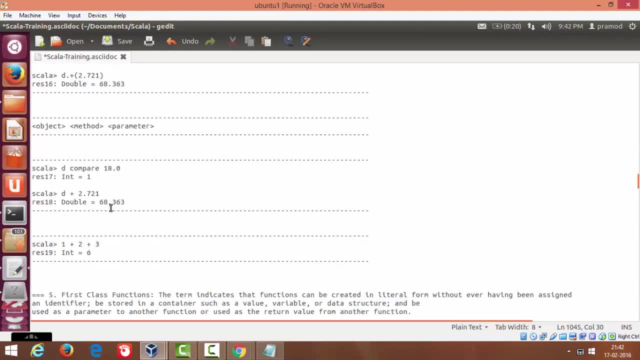 So this is mainly used when we do Arithmetic kind of operations on the Strings, doubles or integers. This is all. This is a Valid, Valid syntax because we have object Space Method on that object And this is the parameter that is being passed to that. 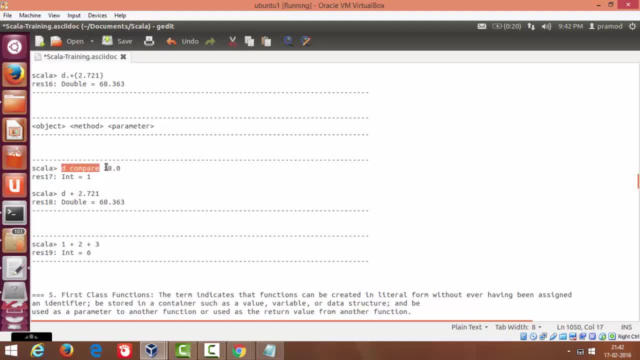 Method. So. but it is recommended not to write in this fashion, So it is confusing a bit. It is always recommended to use arithmetic kind of operations, To use such kind of a syntax Like A plus B, C plus D, A minus B. 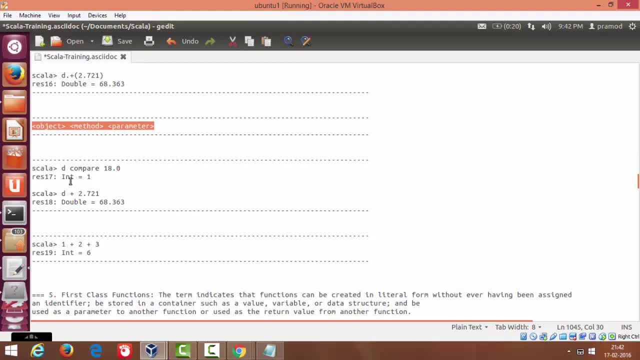 A divided by D. So all those are Specified in this format. So always Specify the arithmetic operations in that, In this format, And Other than that, Try to specify using the dot operator method, Dot Method Object. 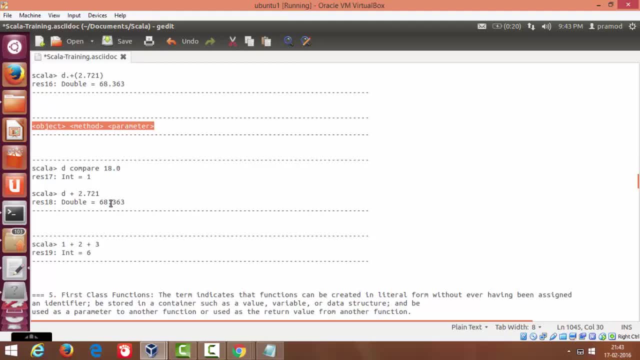 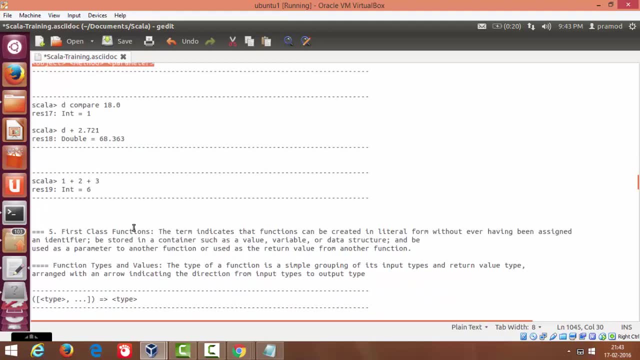 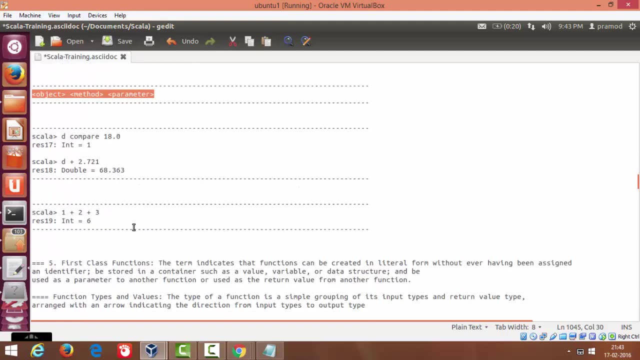 Dot And Method And then pass the argument to those things. Yeah, These are Simple Function Definitions Of Object And Method And Function Definition What all Functions are. So now comes Our 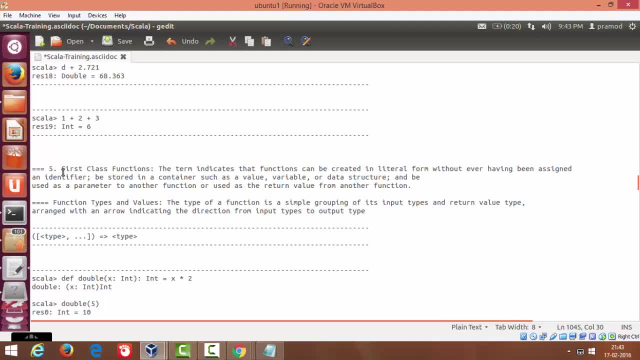 First class functions- Scala. In Scala, Functions are called first class functions. What it means is: The term indicates that functions Can be Created In literal form Without even Having been Assigned An Identifier. You need not specify a name. 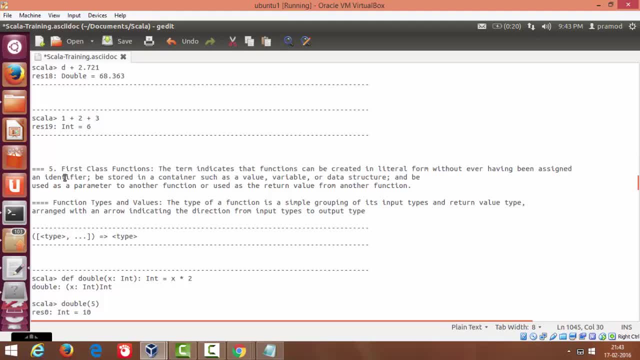 For a function. We can directly write a body For the function. That what? That's what it means: Literal form. Literal form means You need not Give a name To a function. You can directly Write a body. 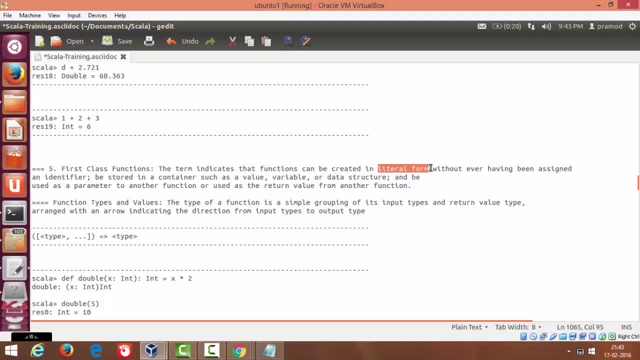 To a function Can be stored In a container, Such as Value Variable Or Any other data structure, Because Functions are Implemented As Classes And functions are Objects. That's the reason We can do. 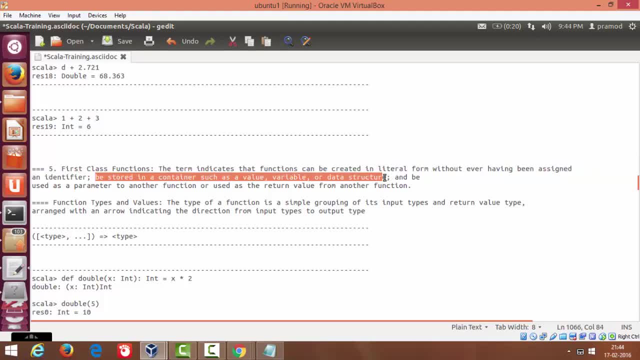 All these Things Can Assigned To some Variable Or Value Or Any other data structures And To be Used As a parameter To another Function. You can Pass a function To a function. 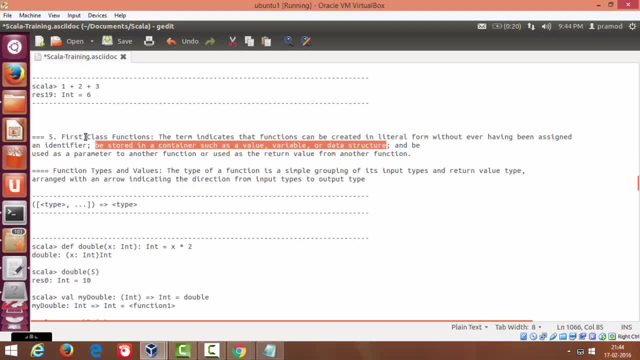 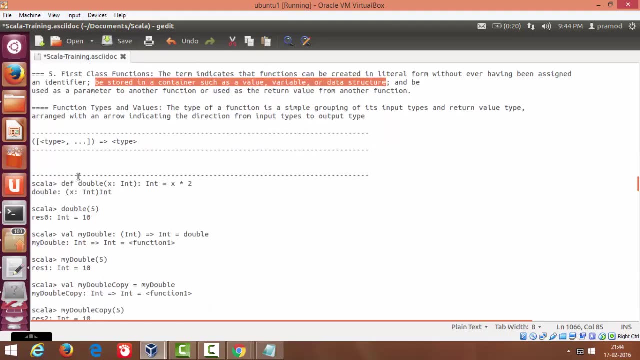 Or Return a function From a Function. That's the reason It is called First class Functions And The reason Behind It is Functions Are Objects, So Let's See Here It's. 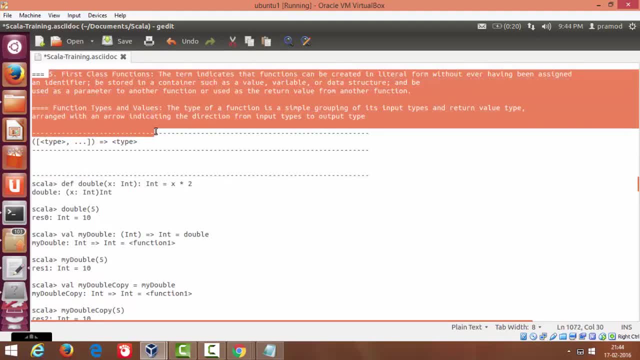 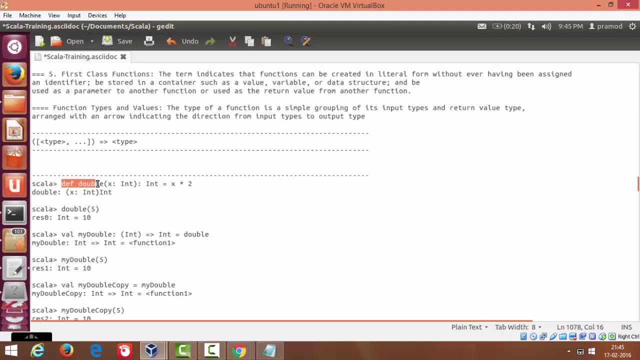 A Bit More Important, Because Most Of The Spark Or Scala Languages Are Based On These. Things Are Return As Higher And Will Result The Double. 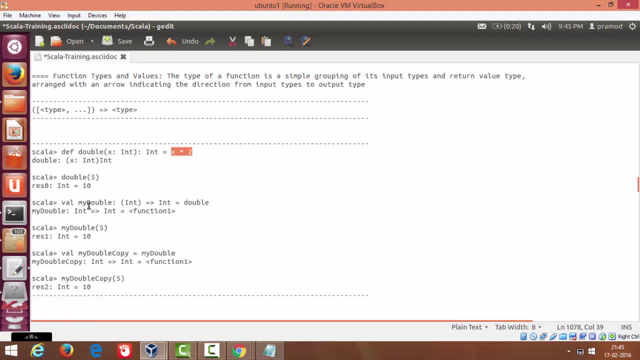 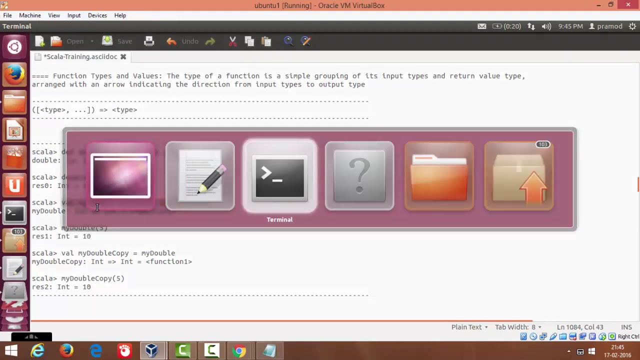 Of That Integer Double, In The Sense It Will Multiply By Two And Give The Result. So If You See, Here We Have Double, We Saw. 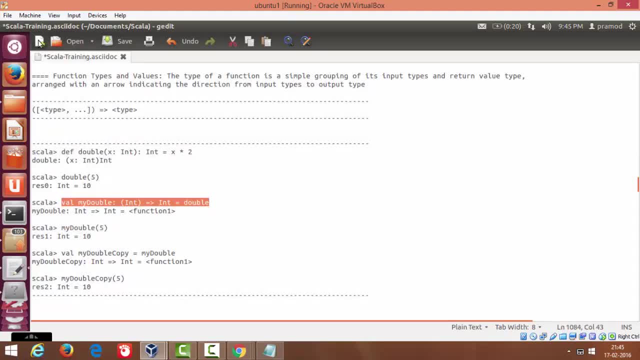 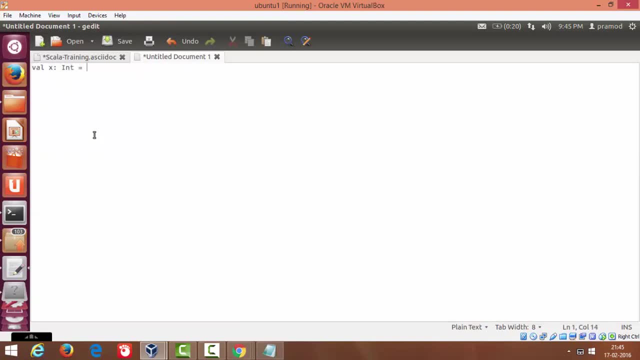 That Val X, Then In Equal To Then. Now What We Have Here Is Val My Double, Then We Have Colon, Then We Have This Double. 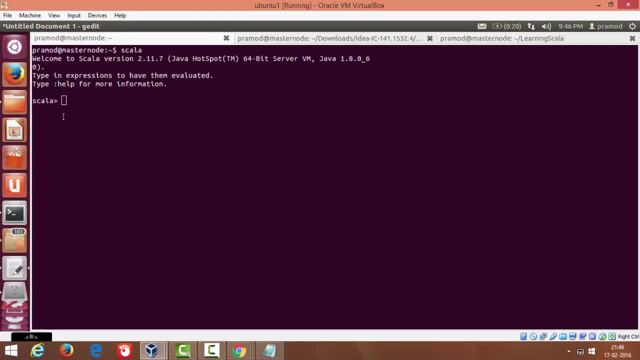 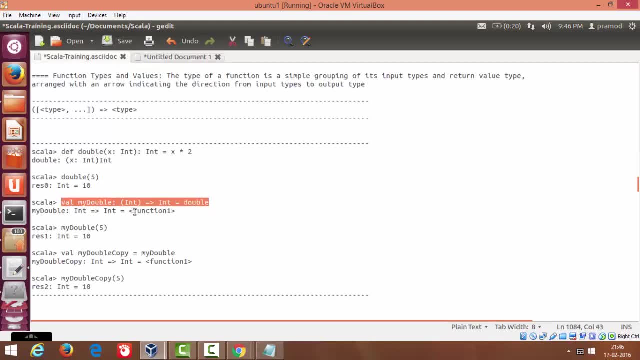 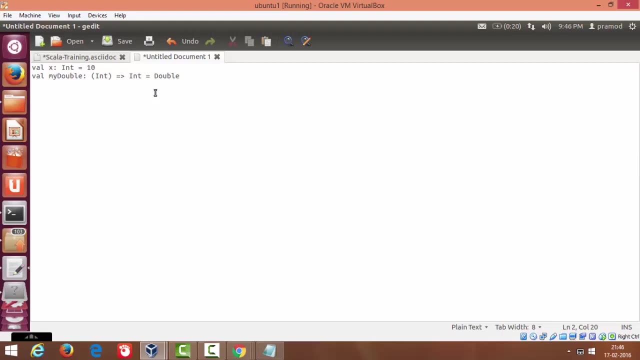 This Is What We Are Having Here. That's What This Shows. Okay, Let's, Let's Put The Open Bracket And Close Bracket Also, But It's. 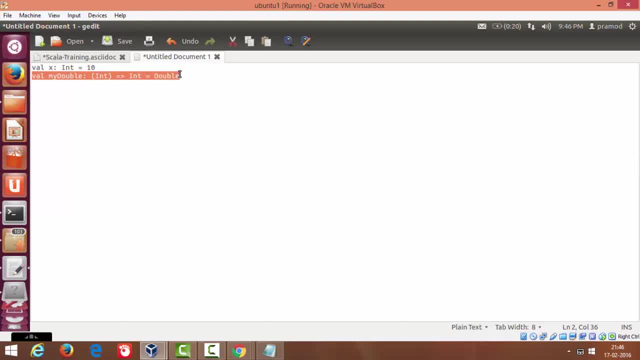 Not Mandatory For Single Parameter. What Does? X Is A Identifier, And Then We Have Colon, Then We Have The Data Type Of The Identifier And 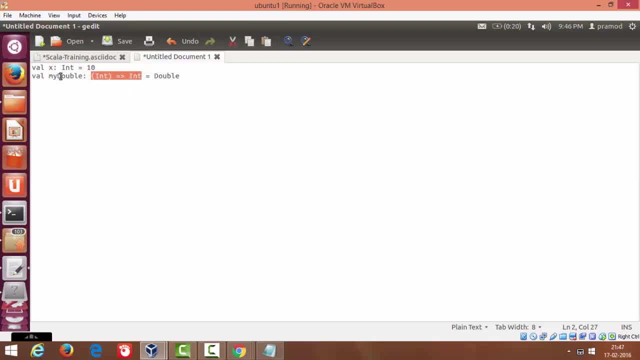 Then We Are Assigning A Value Here. Similarly, My Double Is A Function Variable. It Takes Int As A Input Parameter, Input Parameter And Its. 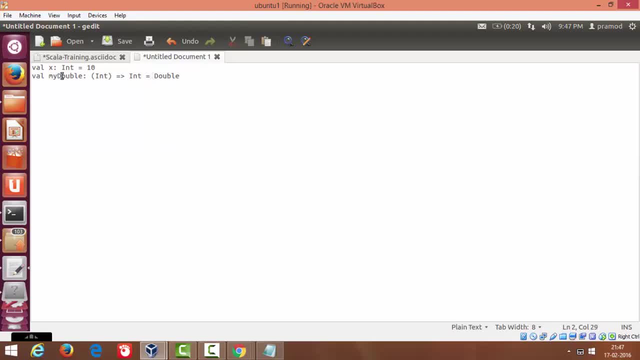 Return Value Is Again Int And Then We Are Assigning To That Identifier Or Function. Just Visualize In The Same Way That My Double Is: 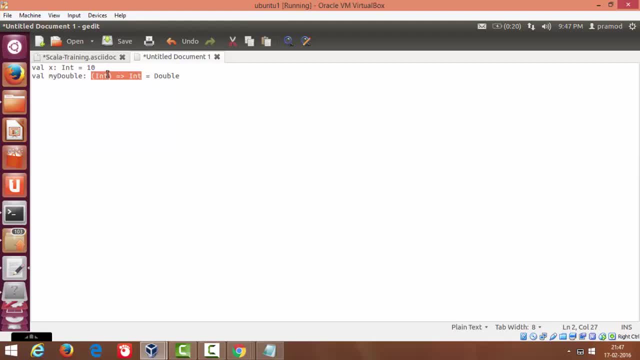 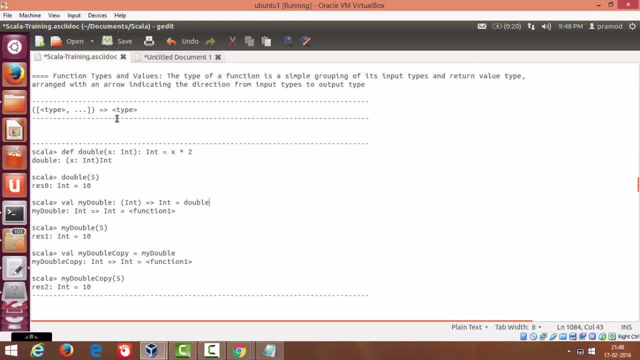 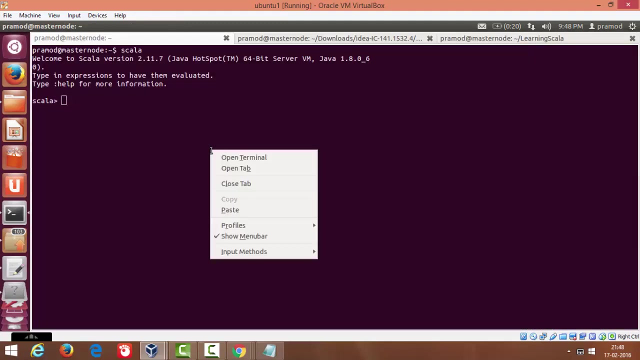 Kind Of A Pointer To This Function And The Data Type Of This Function Variable Is. It Takes Int This: This Is A Simple Function, Def. 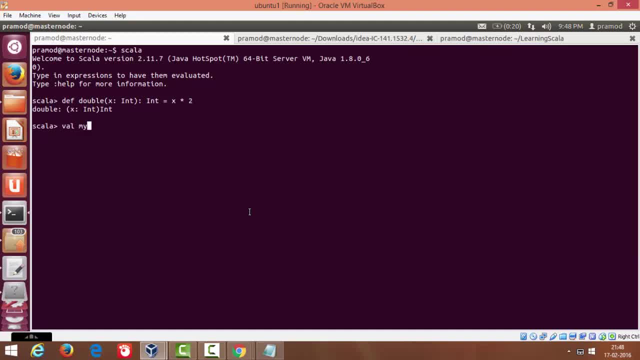 Double, Which We Find. My Double Is A Function Variable And That It's Data Type Is, It Stakes Int And It's Return Value Is. 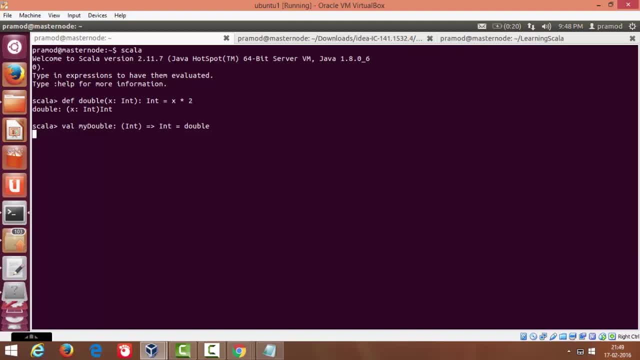 This And We Are Assigning Double Function. This Is Just Like A Pointer To Function Now. Now We Can Use My Double And Pass Actually. 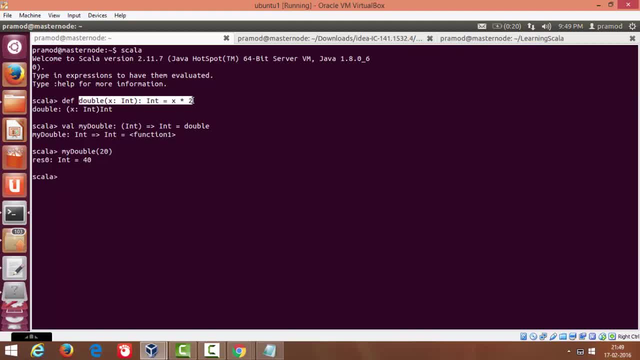 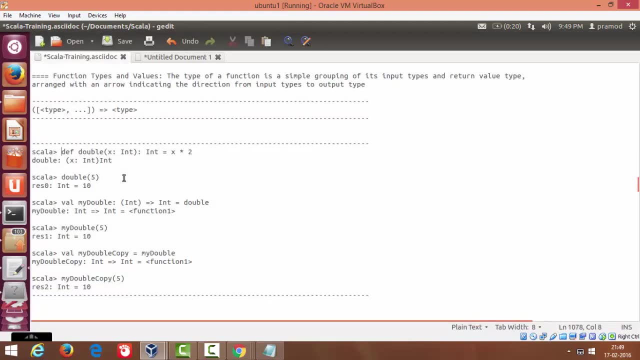 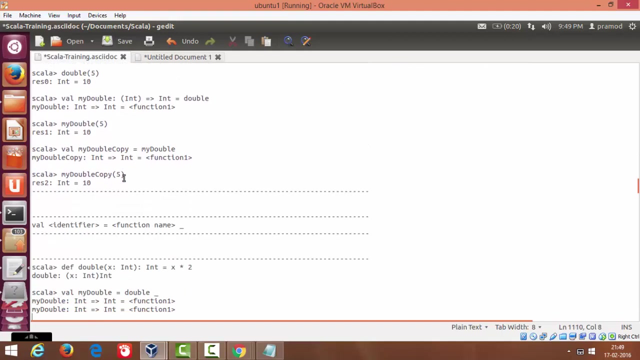 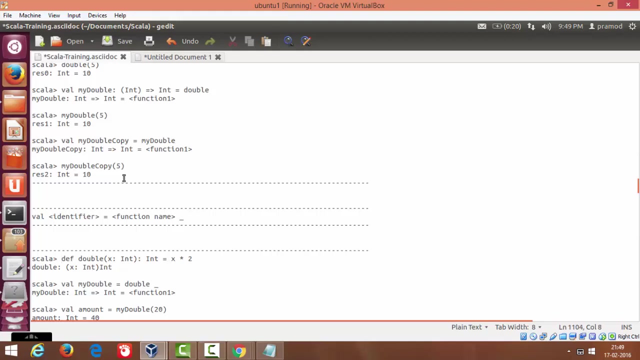 The Value. So Actually This Function Will Be Called. That's What Makes First Class Citizen Scala. Any Any Doubts Here? Shall I Continue? Yeah, We. 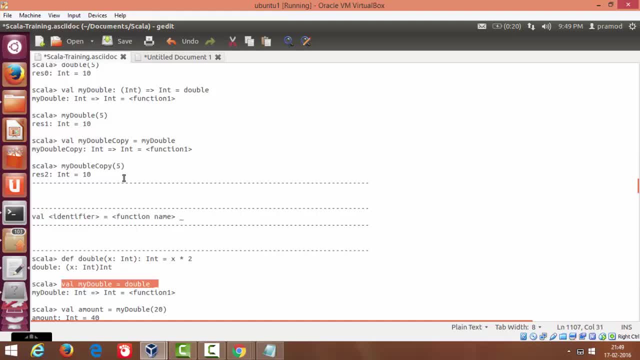 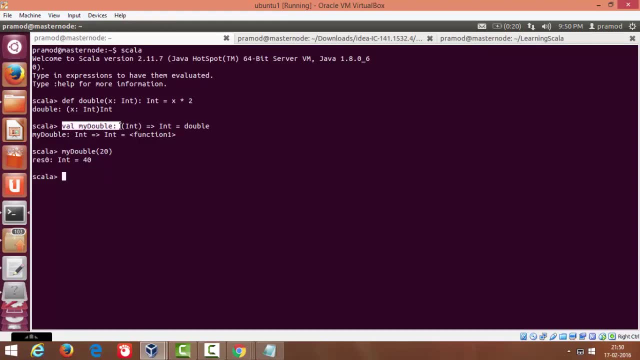 Can Also Specify A Placeholder Like This. So We Have Defining A Function Variable. We Give The Identifier Name And We Specify The Data Type. 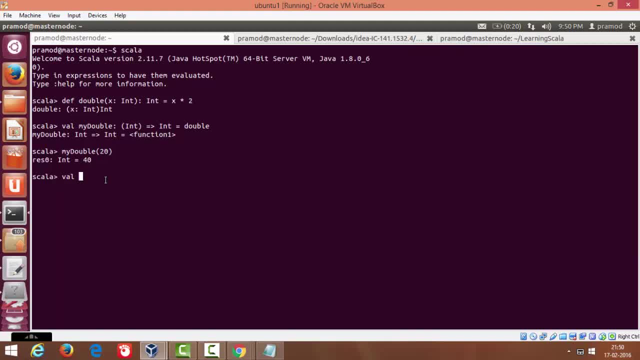 In This Way, Whenever You Specify The Data Type In This Way, If You Specify Double Of, If You Specify Underscore, Okay, And We Are. 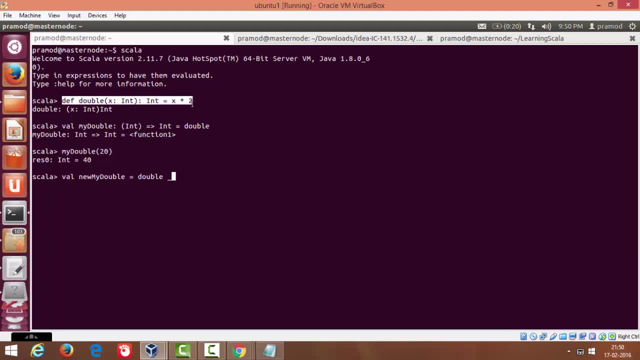 Not Passing The Parameter. To See, Actually, We Are Calling This Function, Here We Are, And, But We Are Not Passing The Parameter. We Are Just 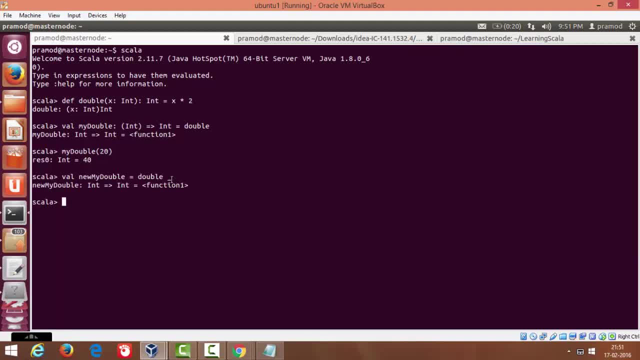 Placing An Underscore Here. When We Do This, It Will Create A Function Variable By Placing An Underscore Variable. This Is All This. 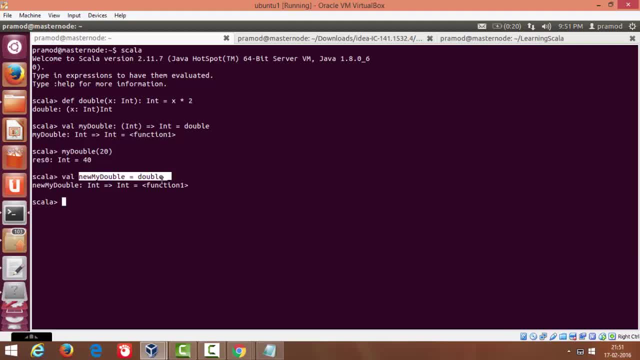 Will Also Create A Function, Variable Again. This Is Again Used For Reusability. We Will See More Examples On What. What's The Use Case? 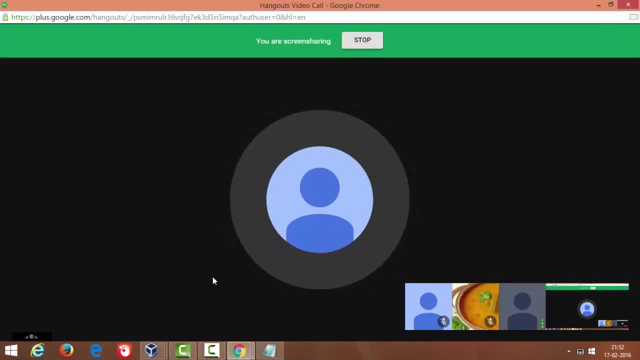 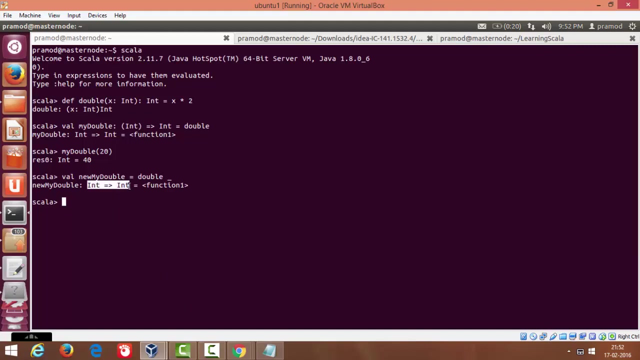 I Didn't Get The Question. It's Showing In Where This One Is. This: Are You Asking About This? That My New, My Double, Is A. 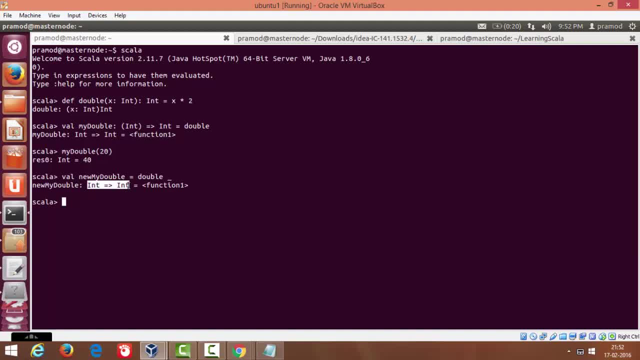 Function Variable Of This Data Type. Yeah, That's Because Whenever You Specify Underscore And Don't Pass The Here Double Is A Parameter Here Instead. 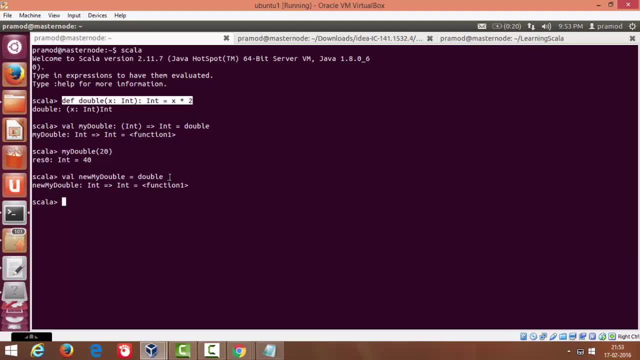 We Are Placing An Underscore. It Means That We Can Pass The Parameter After Some Time Or In Any Other Place. This, This Syntax. 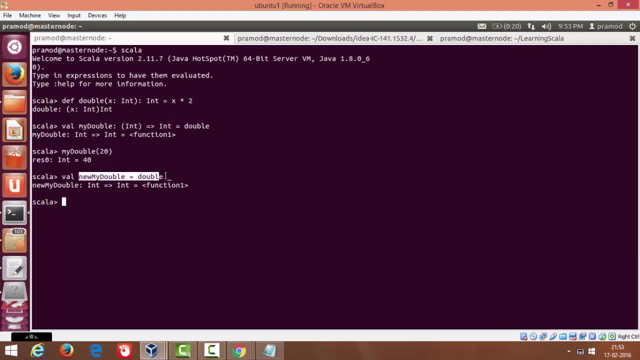 Will Again. This Is One More Way Of Defining A Function Variable By Not Passing The Actual Argument. This Will This. We Can Pass The. 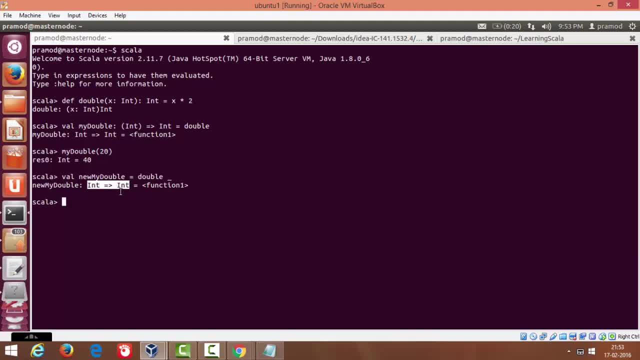 Argument Will Be Passed Later, Probably As The Return Value This Means, This Data Type Means. This Is A Function Variable, So We Can Now Call. 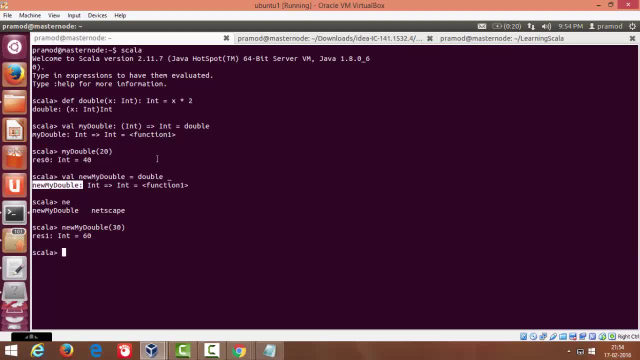 New: My Double To As 30. We Can Pass The Function. This Is Called Partially Applied Function. Partially Applied Function Means You Don't Pass. 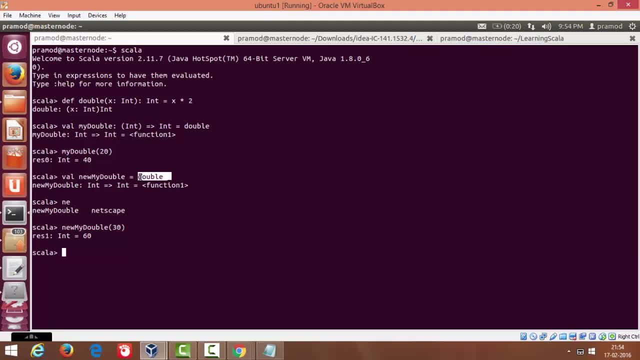 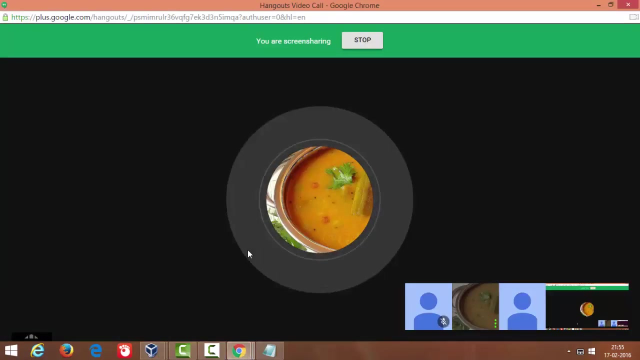 Some Of The Variables Of The Function, Some Of The Parameters Of The Function We Can Pass. This Is That Clear? Yeah, So This Is Val. 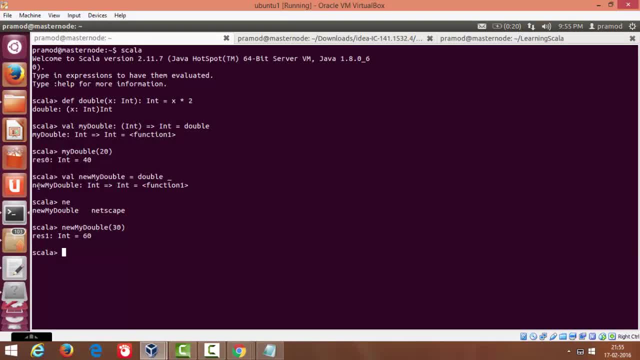 Yeah Right, The Body Of The Function Is A Double, Which It Replace By The Action. Definition Of Function: Right Yeah, That Placeholder Is A Parameter. 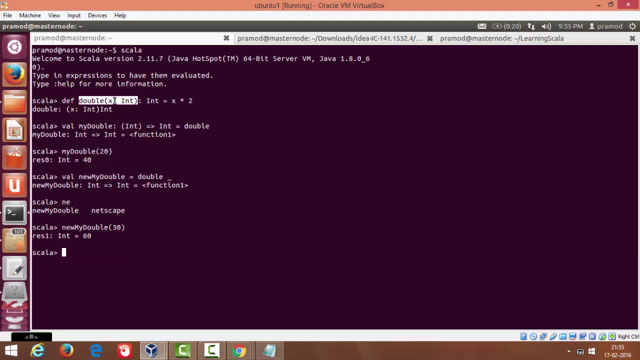 Of This Double, This Function Double Is The Right. It Is Supposed Not Actually Passing The Parameter. Actually, Here This Means We Are Calling The. 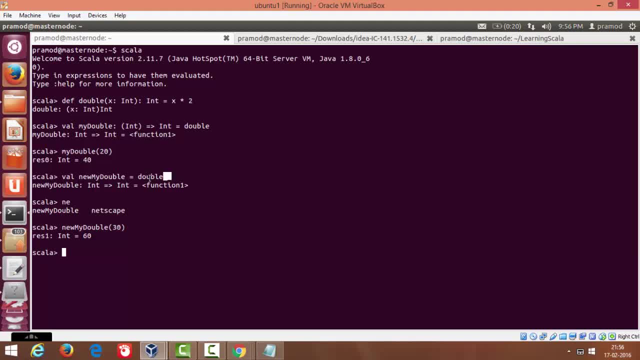 Function. We Are Calling The Function, But We Are Not Passing The Parameter. Whenever, Yeah. Here We Are Specifically Saying That This Is A Function Variable. 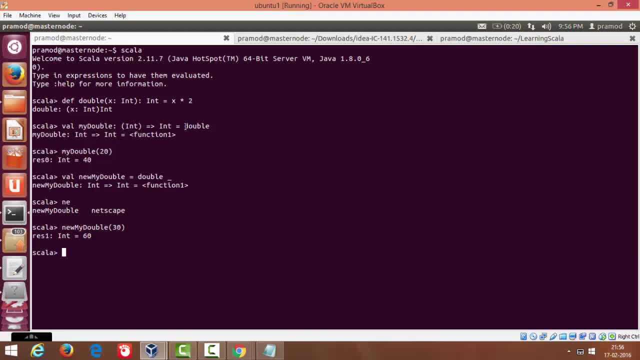 By Specifying The Data Type- Yeah, Type Of The Function, And Here The Function Is Not Being Called. We Are Not Passing The Full Parameter. 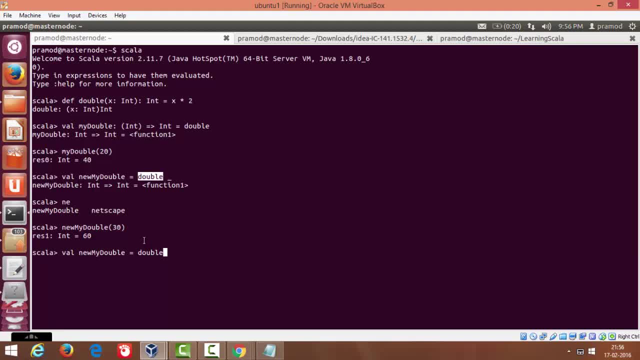 It Will Be. If You See, Val This, Let Me Call This With Proper Parameter. So Here My Double Will Be A Normal Integer Identifier, The 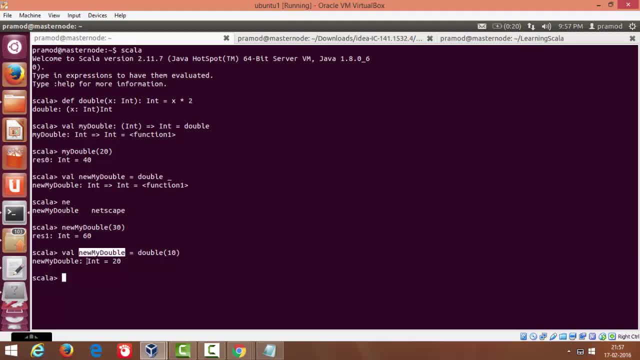 Same Thing. Now We Are Calling, But Without The, Without Passing The Parameter. Now What It Happens? It Will Not Got. It Will Not Get. 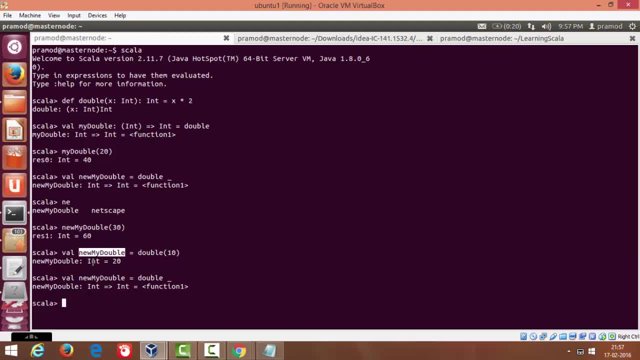 Called Instead Function Value, Function, Function Value. Yeah Yeah, Means It Is This Function. We Are Holding Back The Parameter We Are Trying To Call, But 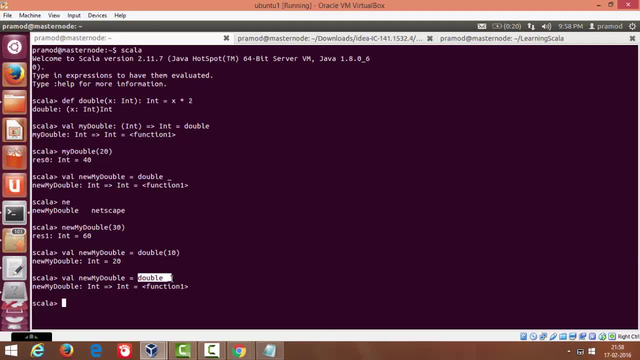 We Are Not Passing The Parameter Function Value Right, Right, Right, Because This Double. Because This Double As The Input And Return Value Is Integer. So 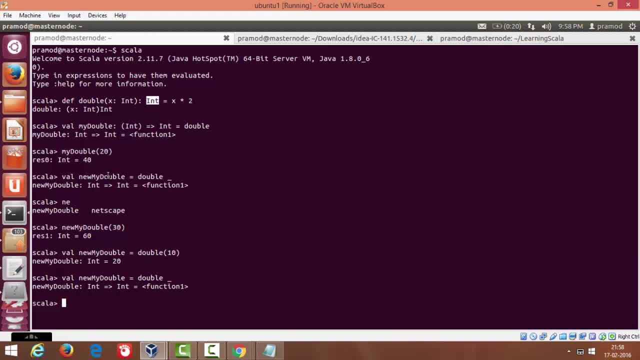 That Got Assigned To My Double. Yeah, Yeah, Yeah, We Can Do That, So We Can Define A Function Like This. Define Function X: We Will. 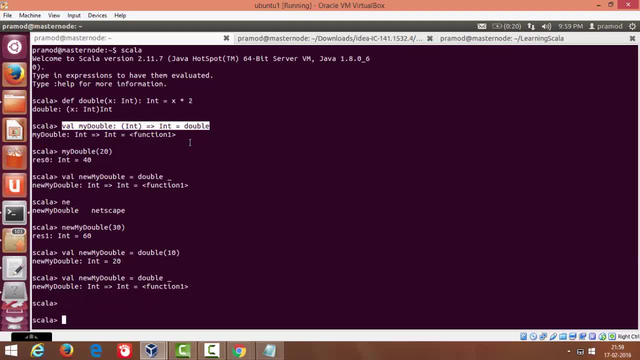 Divide By Two. Okay, Okay, Okay, Okay, My Okay. Data Type Is Double, So We Need To Assign That Particular Function. And Is Equal To: 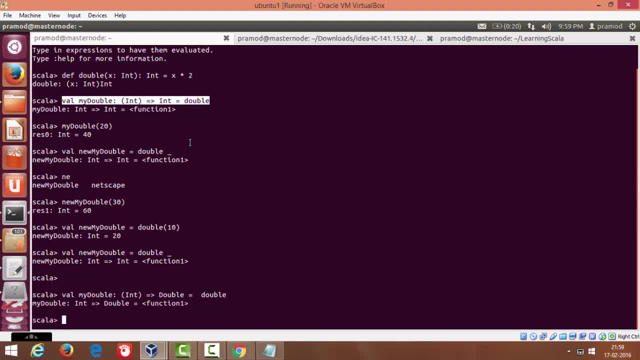 Double. Yeah, It Will. So Then, Basically, What I Understood Is The Return Type Of The Double Right. It Should Be The Return Type Of 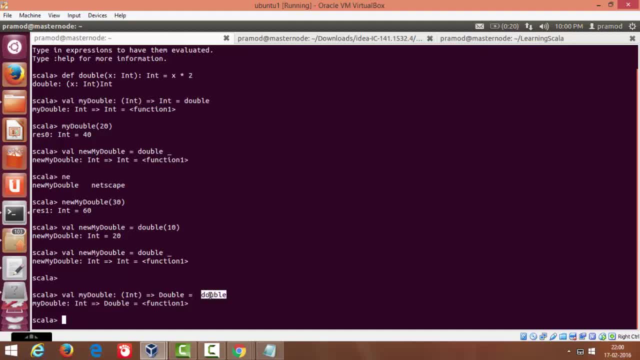 The Double. Yeah, That's True, Because It Has To Be The Return Type Of The Double Function. Once Again, Let's, Let's Make It As: 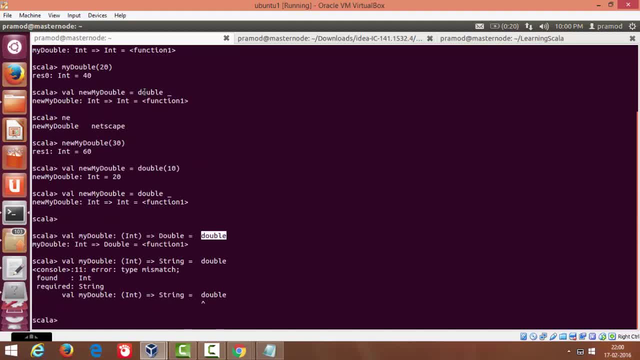 This, Yeah. Now I Think It Is Down Casting, Yeah, Down Casting. That's How It Worked. Otherwise, If You See There Is A Mismatch, 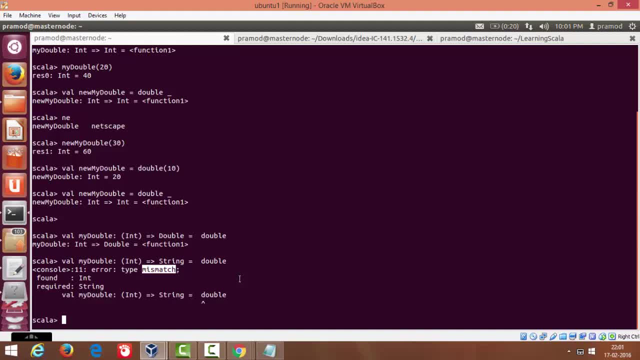 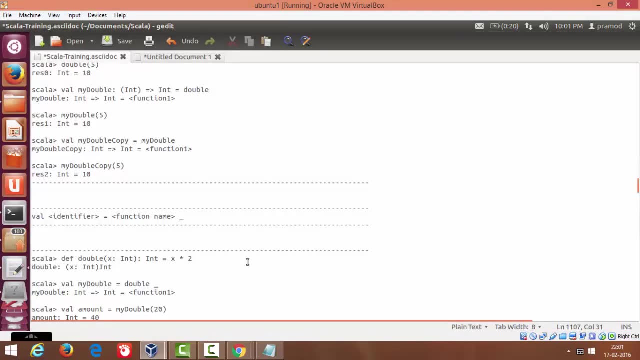 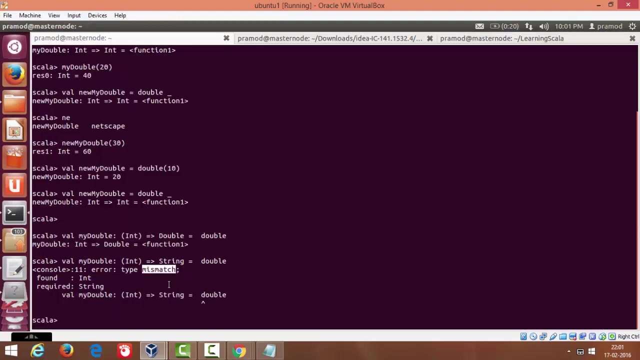 Error. Yeah, Makes Sense. Yeah, Maybe The Up Casting Or Down Casting. Yeah, We'll Be Using More Of This Function. Let's Assume This To Be. 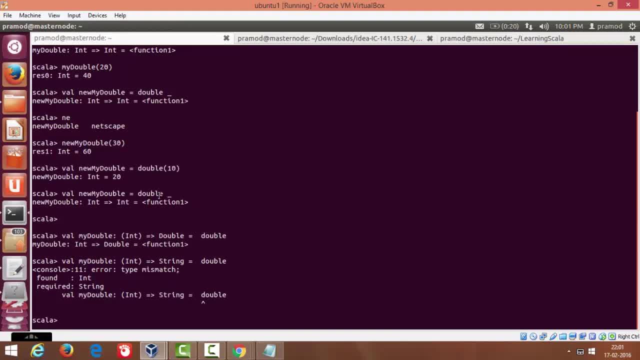 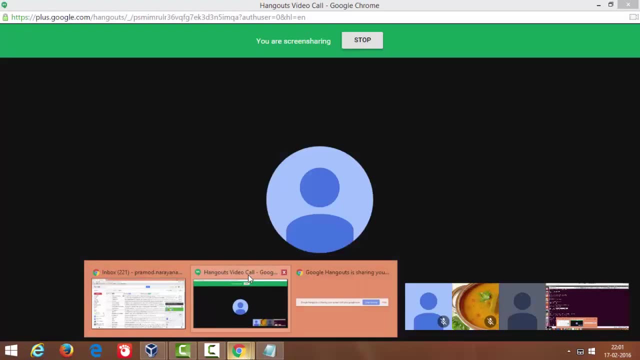 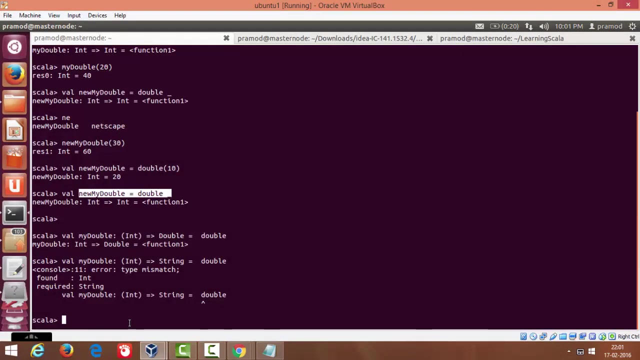 A Like A. We Are Not Passing The Argument As Of Now. We'll Be Passing That. You Have To Mute. Okay, Are You Able To? 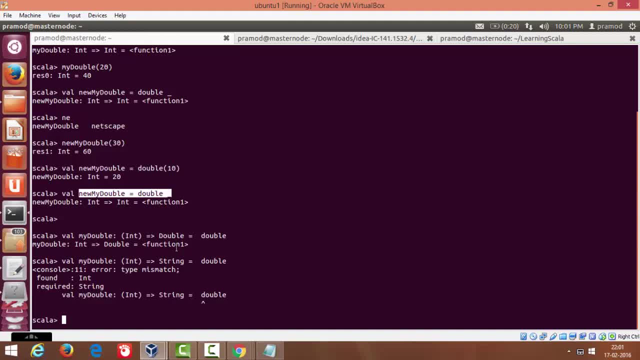 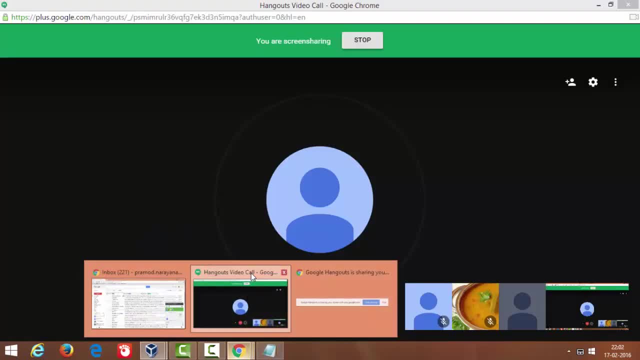 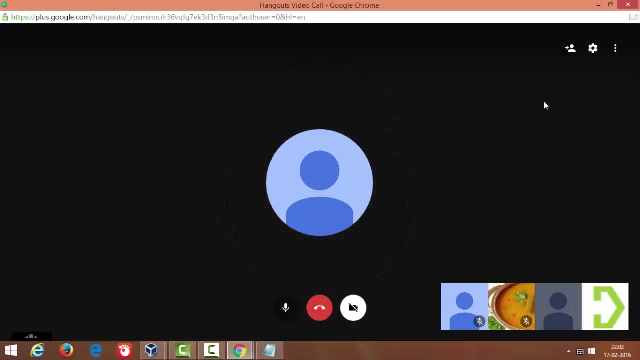 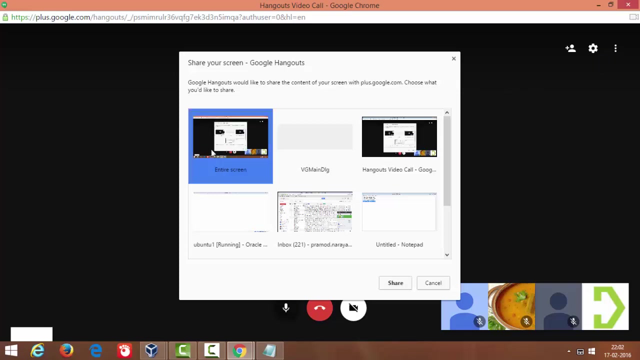 See. Now, They're Not Able To See. My Screen Is Shared. What Are You Able To See? That Is Able To See? That Is Able. 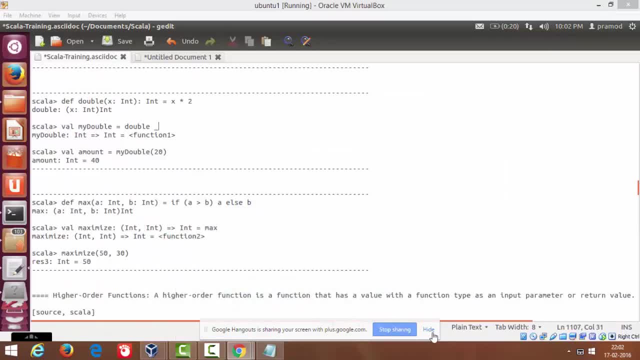 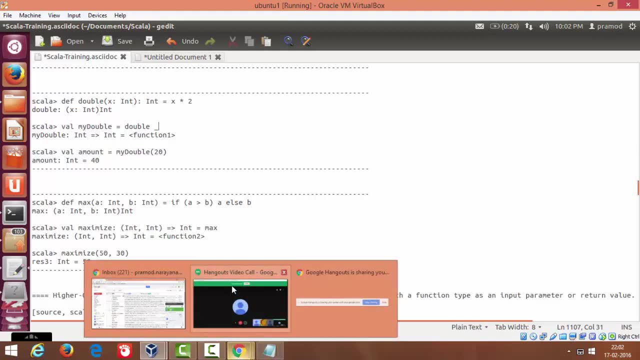 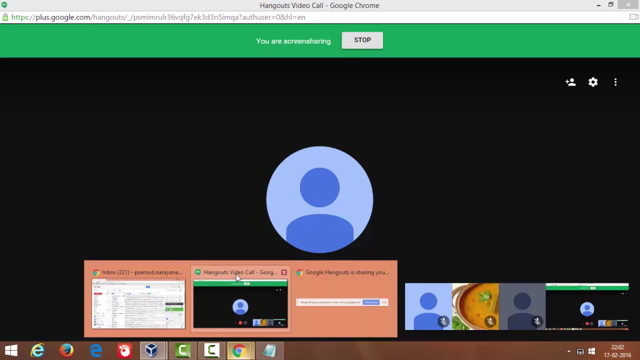 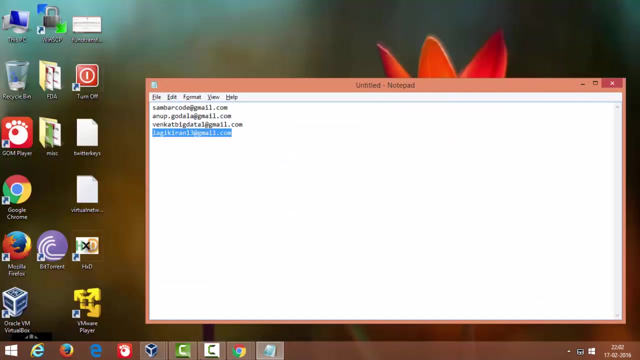 To See. That Is Able To See. Now They Are Passing The Argument Are Passing. That Is Able To See. Now You Are Not Able To. 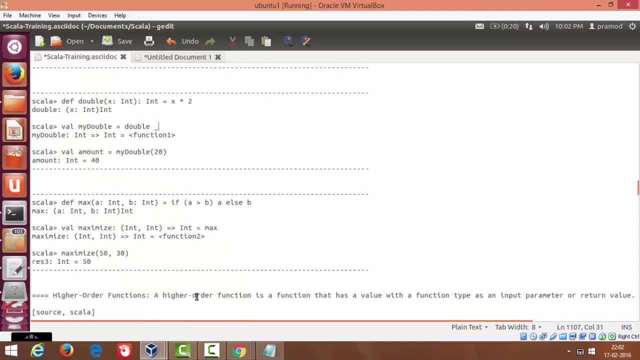 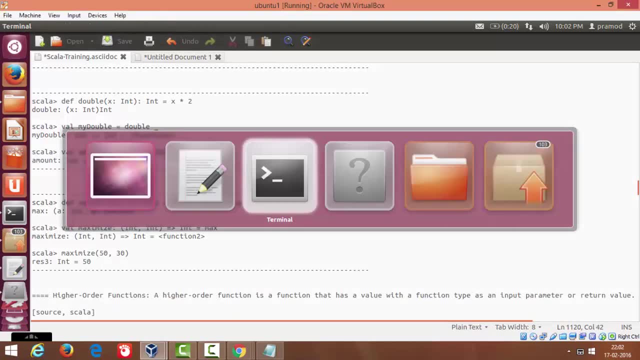 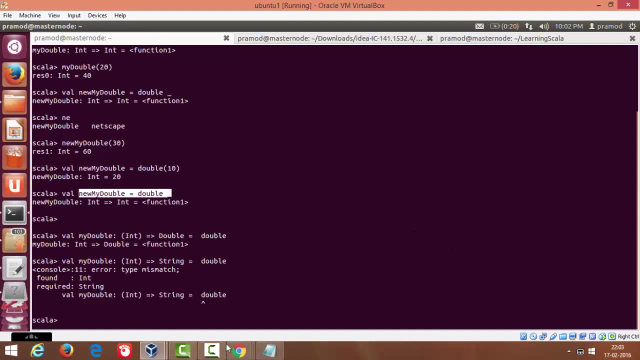 See. You Are Not Able To See. You Are Not Able To See. Even Now, Can You Disconnect And Connect Again. Is It Now Is Able? 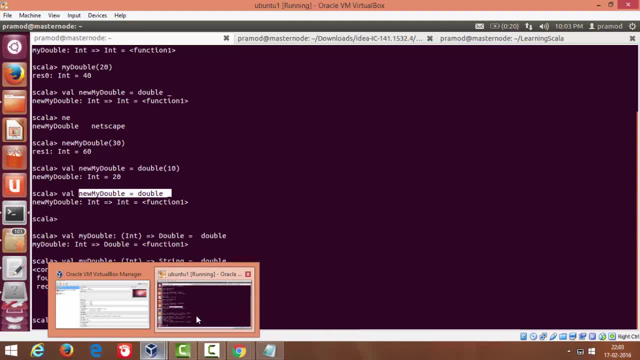 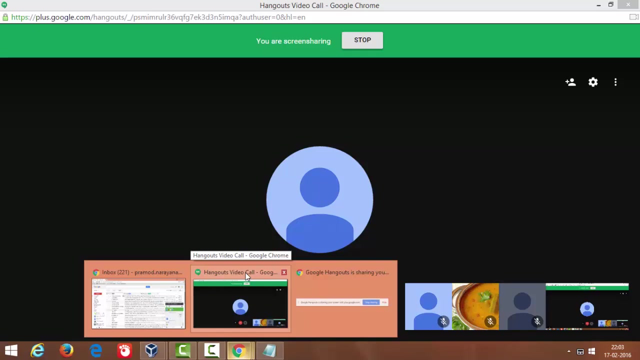 To See. That Is Able To See. Now You Are Passing. That Is Able To See. That Is Able To See. It Is Able To See. 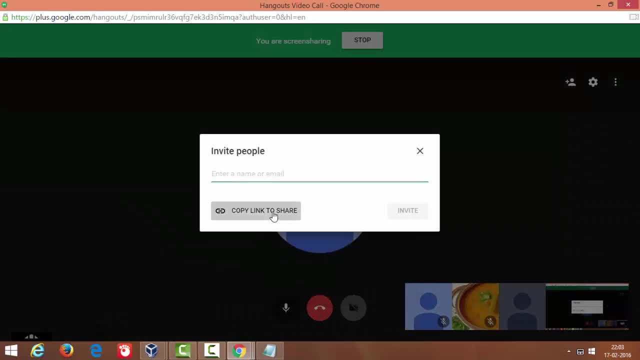 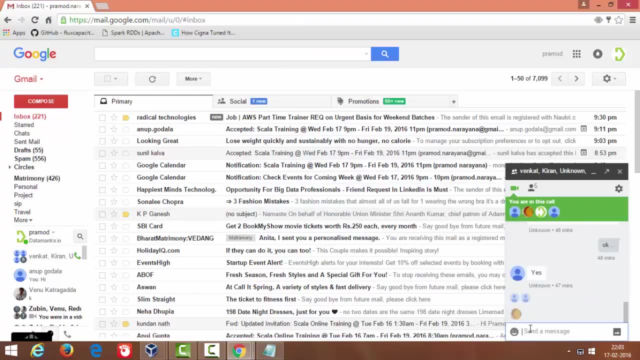 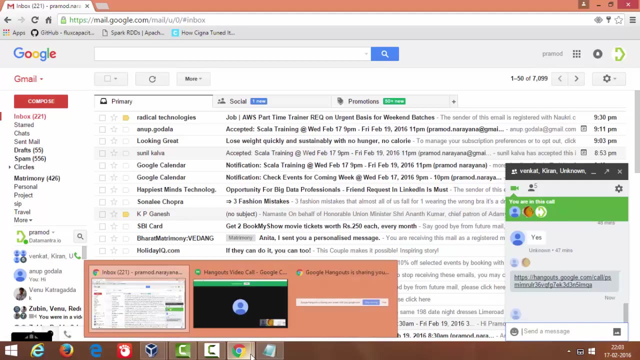 Now Again. It's Now. Is Able To See Again. Is Able To See Now. Is Able To See Now. Office, Now This Took Which To See. 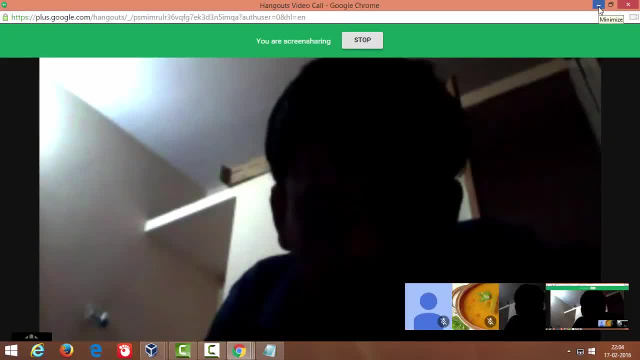 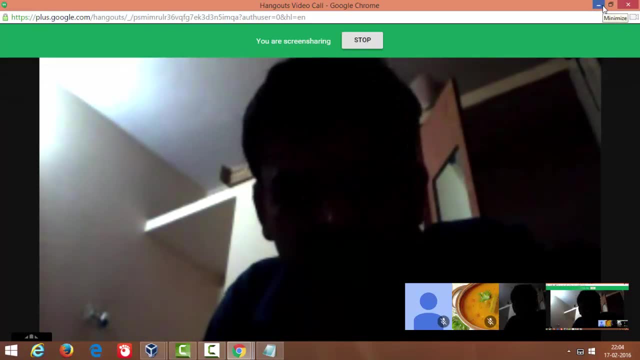 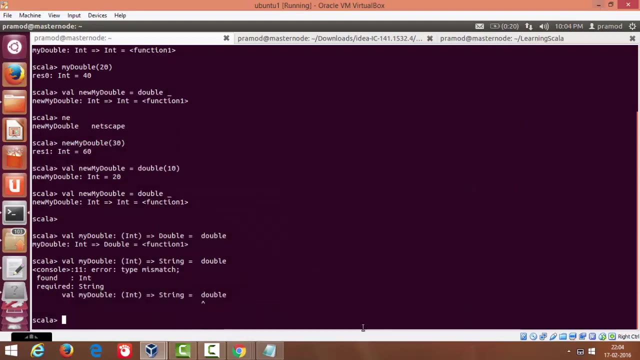 Can Hello, yeah, now able to see uh just mute, pardon, okay, uh just mute yourself, yeah, yeah, uh, things were clear, right, we'll go ahead with next what we have next here. 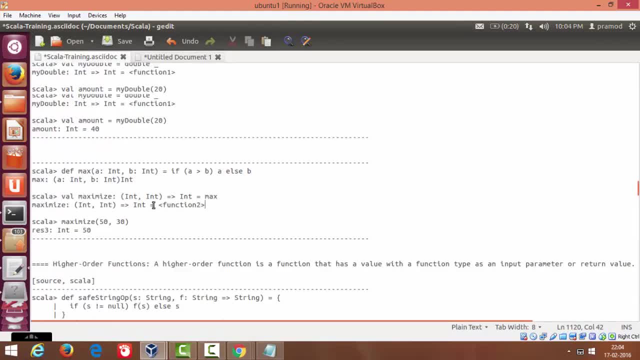 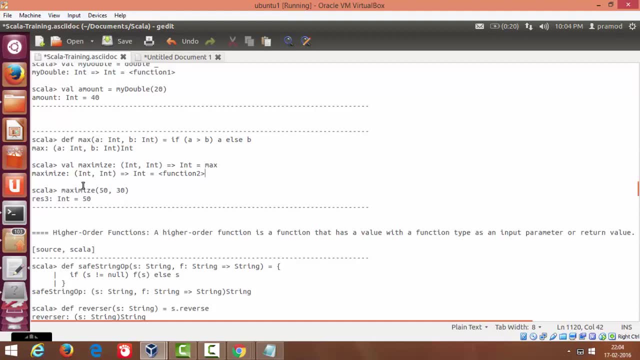 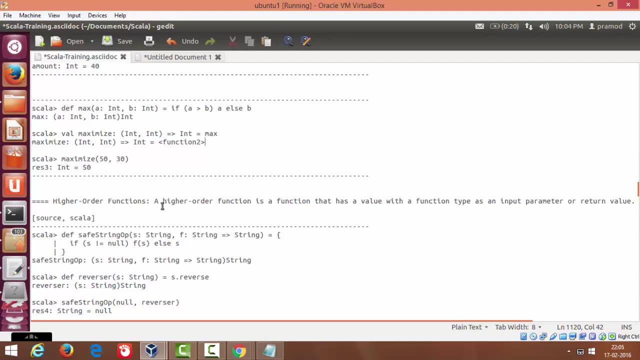 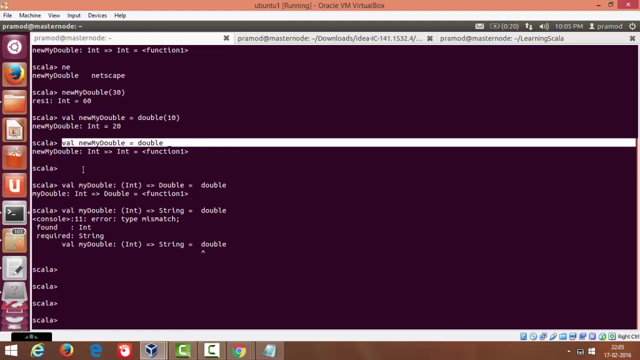 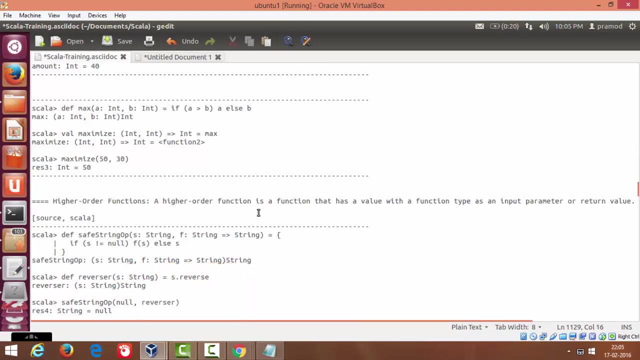 yeah, next we have the higher order functions. a higher order function is nothing but passing a function as a parameter to the function. a higher order function? hello right, this is the one, okay, okay, yeah, yeah, next we have higher order function, a higher order function. 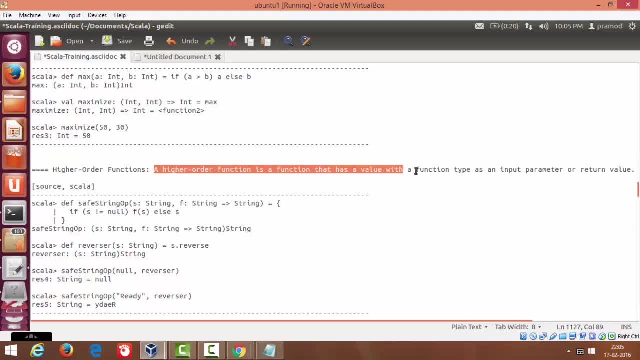 a higher order function is a function that has a value with a function type as a input parameter or a return value means you define a function and to that function you can pass a function or you can return a function from that function. such functions are called higher order functions. 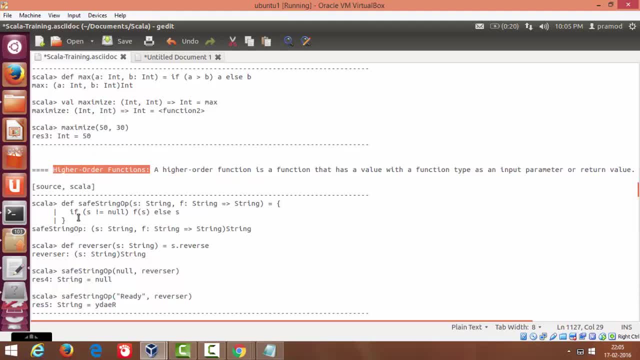 so if you see here this is a higher order function, that's because, okay, if you remember, this is the definition of a function variable. this is a- sorry, this is a data type of a function variable. it means we can pass a function to this function. 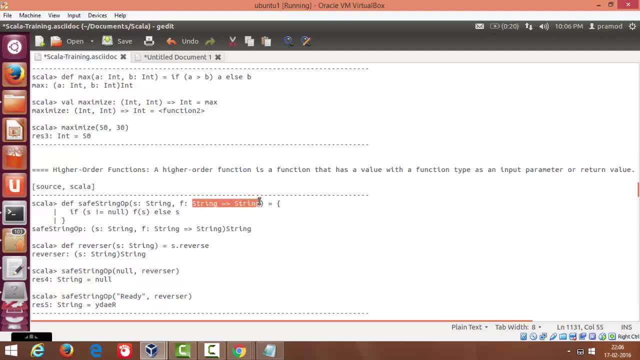 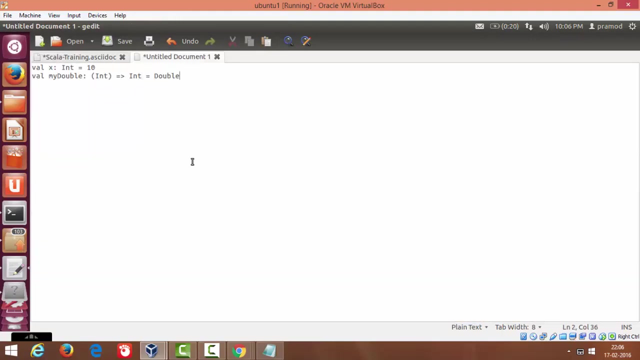 whenever you see this type of data type- we already saw this type of a data type- that means it is a function variable, function identifier and we can pass a function to this function. okay, okay, so let's have this. I think we will see in this. I think yeah. 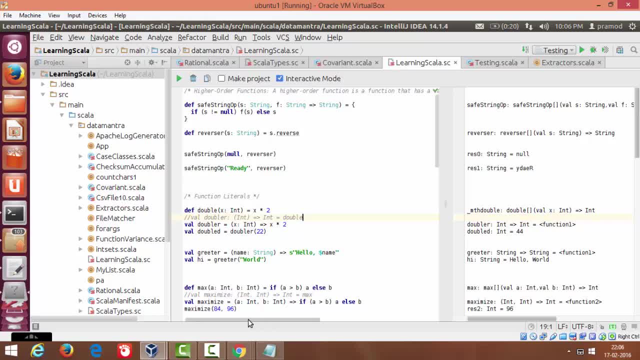 this is much better for those things. so if you see, this is our function, this is a higher order function because it takes function as one of its parameter. okay, so if you see this in the body of this higher order functions, what we are doing, 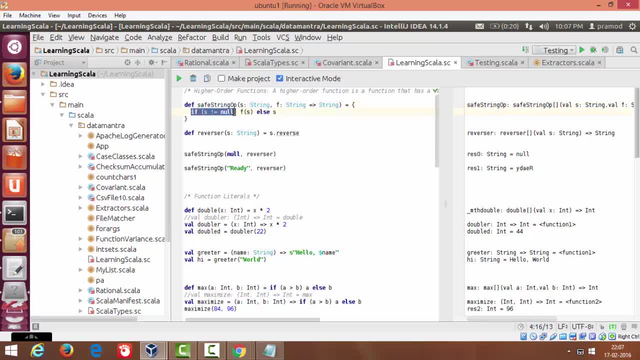 we are checking. if s is not equal to null, then we are applying the function that is passed to this function. then we are applying the function to the first parameter of the higher order function. else we are just returning that function if it is not null. 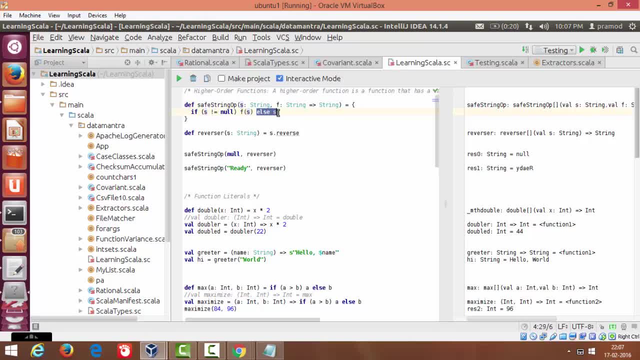 apply the function passed as a function as a parameter. otherwise just return a function. now we are defining one more function here. this is a simple function. it is called reverser, a normal function, just like any other function. it takes s as a string and returns s dot reverses. 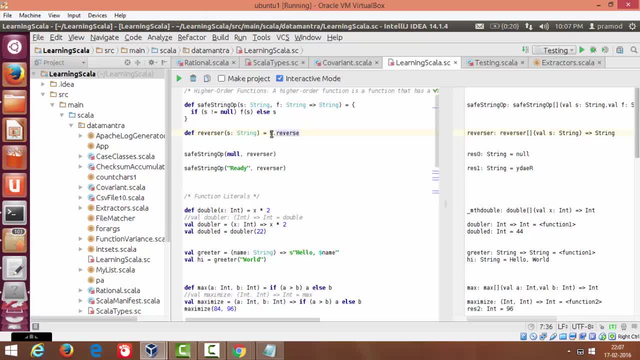 the string here. this is a normal function. it takes a string and reverse a string means the data type of this reverser function is: it takes a string as a input parameter and the return type is also a string, because we are just reversing the string in the body. so we can definitely pass this function to. 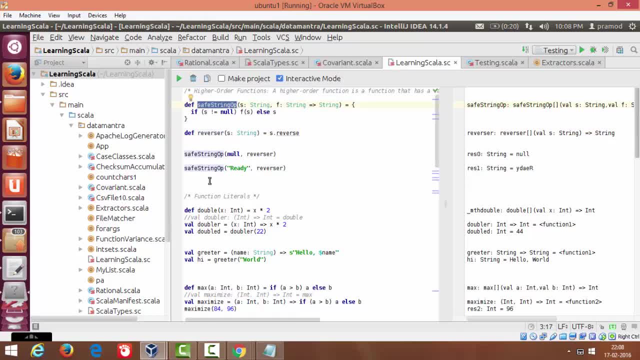 this higher-order function, right, so we are calling this higher-order function. now the first parameter is a string and second parameter is actually the this function, because we have defined the higher-order function as this, which whose second parameter could be a function, so we are passing a function here. so whenever we pass this, if we see 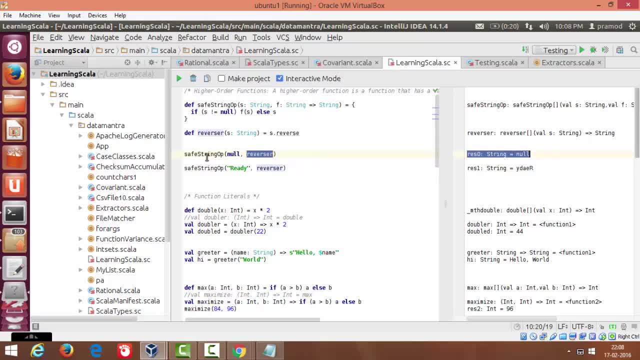 the result is null. this is the output of this function. what is the safe string of this function operation higher order function say: if it is not equal to null, only then apply the reverser function, otherwise just return whatever is being passed to this function. we are passing null, so the return? 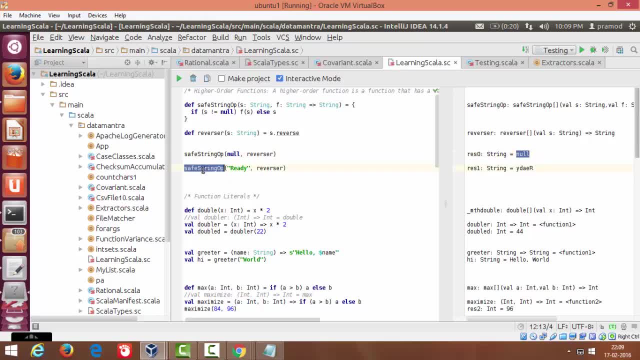 value is null. in the second call to that function we are passing ready and the reverser function, so it is reversing that function and it is returning the value. so you got the idea right why we needed this function variable and this function: data type. this has been defined inside as a parameter to the other function and hence that other function. 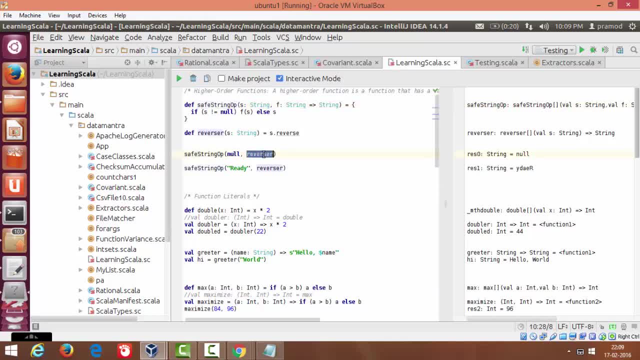 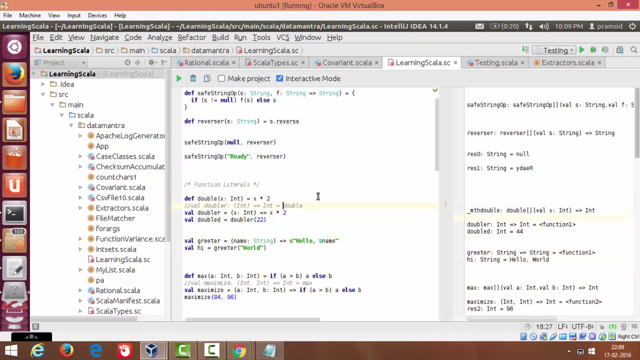 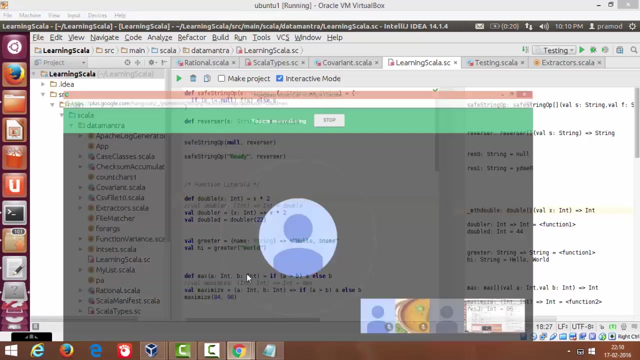 is called a higher order function and we can always pass a function to a higher order function. and any doubts here? okay, any doubts here? any doubts here? any doubts here? Any questions? Okay, Pardon, Yeah, yeah, reverse is a inbuilt function of a string. 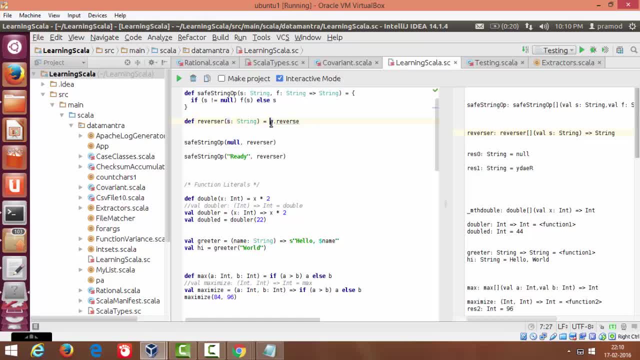 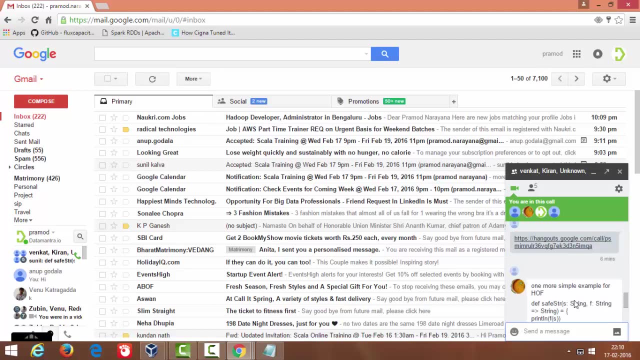 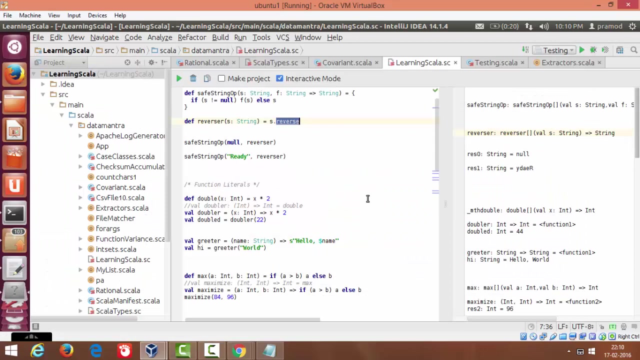 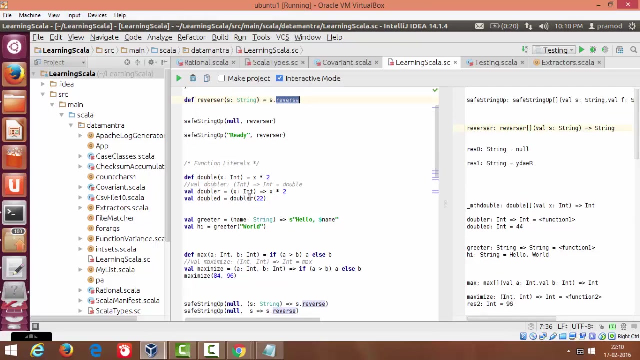 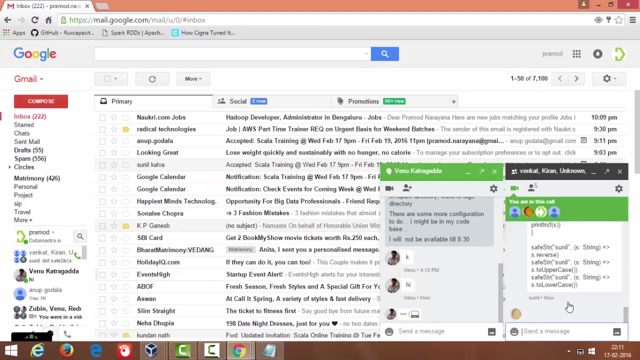 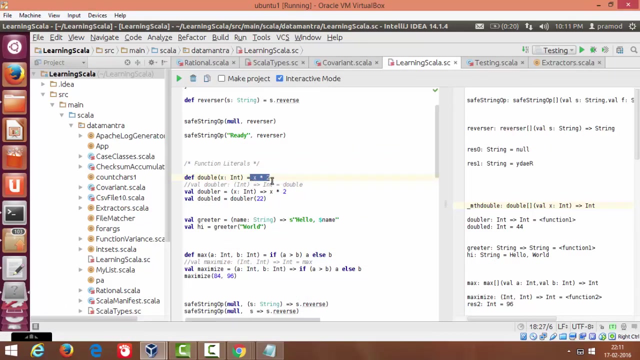 Yes, Yes is a string here. This reverse is an inbuilt function of the string. Yeah means it could be anything, Okay, Okay, Okay. So here we have one more function literals. Function literals are nothing but. Function literals are nothing but. 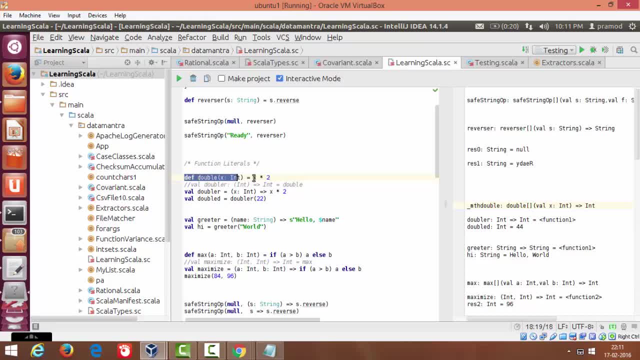 So here we have one more function. literals are nothing but Function. literals are nothing but Function. literals are nothing but Okay. So if we see there are two more functions, We can. if you see, earlier we had. this was a simple definition of the function. 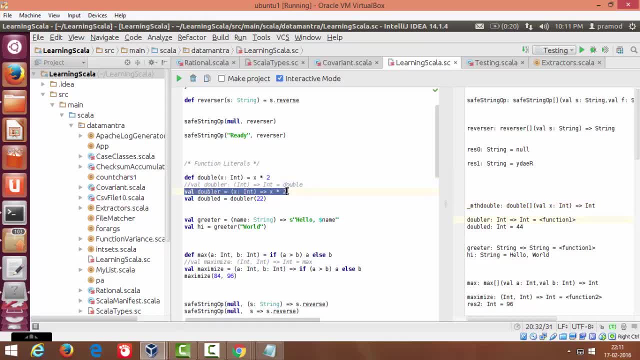 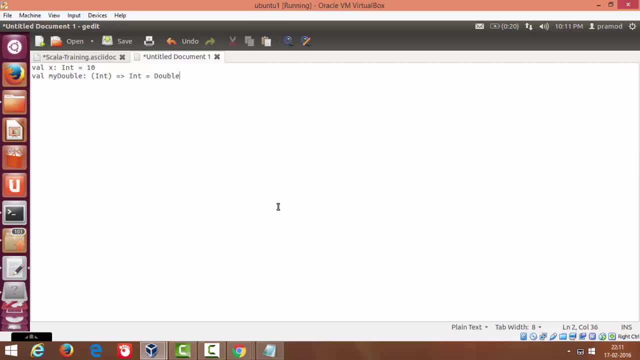 Then we have, instead of Okay, Let me write here itself: This will be much better. We had a def my double, which takes x. This is a function that Okay. Okay, x as int and the value is x, star 2. then we had val my double of the type int, and we are. 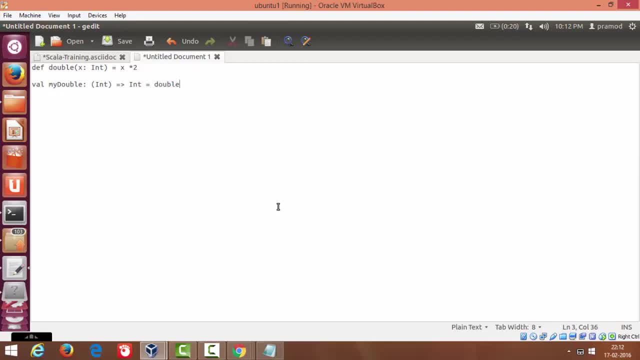 assigning double to this. so what we can do is we can always get rid of this intermediate step. this is the function literal. actually, this is called function literal, the body. you can directly write this body here instead of having this name. we can directly write x, star 2 here, but in that case we need to pass x as a input parameter. so what we are doing 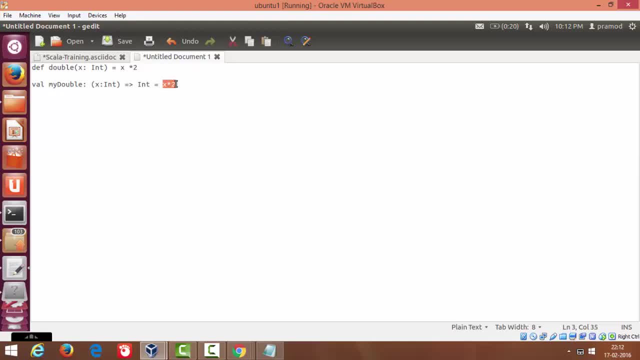 is, we are replacing this function with the body of the function and we are getting rid of this. we do not need a intermediate definition of a mydouble. this is a function without a name. to a function there is no name. it's just a body literal. the literal has been given here. we need not. 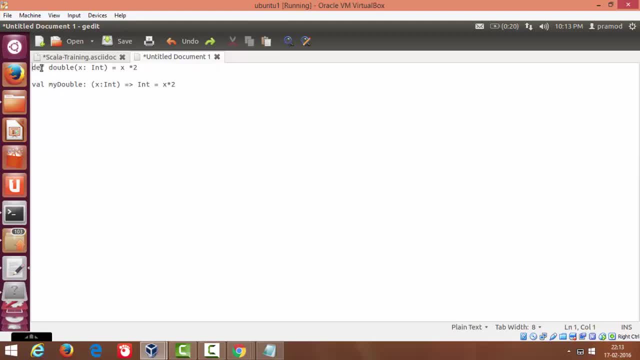 this intermediate step is not at all required. define a function, then assign that function name to this function variable. that is not required directly. earlier it was in this fashion. now we will directly replace the body here. this is nothing but function literals. so we can directly get rid of that intermediate function variable. we can directly place a. 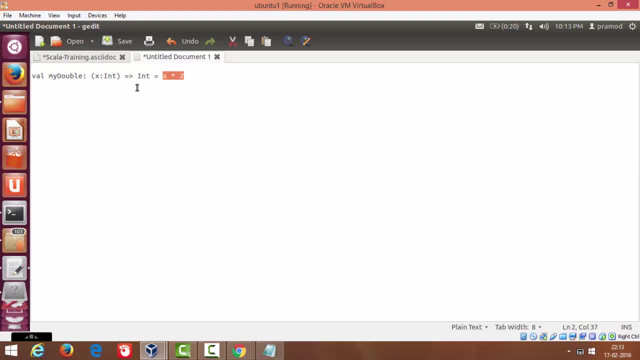 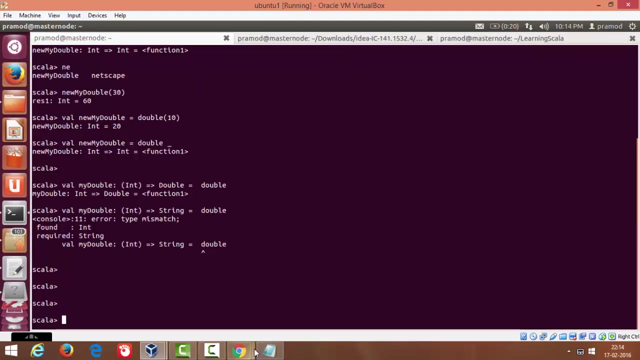 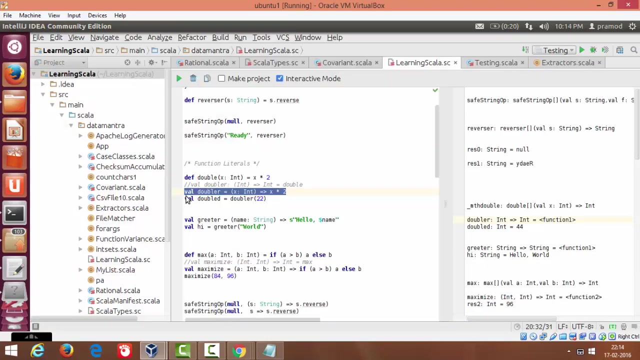 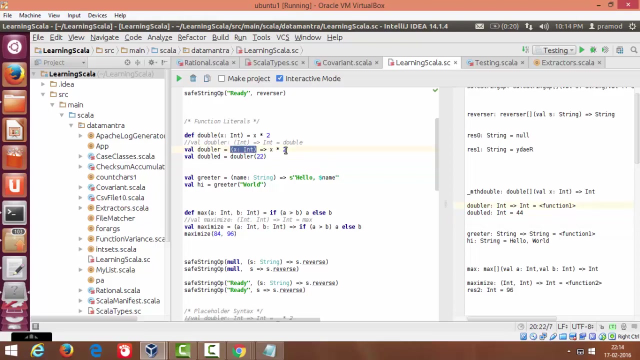 body here itself. this is again a function variable which takes an x as a identifier- integer, and its return type is integer. this is also a valid scenario where the literal is replaced with the actual function name. we don't need a function intermediate function name at all. yeah, this is what we are doing here again, we can. 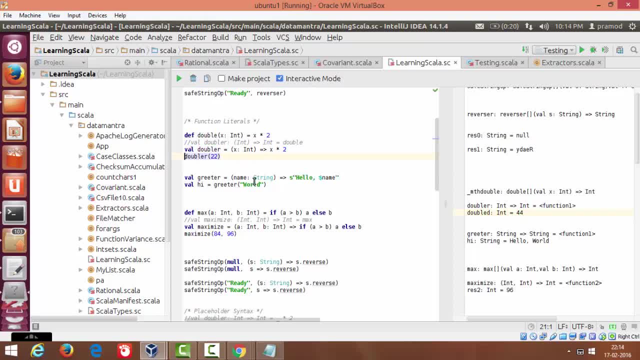 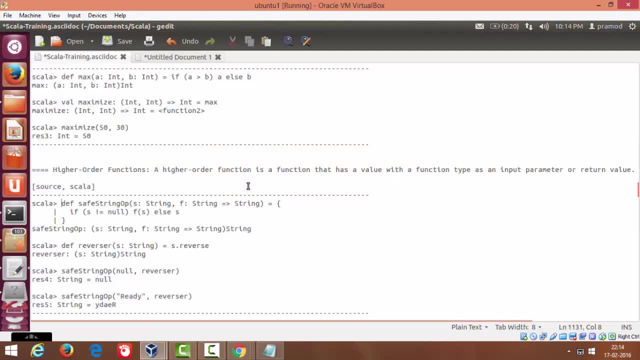 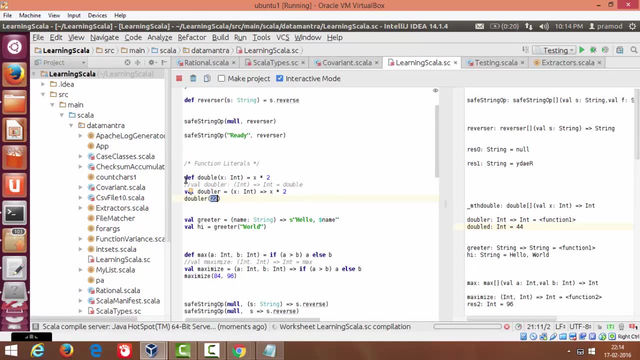 we can call this doubler with actual value. you got the idea right. we need not have this intermediate step, this intermediate step. we need not have this intermediate step. we can directly replace this, this function, with the body of the function. In that case, we need to pass the argument. 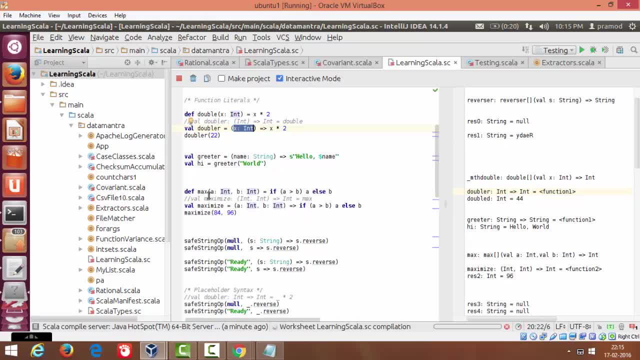 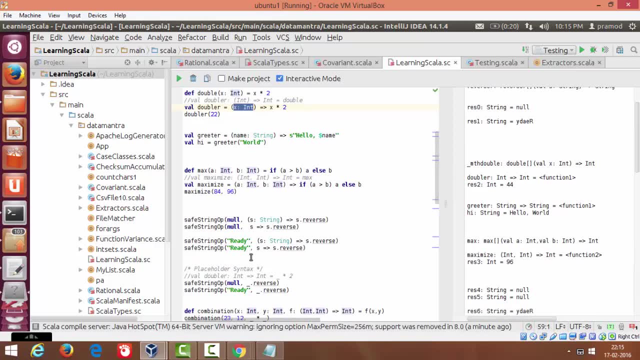 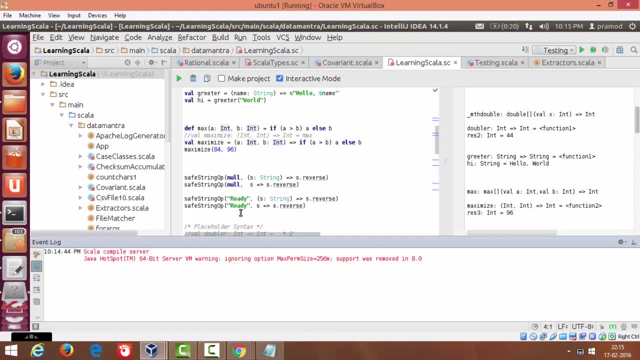 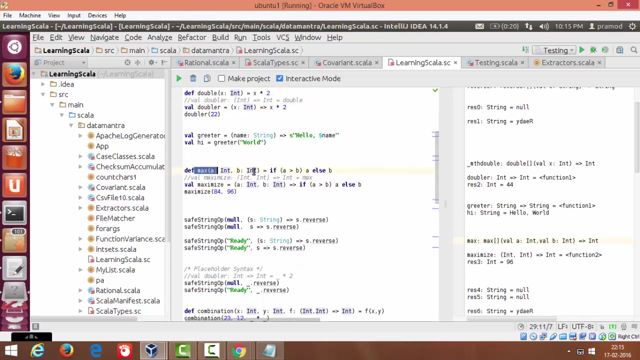 Any questions there. If you see, earlier we had max. was defined max of a- b. If a is greater than b, return a b. If a is greater than b, return a b. If a is greater than a, else return b. Then we defined a function variable and assigned: 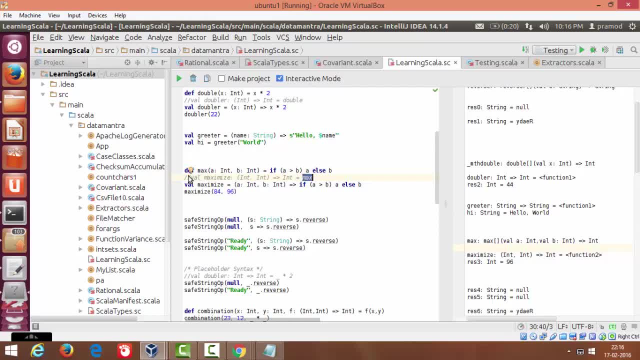 max to that. So now that is not required. This intermediate step is not at all required. We are directly putting the body of that function in our function variable. So in that case we need to pass the actual arguments. So we are. 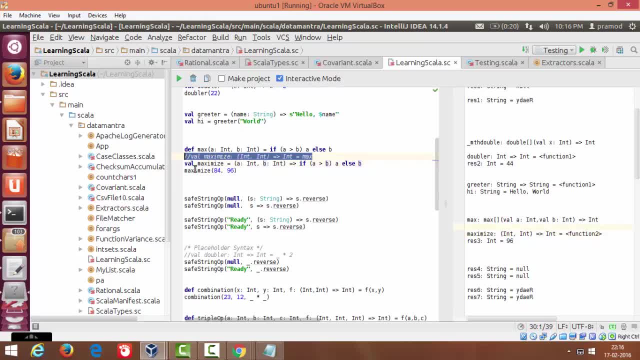 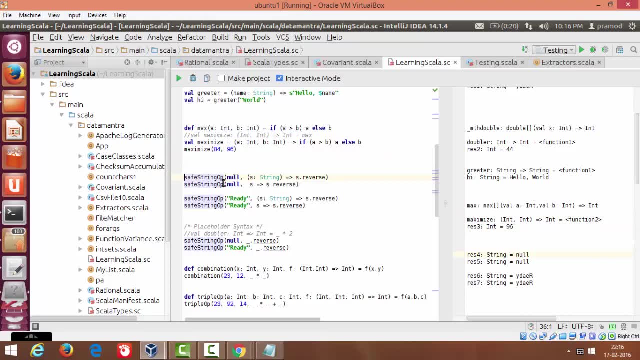 minimizing one step here instead of having these things. So again the same in our case. As we said, we can do two upper, Because the reverse and reverse our answer confuses. As Sunil said, we can do it in this fashion. 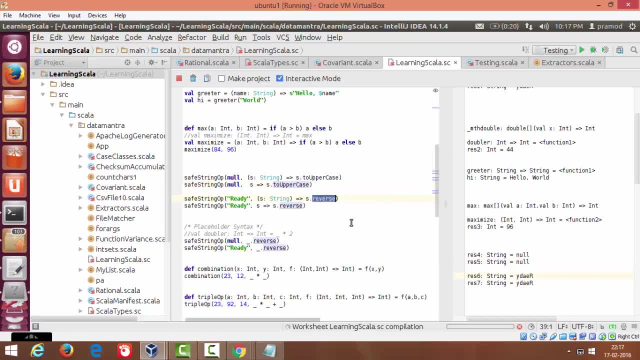 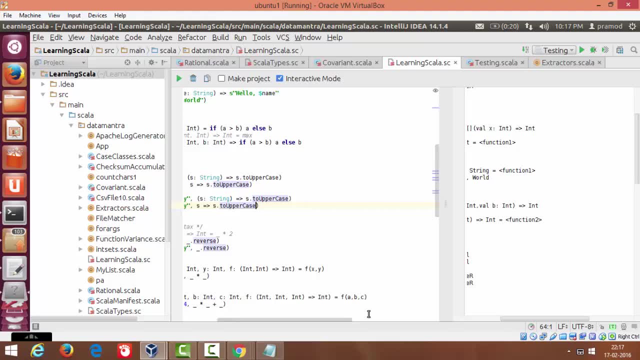 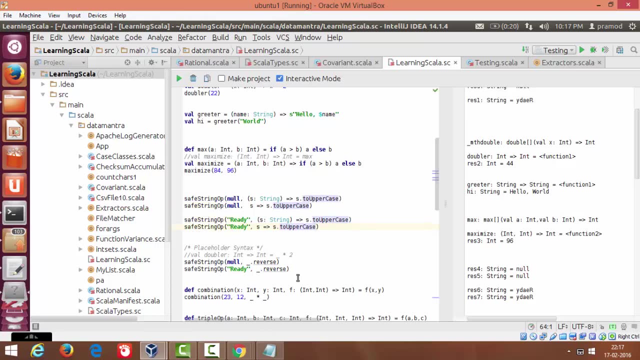 yeah, here also we are the same thing. whatever we did here, the same. okay, same thing. whatever we did here, we got rid of this intermediate function variable. the same thing. we are doing it for the higher order functions. 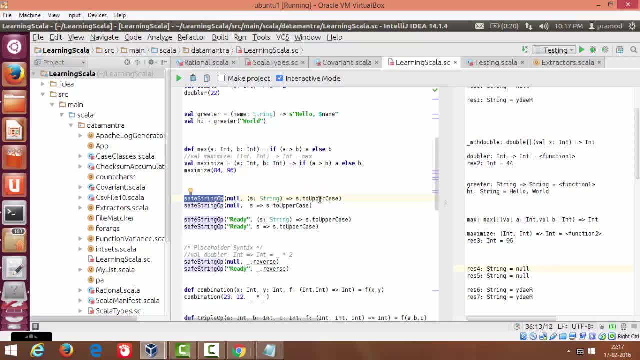 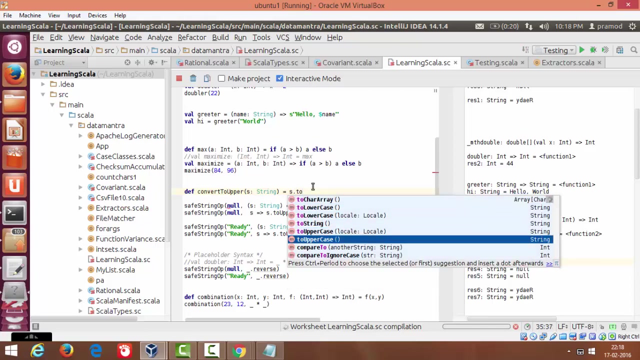 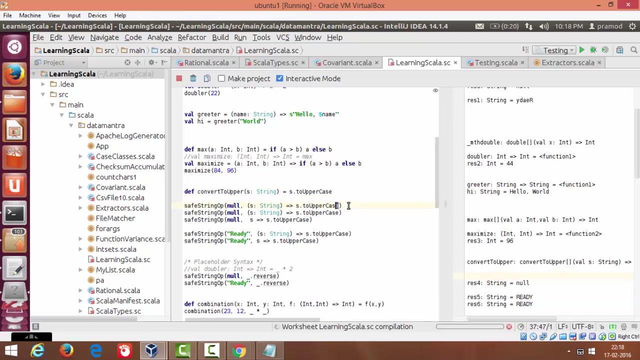 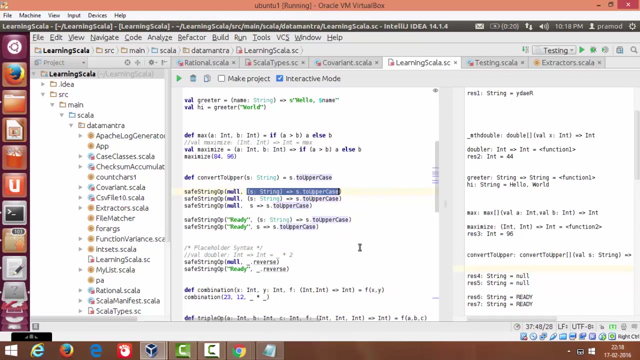 instead of defining a different function, like, instead of defining like convert to upward, and passing string which does s dot to uppercase, which does s dot to uppercase, and then passing this. let's see, you see, instead of doing doing this way, like this, you see, instead of doing doing this way, we define a function. 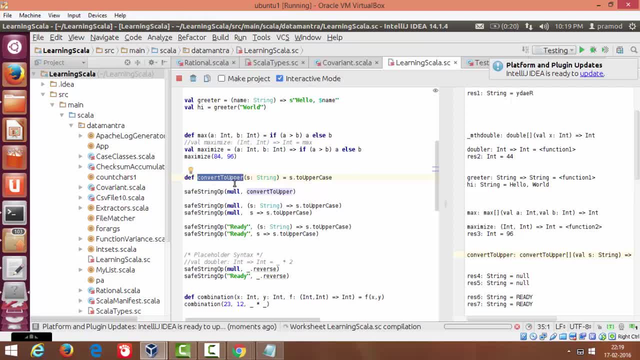 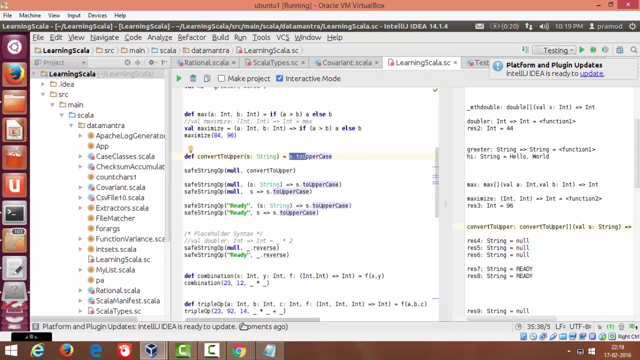 which convert to any anything you pass as a string. it converts to a uppercase and then pass this string from this order string to another side and then we are gonna give function to. this is what we were doing in our earlier example: we define a function, then pass this function to this higher order functions. but in the 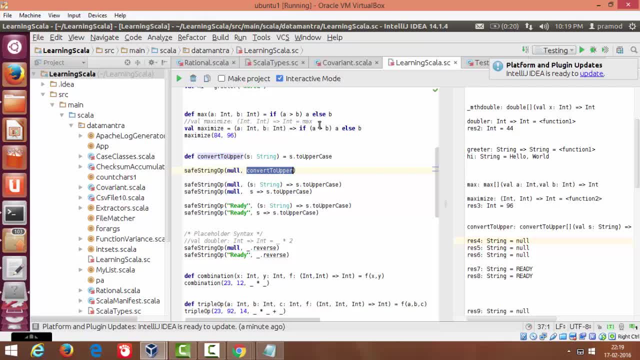 previous examples, we saw that we can directly replace the body instead of calling the. instead of passing the function, we can directly replace it with the body of the function. so, instead of doing this way, we can directly pass the body of the function or pass the argument and the definition of the. 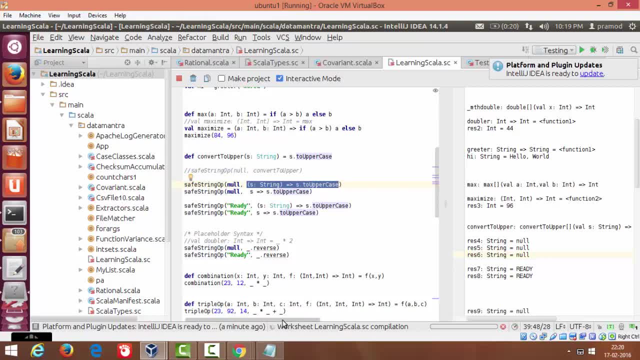 function directly to this function, to the higher order function, since, since the data type is inferred, we can get rid of this data type. the data type is inferred, we can get rid of this data type, the. that's what I am doing in the second. I am writing the same function because 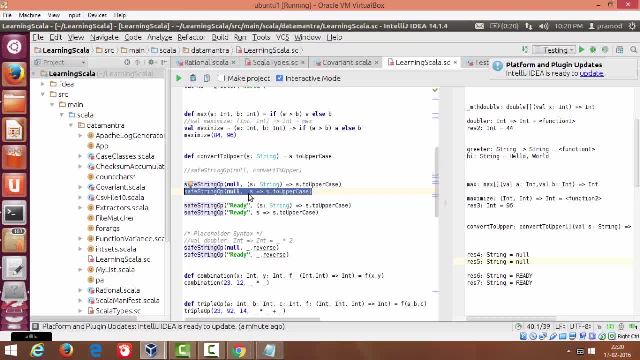 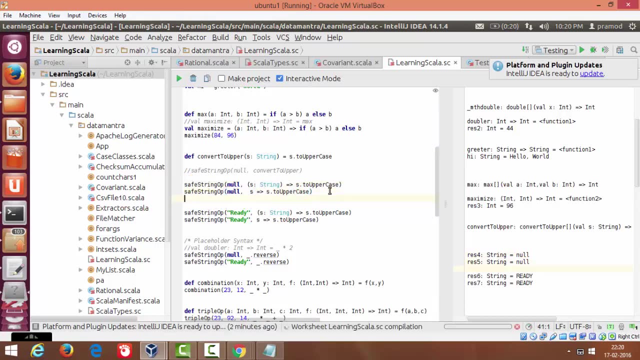 data type is inferred by the compiler, so you need not specify the data type. also earlier we specified string, but that string is not required. the data type is inferred also. again it could be shortcut. already we have done a shortcut. again the shortcut is possible so we can write the same function again. 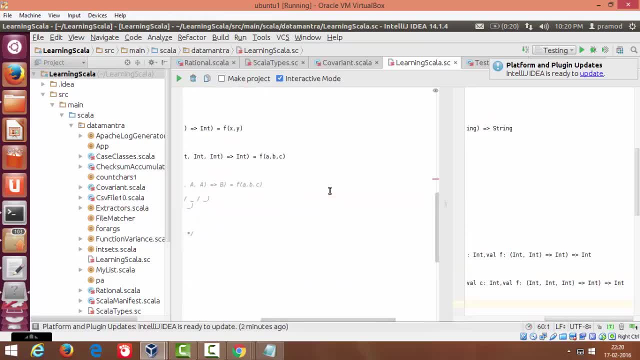 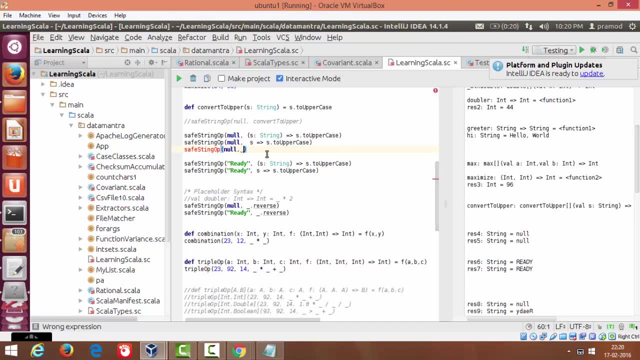 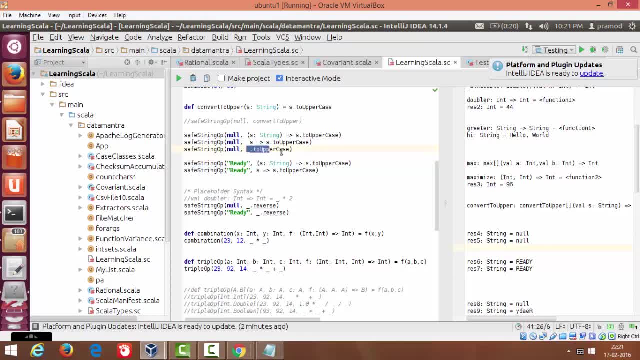 two parameters. the first parameter, this is the definition of the body of the function. we can directly pass the body of the function as a parameter and here underscore is the parameter of the higher order function's function. so if there are two parameters, the first- underscore will be the first parameter and the second parameter will be the second. 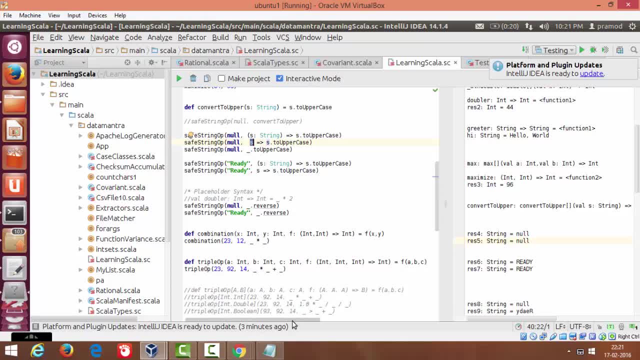 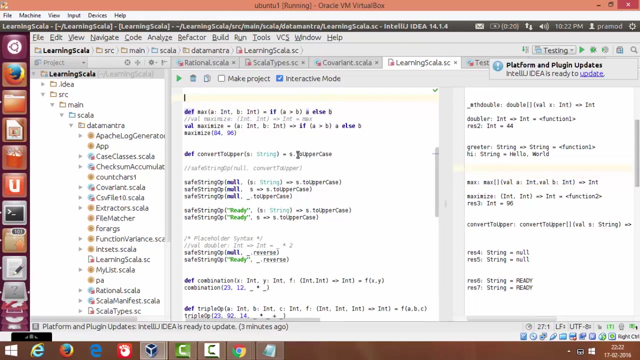 underscore will correspond to the second parameter. so I hope it's bit cryptic. please do ask questions. if you have any questions, or did I lose you guys? hello, okay, so one more time I will will explain it. This is our higher order function, The definition of this higher order. 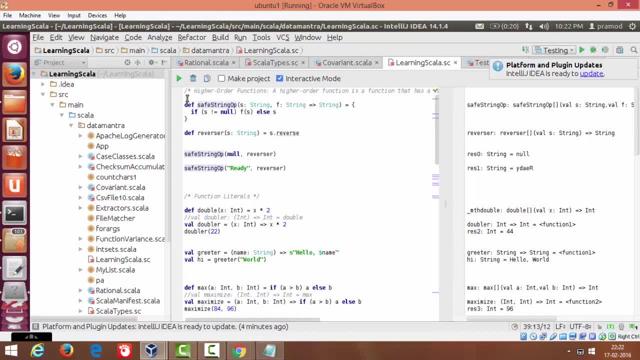 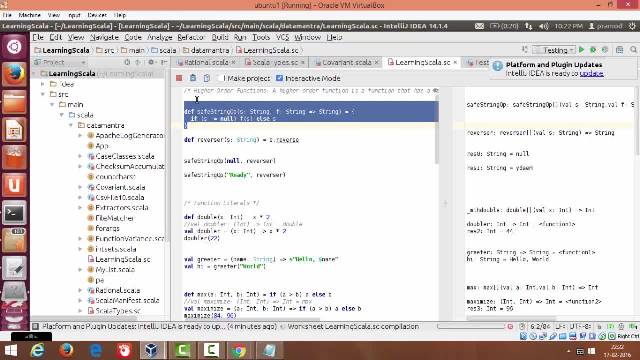 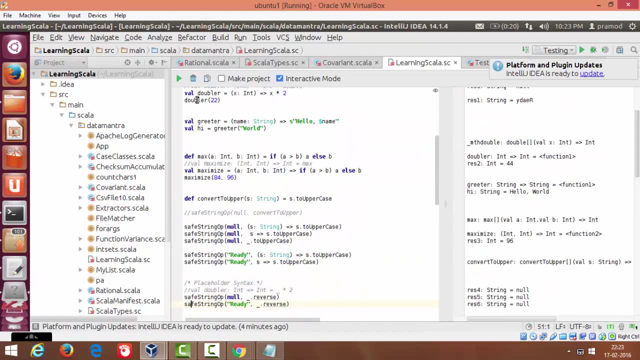 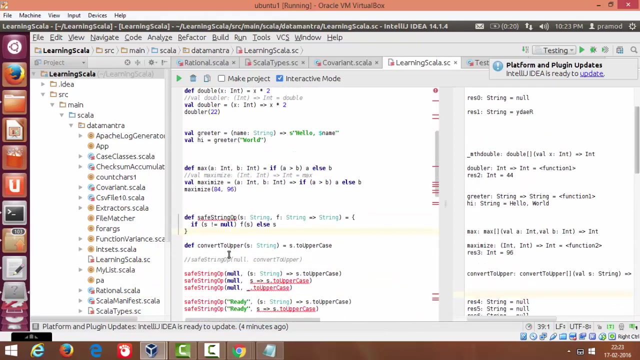 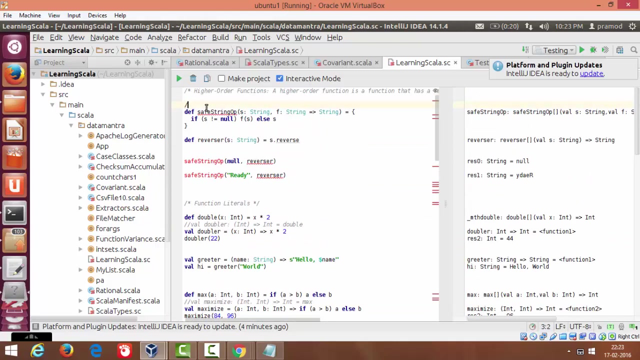 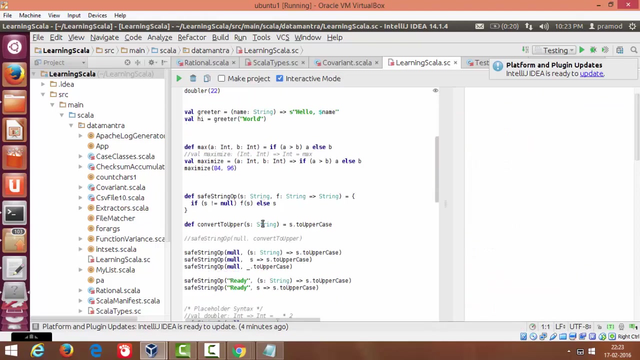 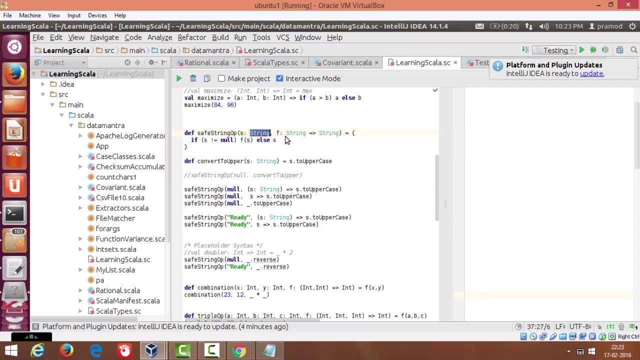 function is. let me put the definition here itself. So this was our higher order function. Just ignore these errors, because I am defining two times the higher order function. Yeah, this is how we defined our higher order function. that takes first parameter as a string. 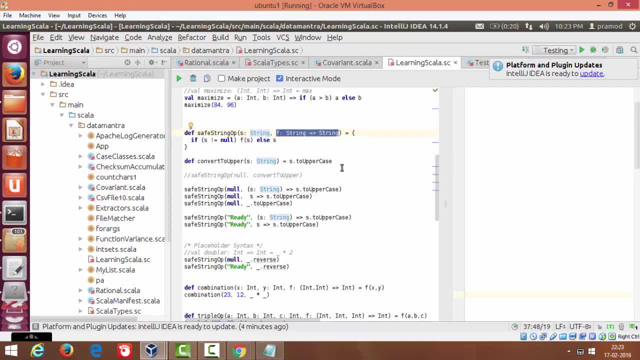 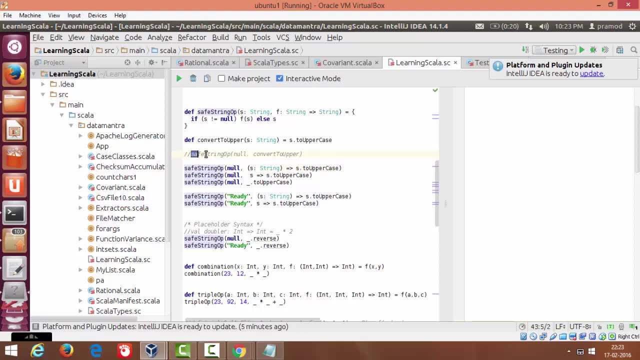 and second parameter as a function. Now we are calling our function Using this higher order function. here we could call in this fashion: also: We can call the higher order function as passing: the first as a string and the second is this function. This is a function that takes input as a string and it returns upper case, which means the. 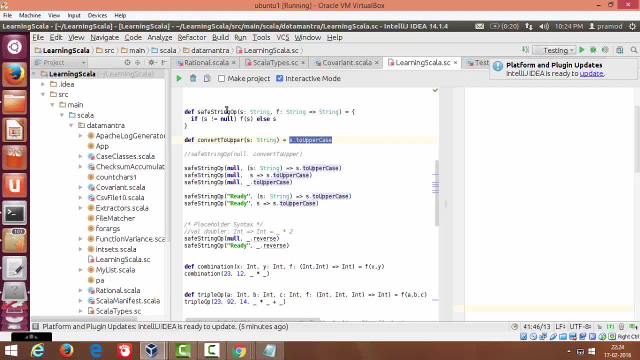 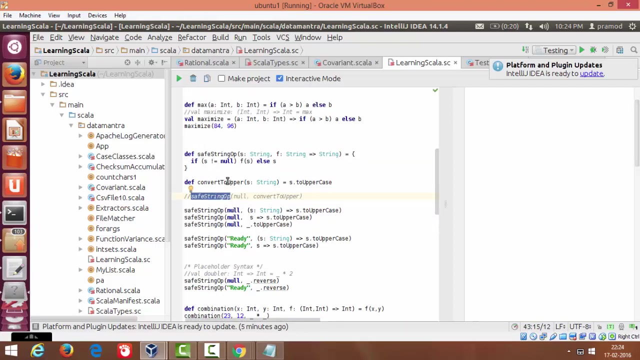 return type is also a string. Since we have defined our higher order function, which takes a function which has input as string and output return type is string, So we can always pass this function as a function to this higher order function. So we also saw that instead of having a name defining a function and then passing that, 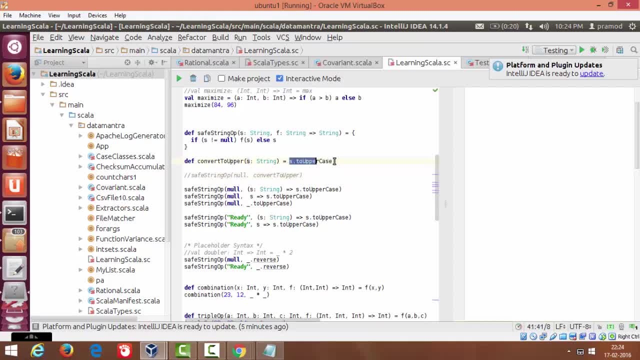 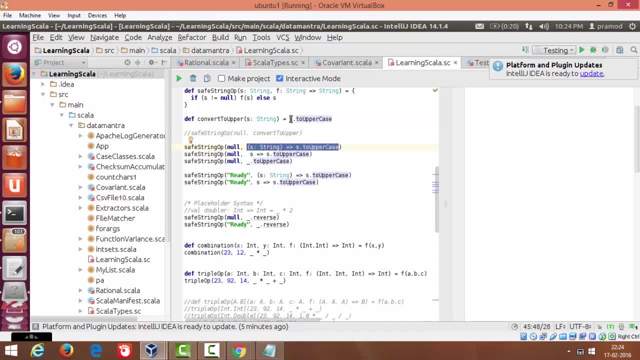 function as a higher order function. we can directly put this body in place of the function variable. We can directly put this. we have to pass the argument. This is how we are passing the argument. Again, we know that Scala will. this is a shortcut way of doing passing the literal of the function. 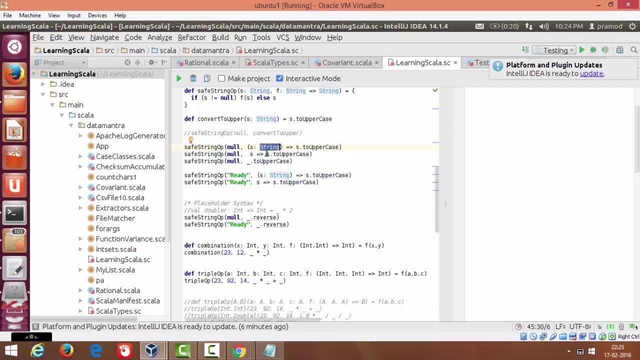 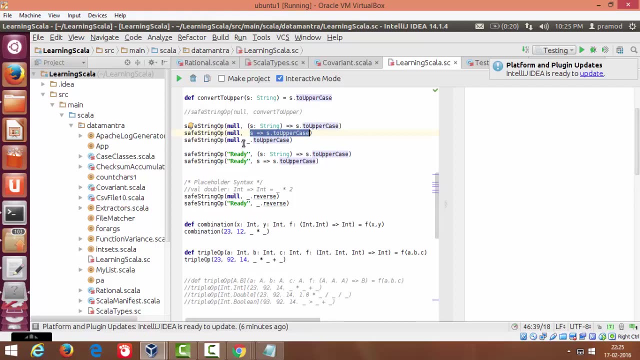 Then we saw that the data types is always inferred by the Scala compiler. So we can always get rid of the string data type because the Scala compiler infers for you, And again we are doing: get rid of getting rid of the actual parameter. A parameter can be replaced. 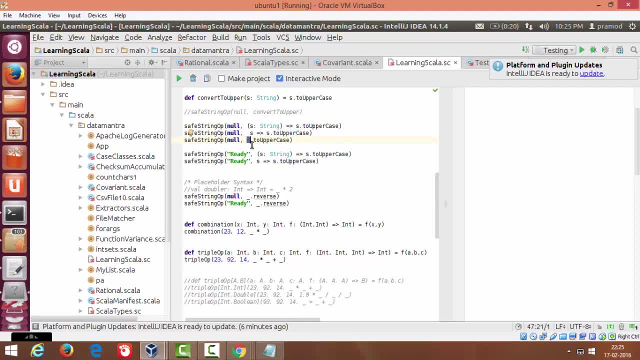 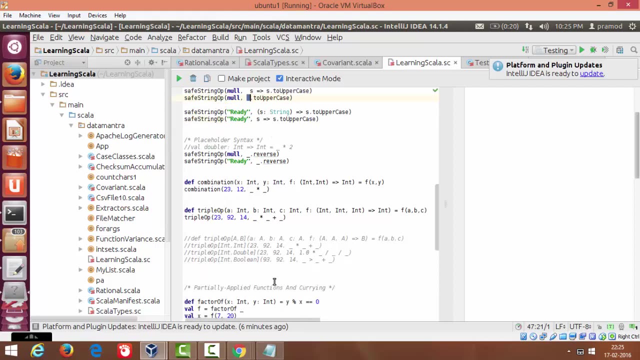 with underscores. Underscore is a placeholder for the parameters. If there are two parameters, the first underscore will correspond to first parameter and the second underscore will be corresponding to the second parameter. We will have those examples Again. if you see here the same examples. 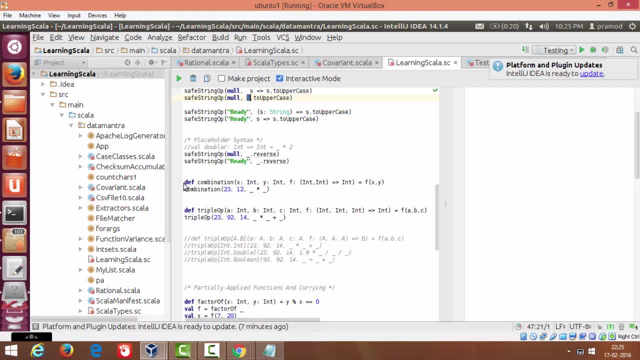 with two parameters we are defining. Here is a function higher order function that takes two integers. that takes two integer parameter as the first two parameters and the third parameter is a function variable. And that function variable again takes two parameters- int parameters- and return type is again int. What we are doing, just doing. 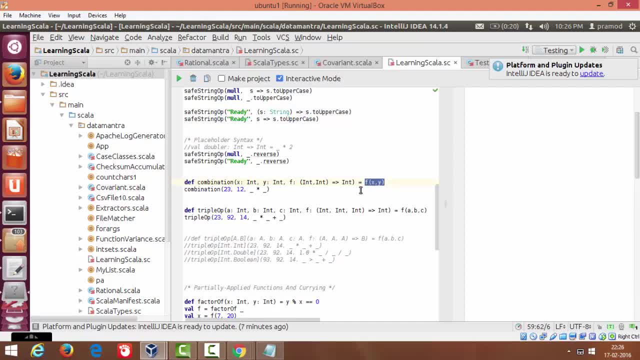 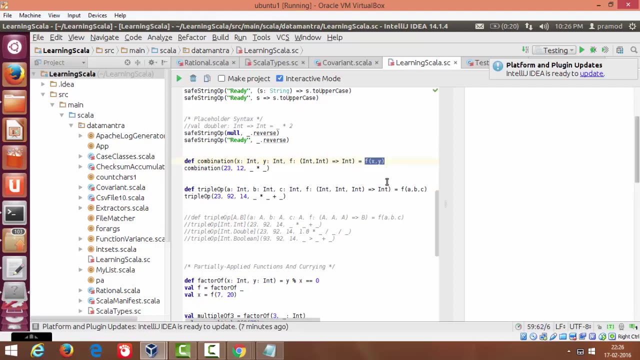 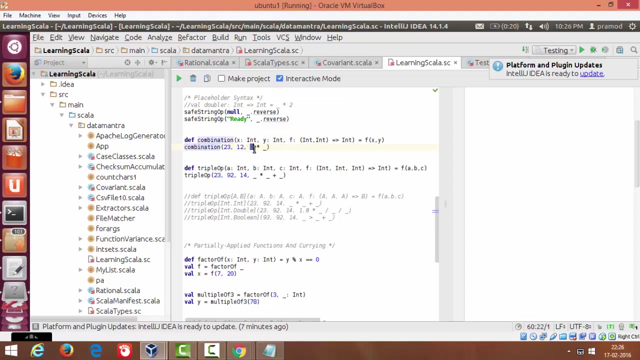 f of x, comma y, which means we are applying this function to the arguments first, two arguments of the higher order function. We are just applying that function. So how can we call this function? We can call this function in this way. Here the first parameter corresponds. 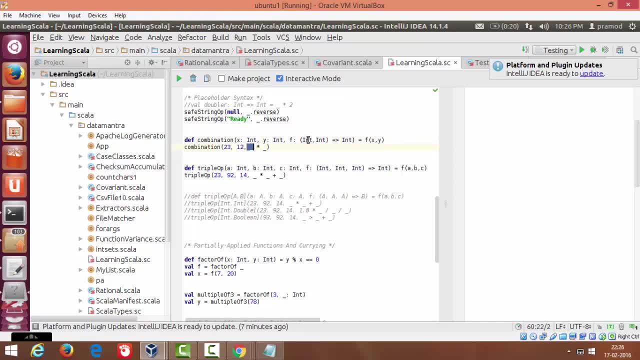 to this. first underscore f of x comma y Second underscore corresponds to this parameter. So we are directly specifying the body of the function while calling the higher order function. So this will actually replace this. It will do x, star y. Here x and y are 23 and 12.. So the placeholder will be the always. 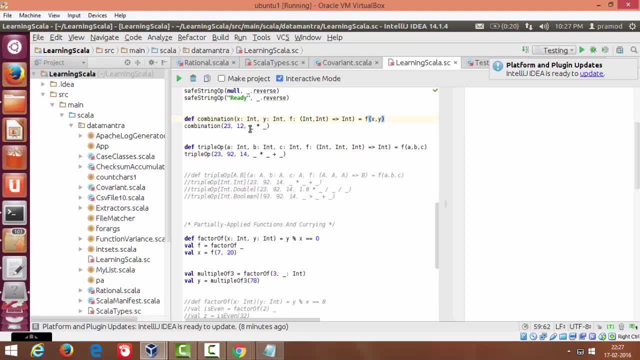 first parameter, The first underscore will be first parameter, depending upon the number of parameters, the placeholder, depending upon the context, the underscore meaning of underscore differs. earlier we saw that in pattern matching underscore was like default case: any. it will match any, anything in the pattern matching and also 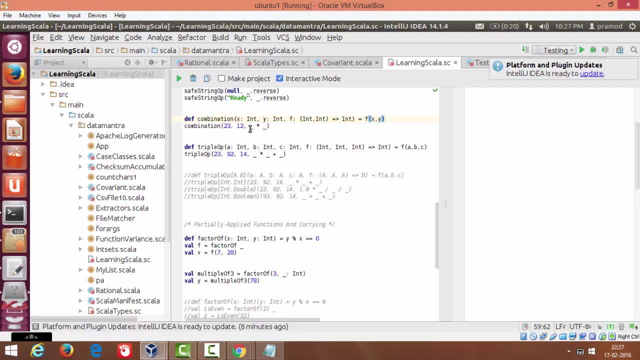 in doing import. if you see, in java we do import some libraries dot star, it means it includes all the classes in that libraries. but in scala you can use a library dot underscore: it means it includes all the classes in that library. so, depending upon the context, the value, 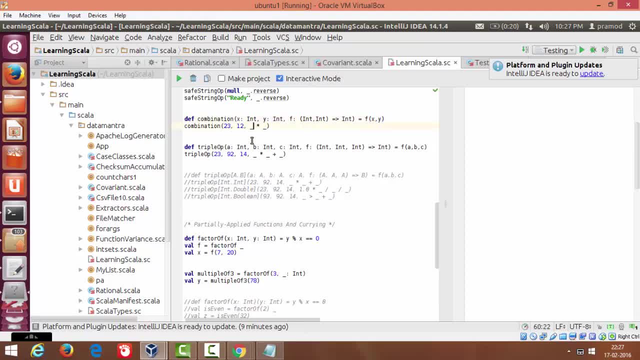 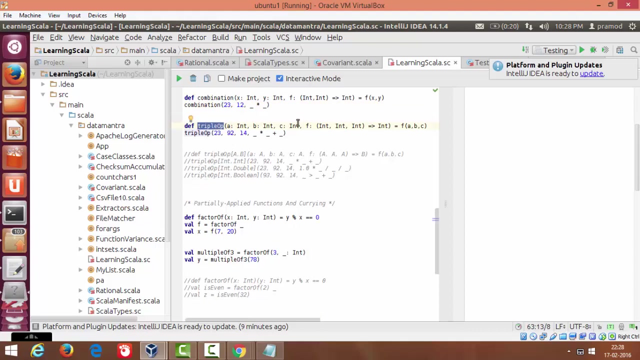 the definition of underscore differs. in pattern matching, it was used to match anything and in higher order function, it is used to match the parameters that is being passed. as to the functions of the higher order function, similarly, we have a triple operation. again, it takes three integer parameters and the last parameter is an, a function variable, which takes three. 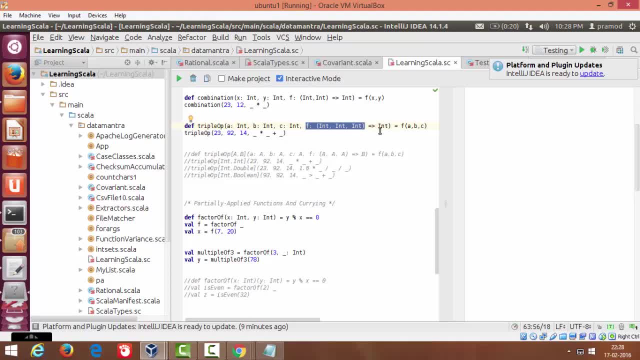 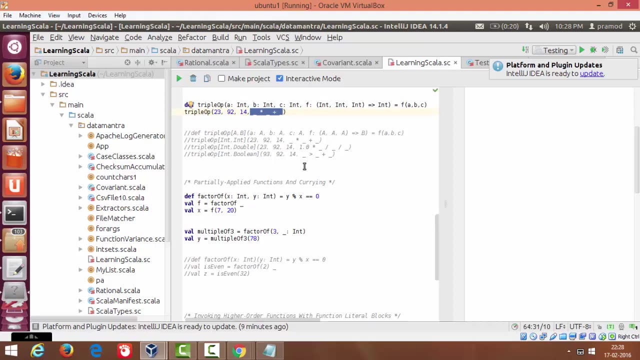 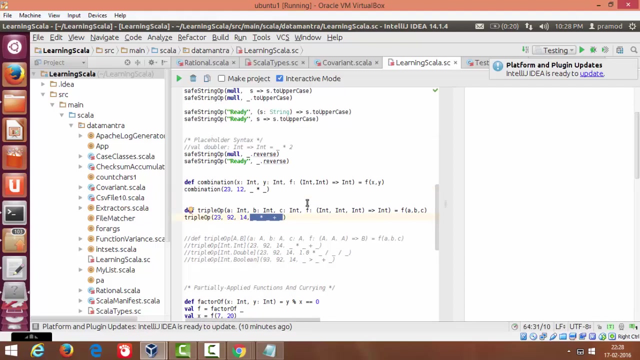 ints and the data type return. data type is int and it applies on the and the function applies on the past parameters to the higher order function. again, we are defining the function here itself. so this is our. this is how a higher order function looks like. we pass a function to it function. similarly, we 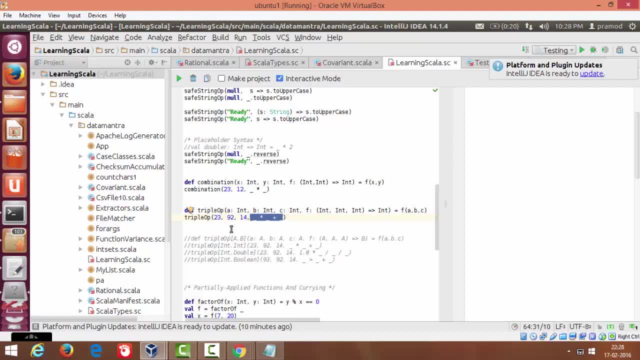 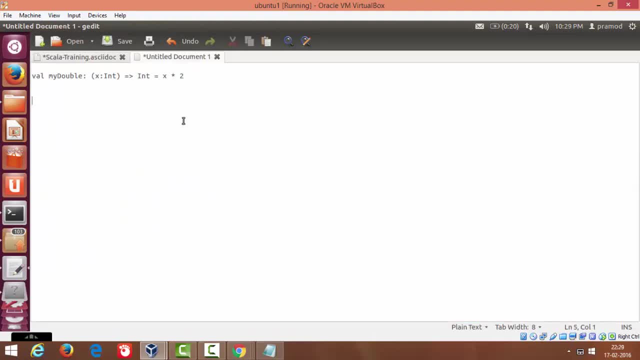 can return a function from a function. when we return a function from a function, how it looks like we can have: def- higher order function takes int. then f is a function that takes int and returns int and we can have this function to return some function itself. in that case, the return type of this higher order function. 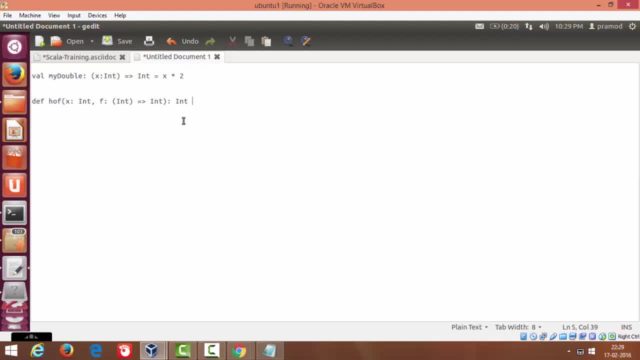 will be like in this way. this is a definition of a higher order function that takes one of the parameter as a function and it returns a function whose data type is it? that function takes int as a parameter and returns return value of that function is int. this is also. 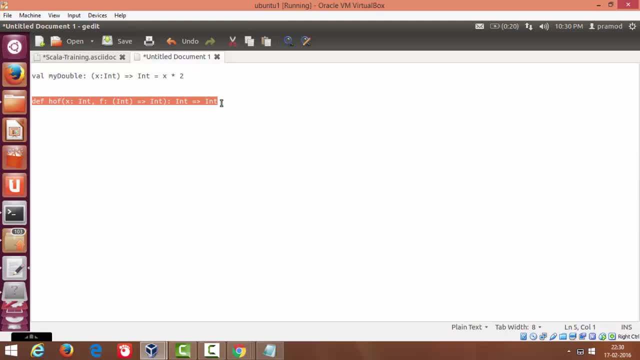 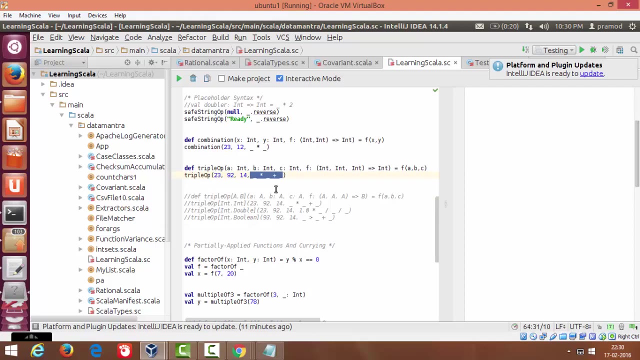 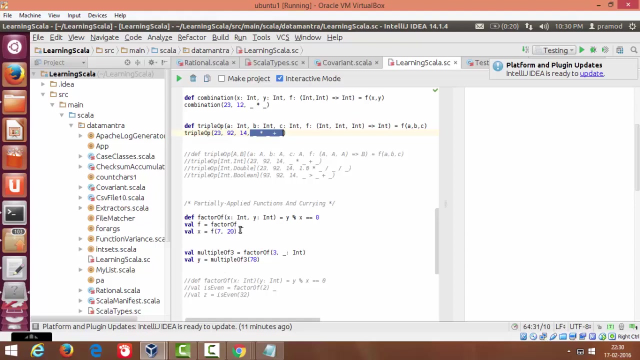 a valid function. Here we are returning a function from the function and also we are passing argument as a function. this is also a valid syntax. see. now we will see the use of this partially applied function. whenever we specify underscore, it is called partially applied function and 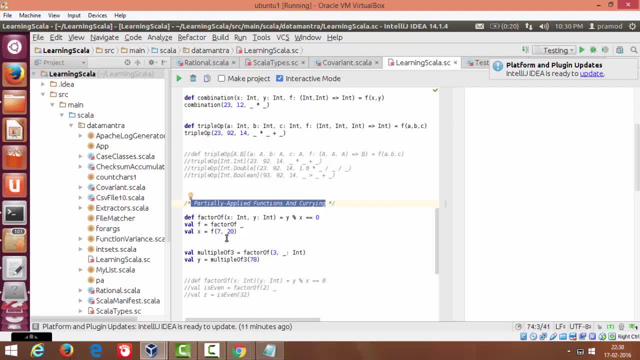 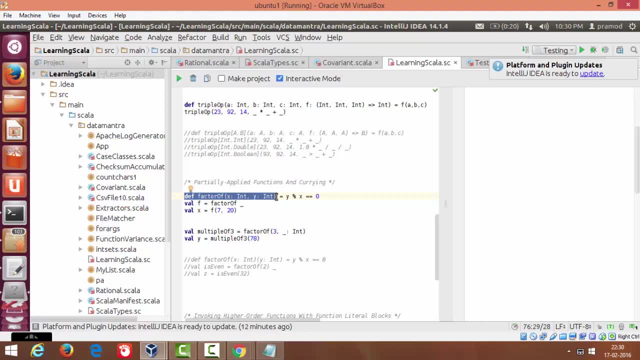 curry. So what we are doing here, factor of, is a function, simple function, and we are saying: whether x is a factor of y, whether x divides y and there is a 0 remainder, like 2 is a factor of 4, we have 5 is a factor of 25, 5 divides 25,. 10 is a factor of 100, means 10 divided. 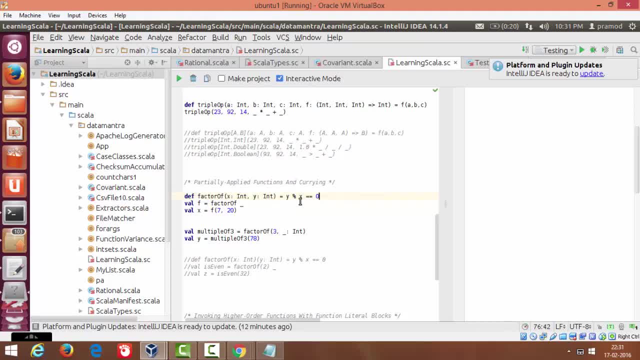 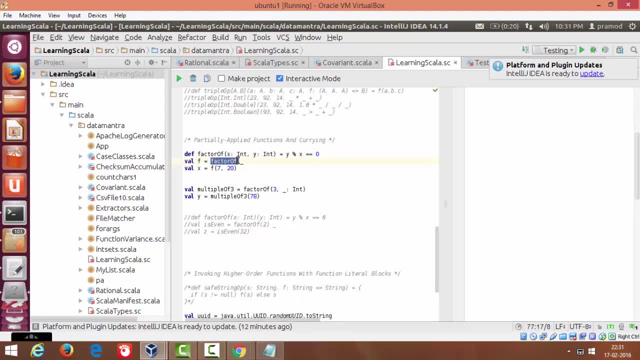 by 100. that is what we are checking with this function. So we can do in this way. as I said earlier, we call this function, but we do not pass the actual argument. instead, we pass underscore. it will return a function variable right. once it returns a function variable, we can pass the actual arguments. this is partially ordered. 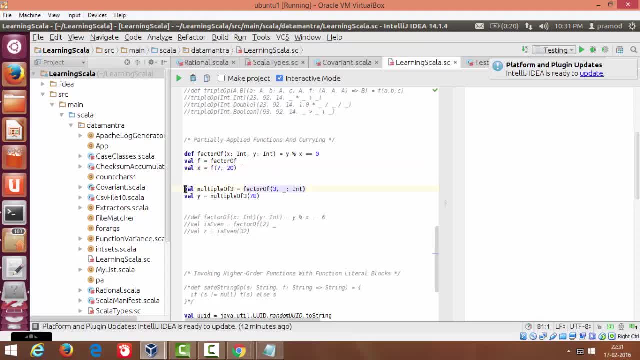 function. So we see how we can make use of that partially applied function and reuse some of the function. So we have a function that that is, gives a factor of 3.. So we can define in this way: we are passing factor of 3 and some function underscore. so 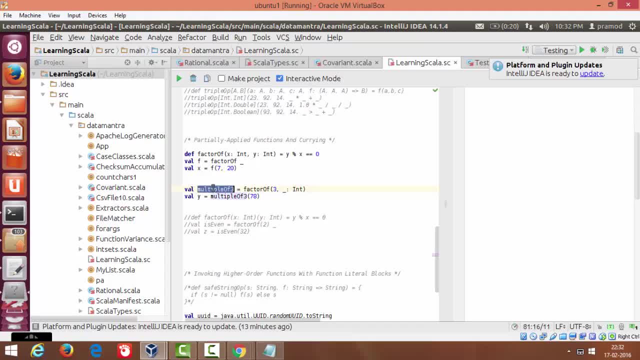 it will return a function variable and we can call it as a multiple of 3.. So this is like good to read. We are checking whether 78 is a multiple of 3. so this is how it could be used as a partially applied function: by passing underscore instead of having in this fashion, like saying whether. 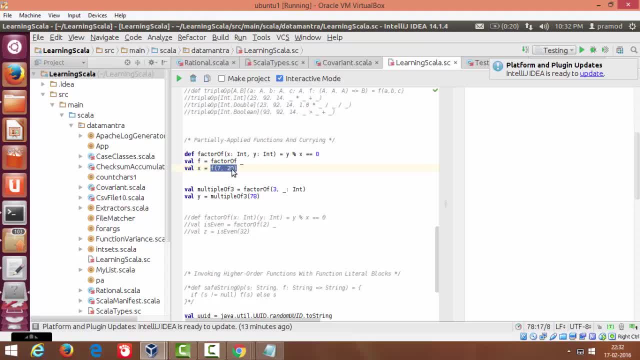 F is a Dany400.. whether 7 is a factor of 20, this doesn't look good, right? It doesn't give a readable format like what we are trying to do here. We can't say what we are trying to do here. 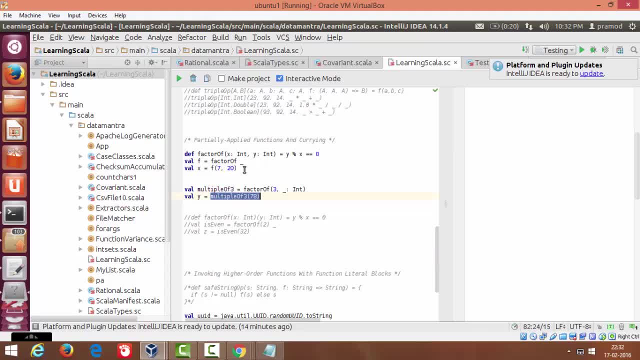 but this, this: this will show you what we are trying to do. It is more readable. So we are not passing a variable here, Instead of we are keeping it as a function variable and then we are passing when we call this function variable. So this makes more readable. 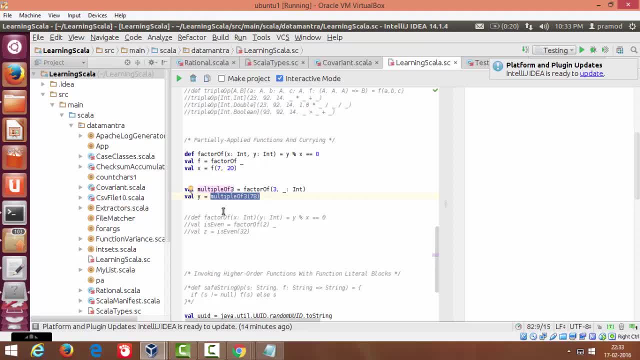 This is what this is, where partially applied functions are used, And also- we'll see more other examples- When we actually see spark. in that case, also, partially applied functions are used. Partially applied means we are holding back some of the parameters We are not giving. 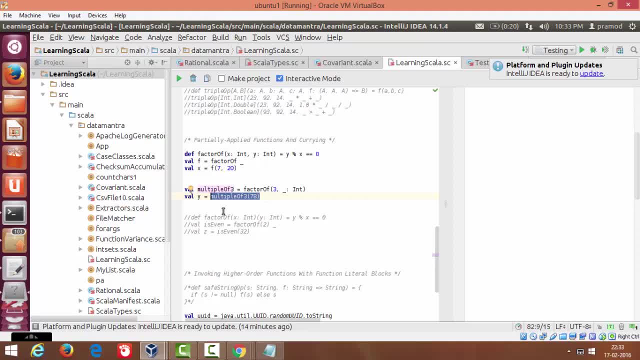 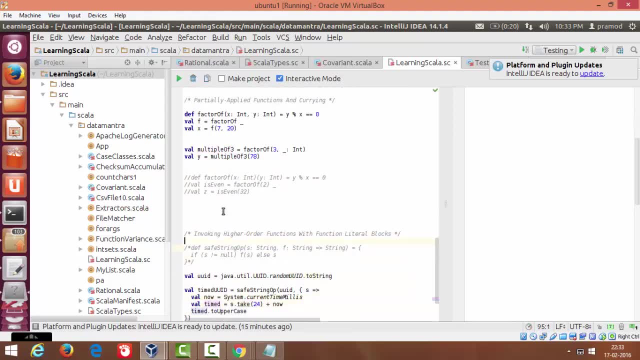 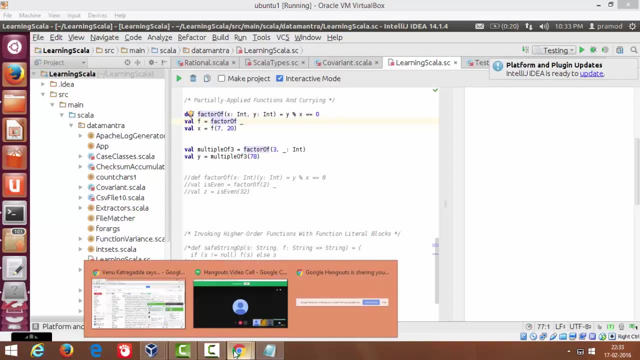 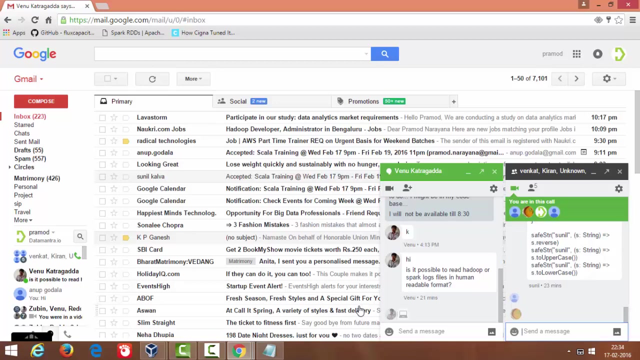 all the parameters. That's the reason it will be partially applied. Uh, any doubts here till now? or did I lose some of you? If you have questions, please do ask the questions. Okay, thanks a lot. Let me just sign off this here. 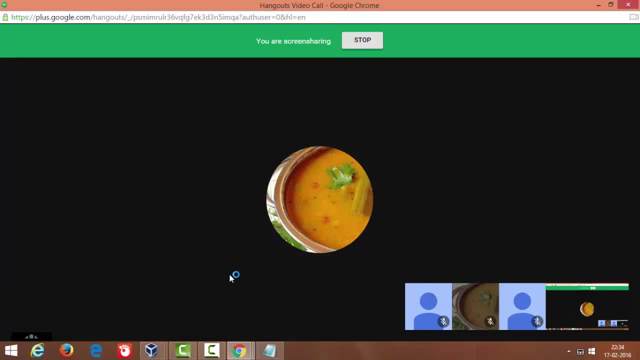 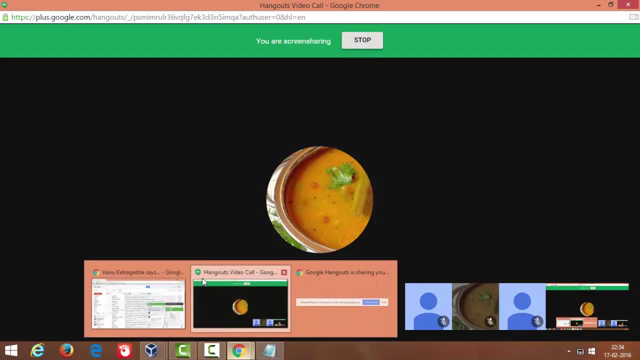 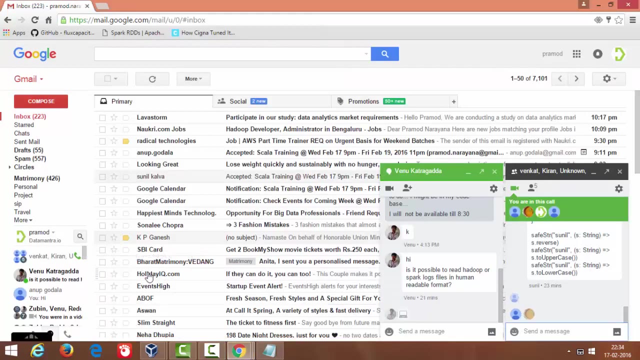 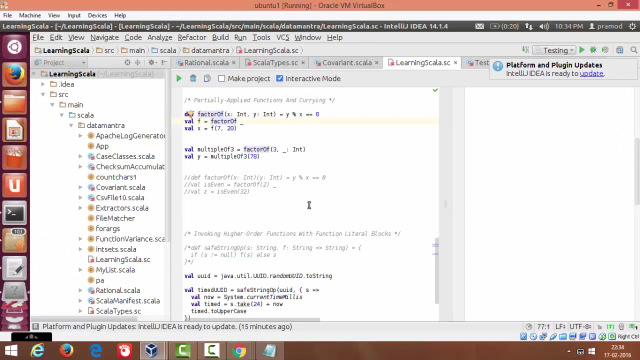 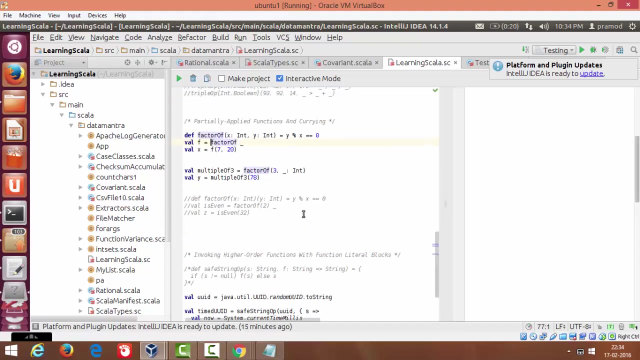 Okay, Silence. I assume everything is following. Everybody is following. Yeah, Okay, Okay, Silence. I assume everybody is following. Yeah, Okay, Okay, Silence, Okay, Yeah, here we last time. in all these example, the body of the function was just a simple. 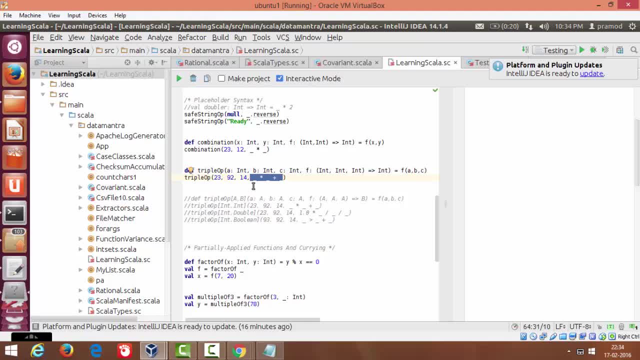 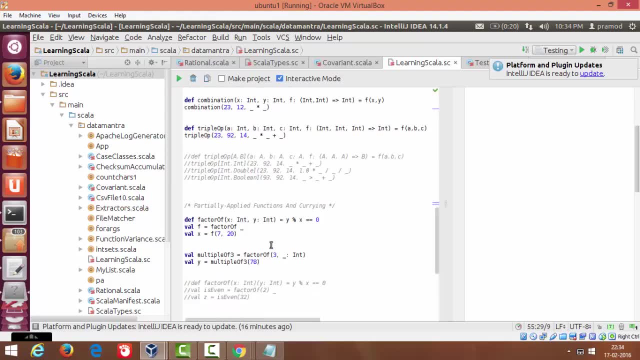 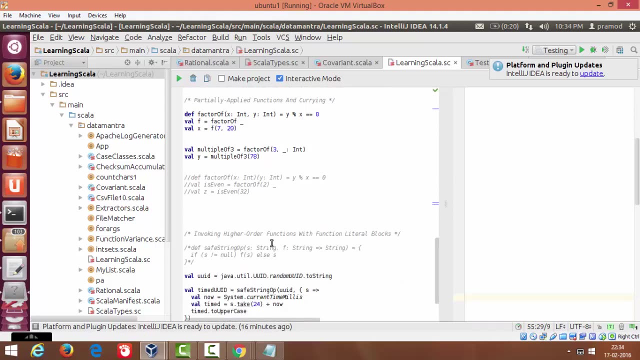 expression. we are doing multiplication, arithmetic, reverse, single, single expression, the body of the function. but we can have a body of the. usually the body of the function will be much, there will be lot of expressions. so it is called a block, function block, literal block. so if you are having such type of function, we can use this open flower bracket and close. 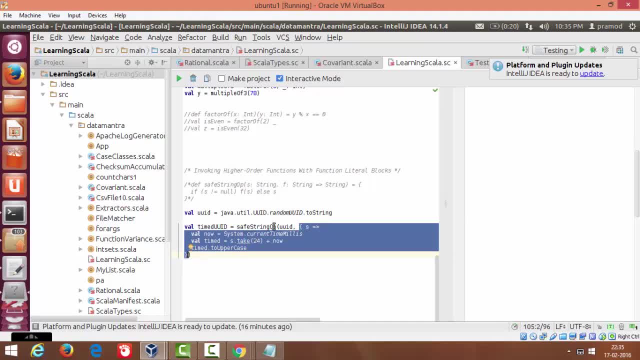 flower bracket. again, this is our same save string operation, which is a higher order function for which we are passing once. first parameter is a string and our second parameter is a function, actually a function. we are defining the function here itself and this is a much bigger function, not just a simple expression, so you can define in this way also. this is: 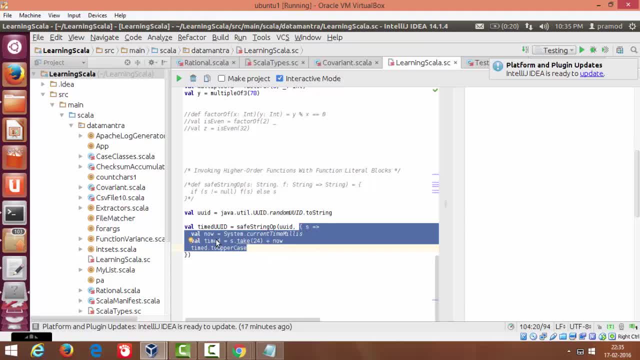 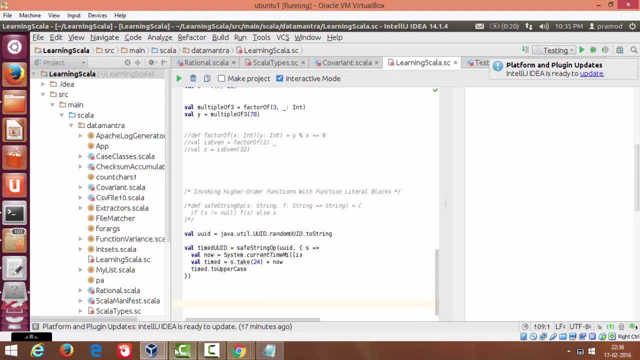 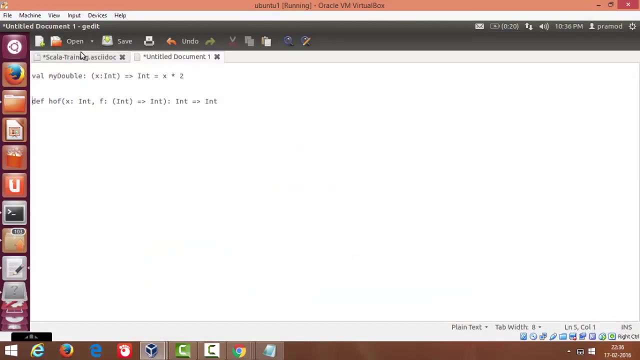 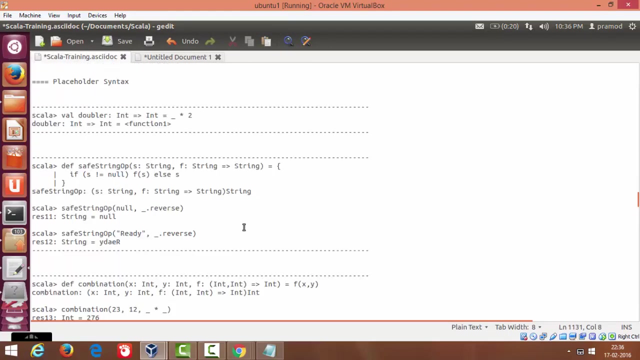 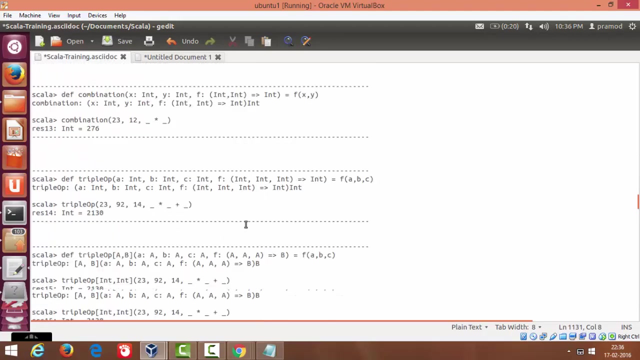 called literal block. the whole block of the function is written here itself. so we would call unit based on the function. the column is in a state two. so let us see the Fat Factor. Let's go by capital letter, k, evolution, Then we will get a one over the一个, one over a video, and then if we use view или 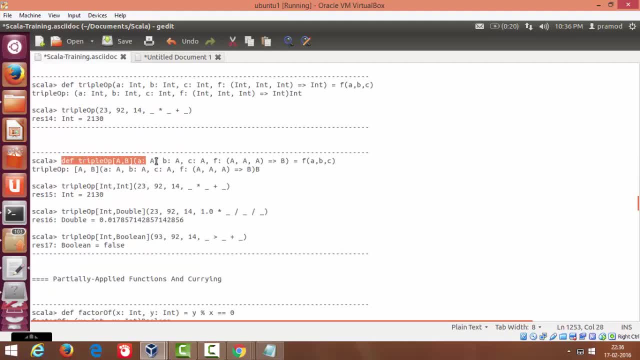 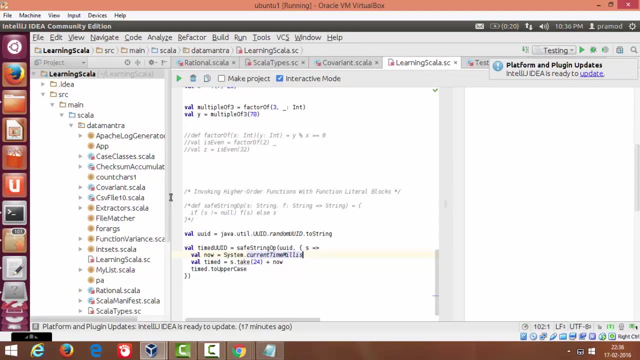 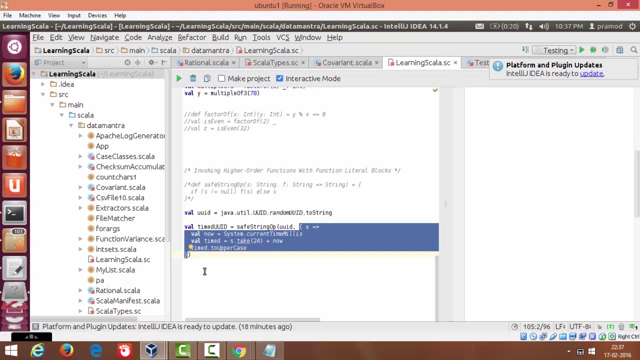 view the max and those become auto in our state: two, two, three, four, and then you see one more for generic data typing. so this is the same example: triple operation, show saw for which one keep operation. okay, this is the body of the function directly being passed. 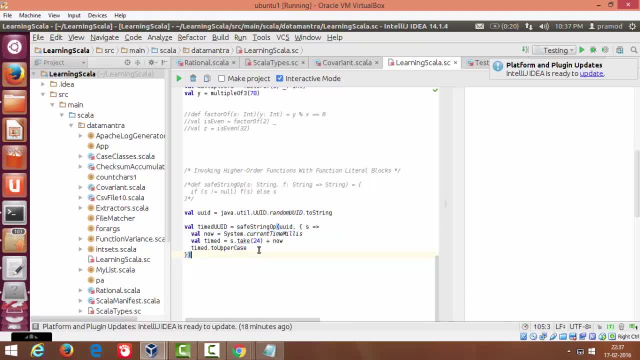 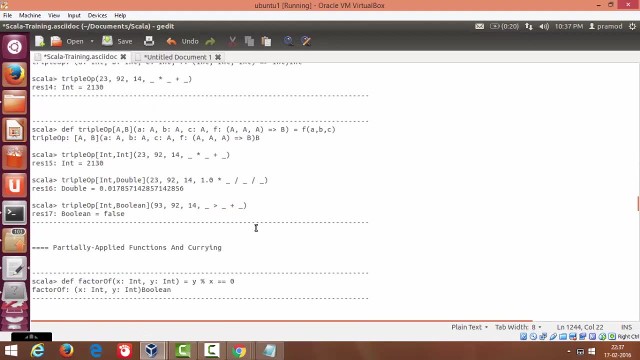 and this will be the last. this is the last statement of that function, which is again a. the return type is string. here is what we discussed earlier. like generic data type, we have triple of a, triple of B, a comma B are the generic data type. it can hold any data type. so 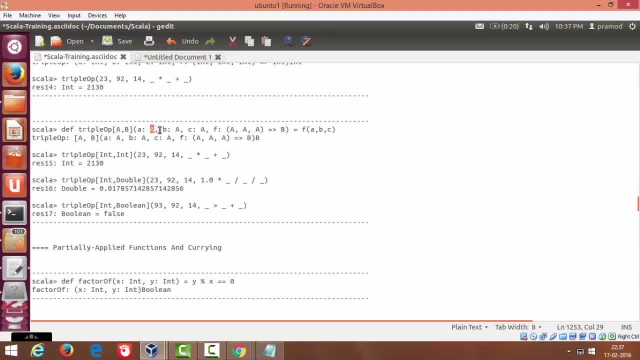 the first parameter is a of the type a. second parameter is again of the type a. third parameter is again of the type a. then we have a function variable which takes three parameters of type a and its return type is B. so that's the reason that the type parameter of this higher-order function is a comma. B means it takes two. 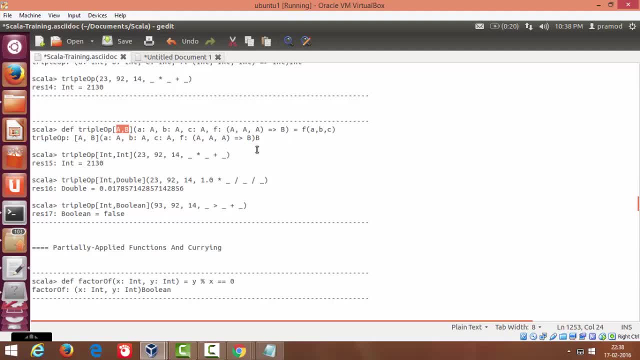 different data types. so to this we can pass any function, any definition. so if you see we are saying it as int, comma, int. only when we do star and plus operation, the return type of this will be int itself. so that's the reason a is also int and B is also int. 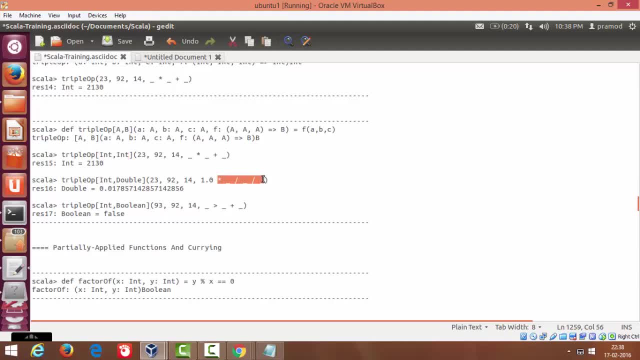 but when we have division kind of operators we will return a double. so that's like 2 divided by 3 will be a double right. so that's the reason the first parameter is type parameter is int and second type parameters double. again, these things are not mandatory, it will be inferred. 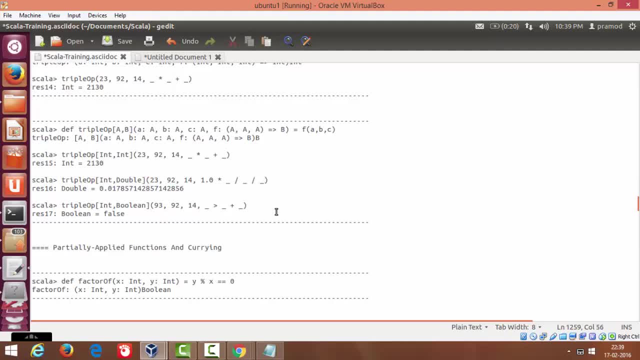 based on what operation you are doing here. similarly, what we are doing here is the definition. sees, if you see the definition, we are doing second parameter plus the third parameter and once we get the result of that, we are comparing whether the 0th parameter is greater than first parameter. so, based on the 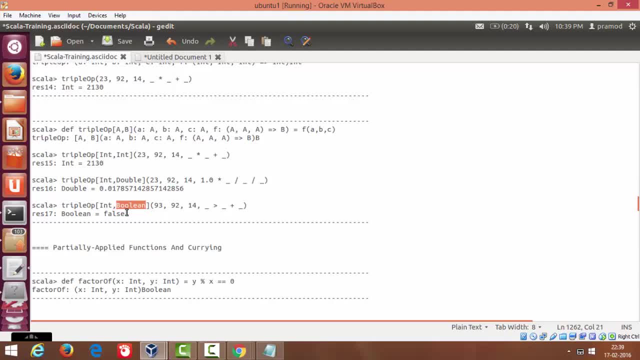 evaluation. it will return Boolean, so the data type is int. type parameters are intent Boolean. so the same triple operation has been used for different data types plus the higher-order functions. so this is a triple operation, is a generic higher-order function. it can work on different data types based on the what, what operation you are. 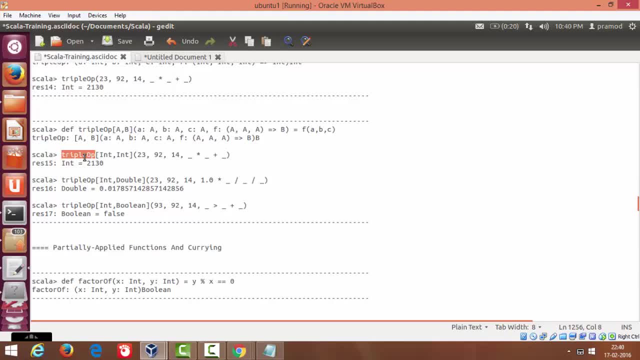 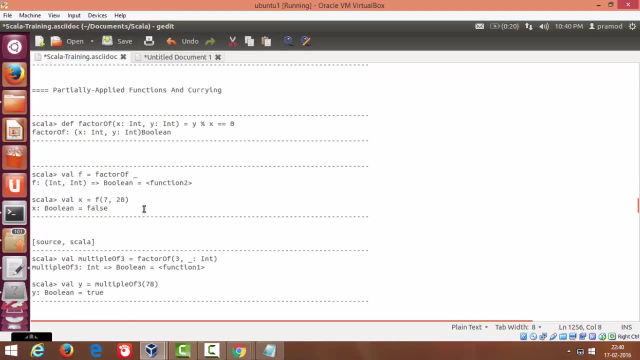 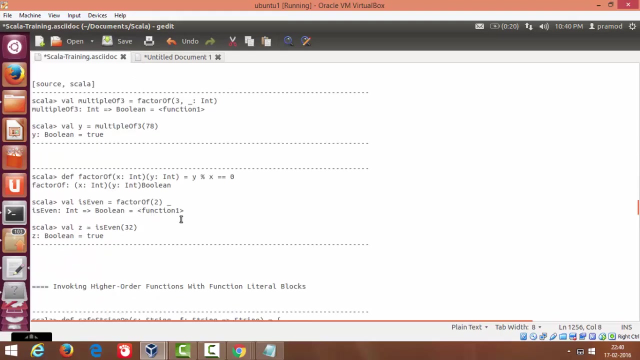 performing what is your itself. so if you see again, one more example is there which gives a carrying example. so this is what we saw occurring multiple of three. so this means again that when to code a particle 1, So we have two parameters, factor of x, factor of group. two parameter list, x, comma, y and 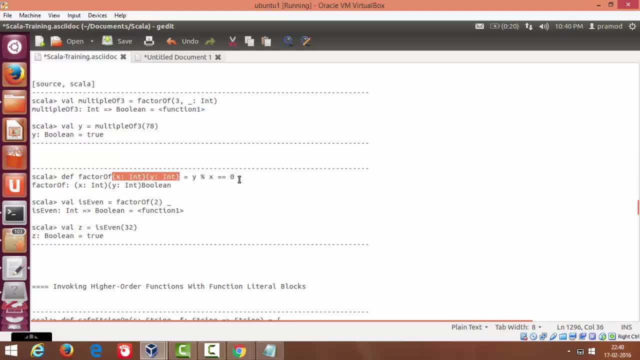 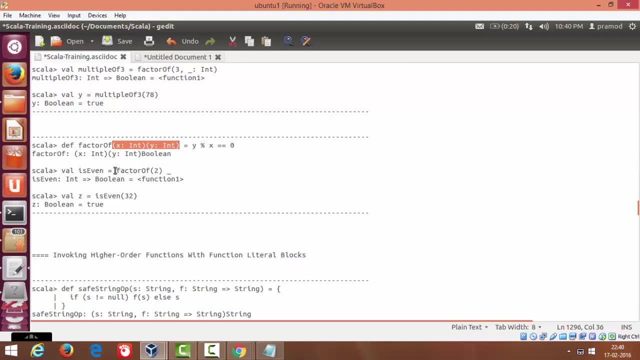 we are checking whether x percentage y is equal to 0. That is nothing. but we are checking whether, if x is a factor of y, like 2 is a factor of 4,, 5 is a factor of 10, 10 is a factor of 20, such kind of things. 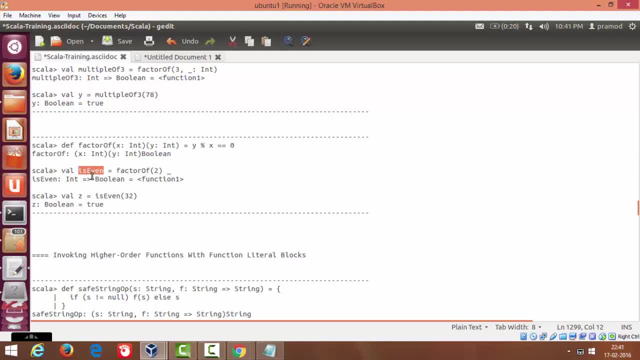 So we can define a function variable is even and we can call factor of 2 and then pass an underscore. what it will return is a function variable is even. is a function variable we can call later, So this becomes more readable now is even 32. instead of giving means, we are reusing. 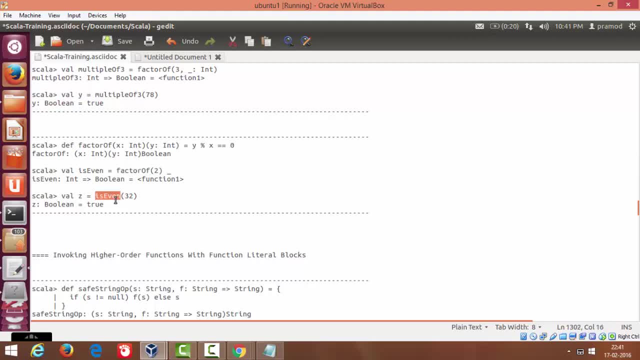 this factor of 2.. So we can write a function to get an even number function. So that is what makes it curing. it is be used for reusability and a better reading function. I hope you got yes. Curring with grouping. curing is nothing but passing multiple parameter groups. 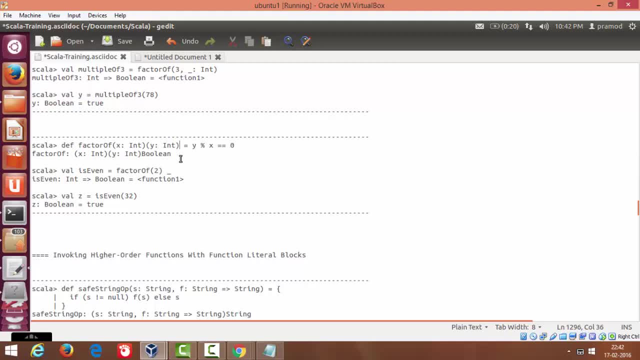 yeah, yeah, that is also good enough, but this is also one way of doing it, and we have some more examples on this, not just this. we need not specify this parameter at all. we can say this as an implicit parameter. we will see when we see implicit parameters. so in that case, it. 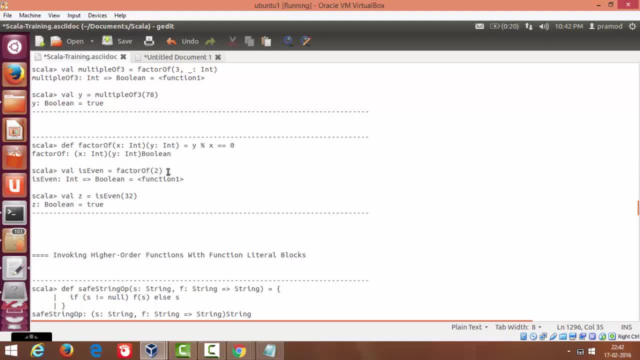 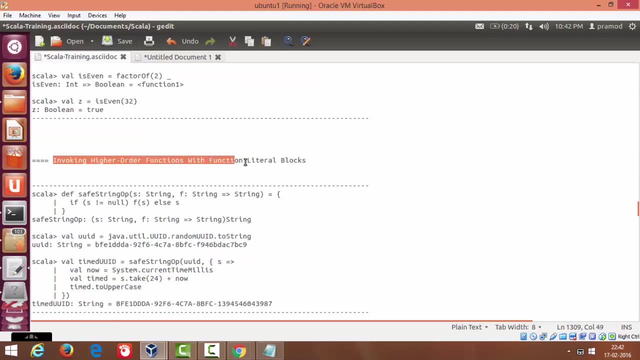 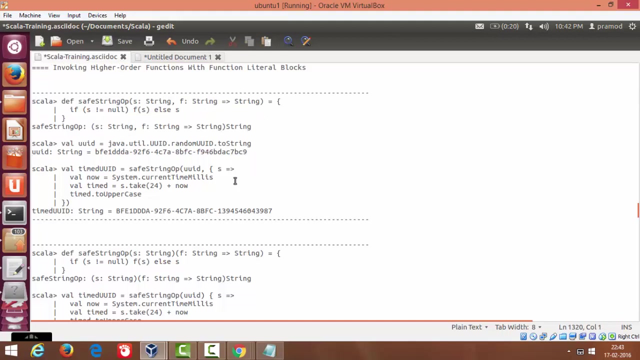 will be much more clear. you don't have to pass anything at all. by implicitly, the compiler will pass one of the parameters we saw invoking higher-order functions with function literal blocks. this is what we saw. we can specify the literal in the body itself. sorry, as a definition, we can specify a function. 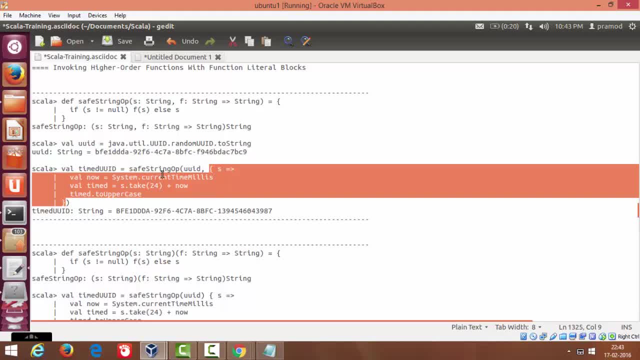 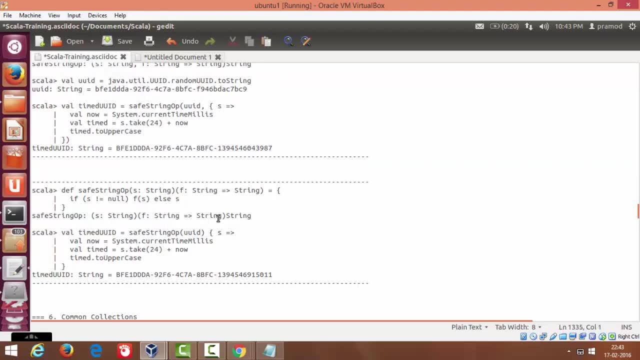 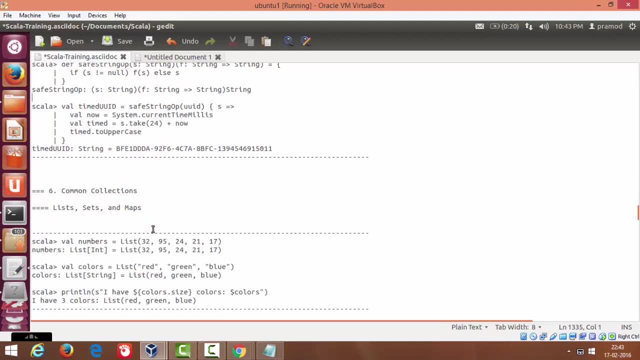 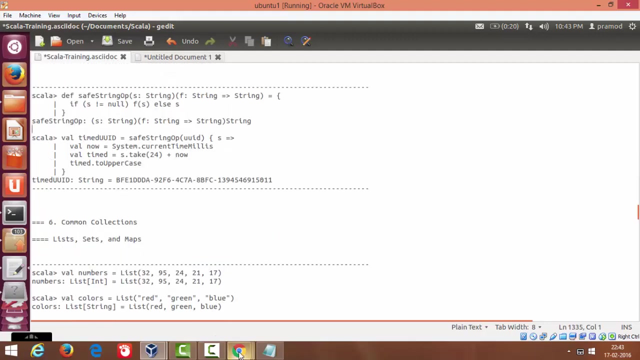 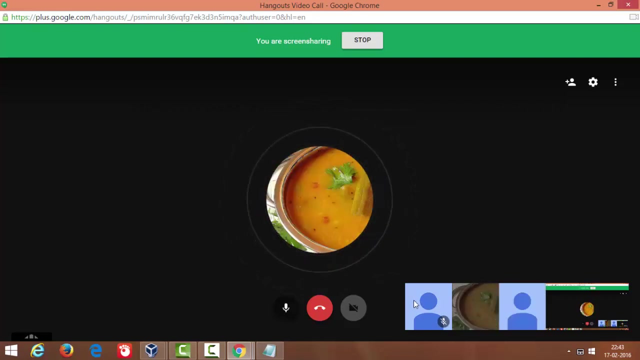 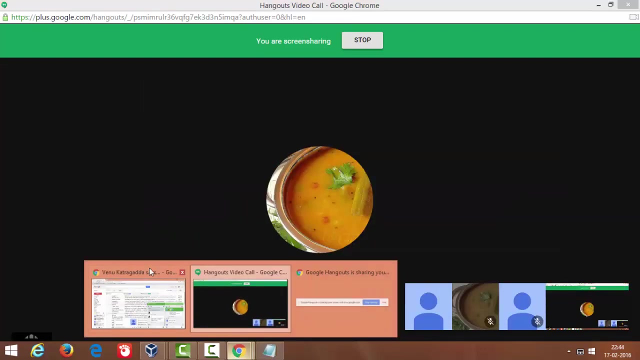 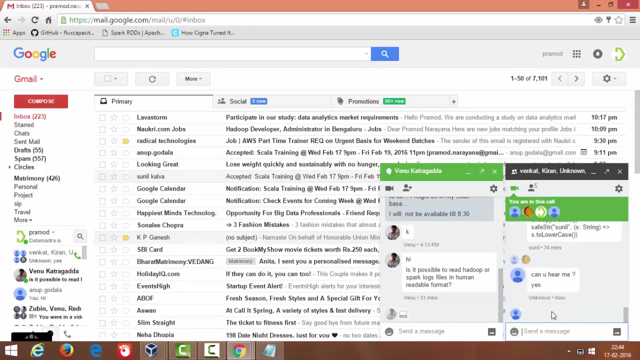 literal body to the higher-order function. these are. these two are the same example. so shall we go ahead with collections or shall we stop here? hello, hello everybody. fine with collections. okay, I know that I can't hear you. okay, yes, we can continue again. no, I can't hear you. okay, yes, we can continue. 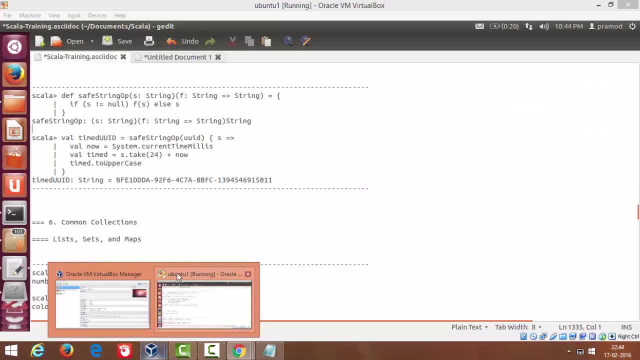 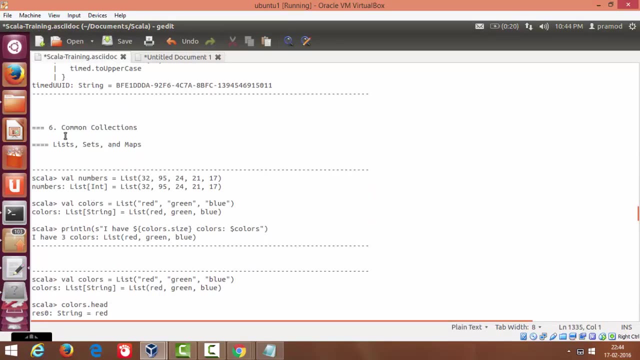 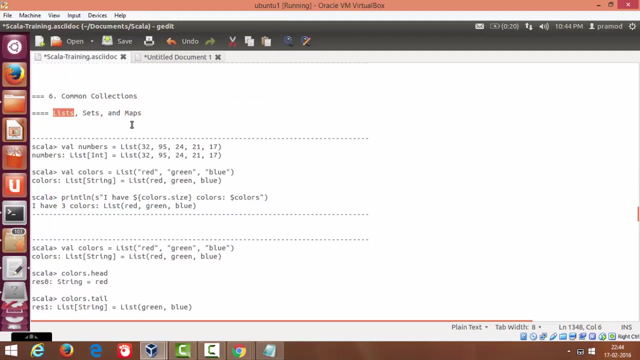 okay, no, I can't hear you. okay, yes, we can continue. So next we have common collections: lists, sets, maps are the sequences. usually we say: are the common collection? sequences, sets and maps different, are categorized under different things. we can say sequences here, sequences, sets and maps. list is a subset of sequence. 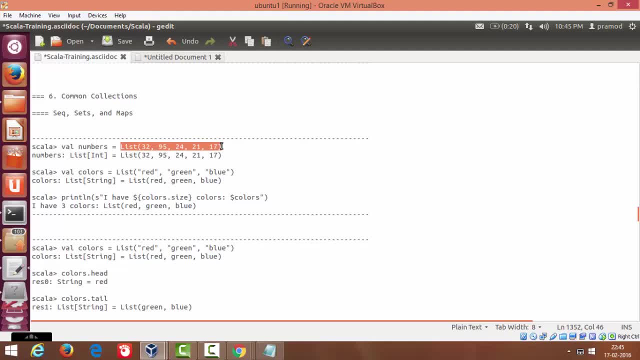 so list is one of our collection and most of the till now we saw how the higher order functions were called. so, on collections, by default collections are immutable. that is what I said from the starting. Scala is immutable means the default collections are immutable. List is an immutable, so most of the higher order functions are methods of the collections. 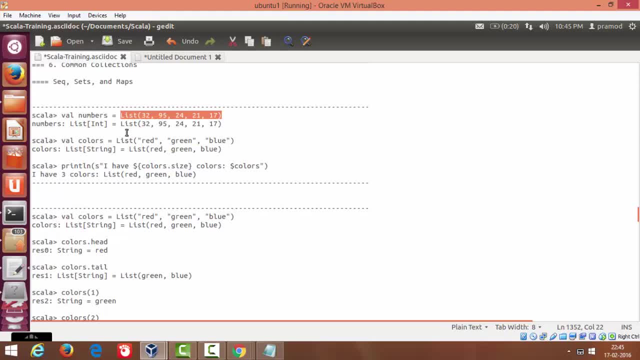 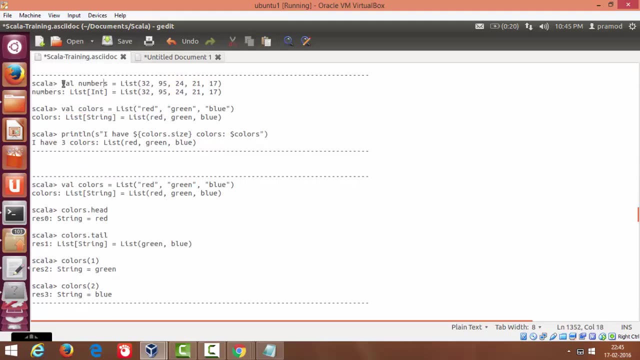 so will see how those work. actually we will start using higher order functions. on collections, this is normal list. here data type is inferred automatically. we see it has inferred it as a list of integer. when we give list of red, green, blue, it says is a list of string, the. 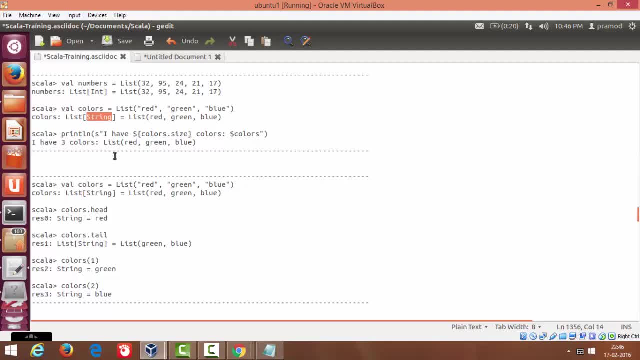 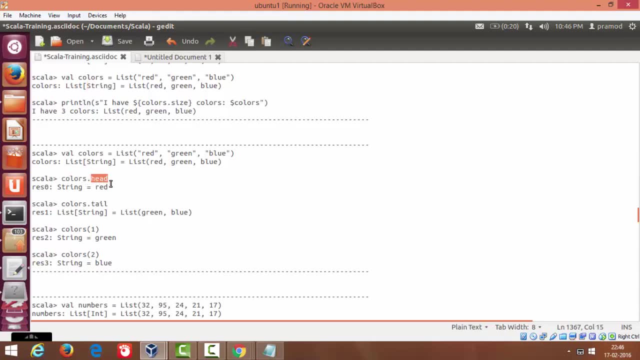 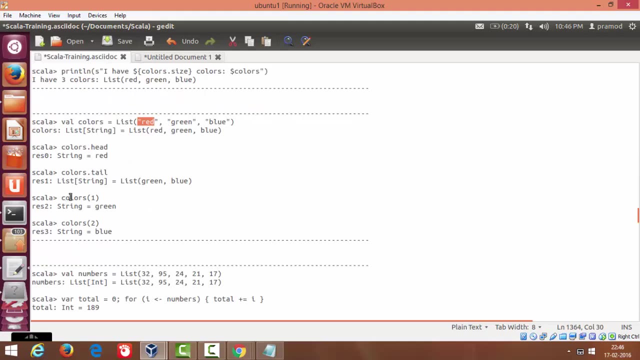 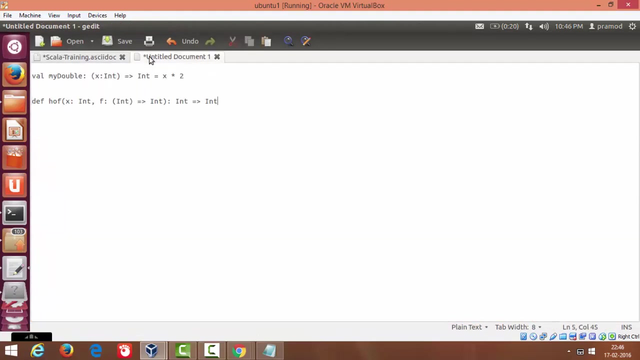 compiler automatically inferred the data type for you. so these are the simple operations on list. head will give you the first element in the in the collection list. the tail will give you the rest of the elements as a collection. so the way it is implemented- list is implemented internally- is we have first: 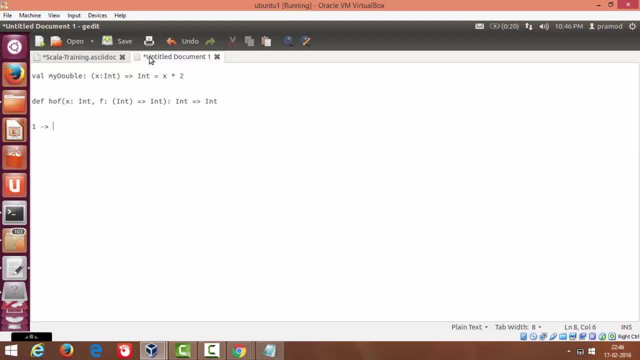 element. then we have a pointer kind of to the second element. this is how it is implemented as a singular linked list. one second lab you. yeah, this is how a list is implemented as a single team list. so whenever we do, whenever we call colors dot head, the first element is written. whenever we do. 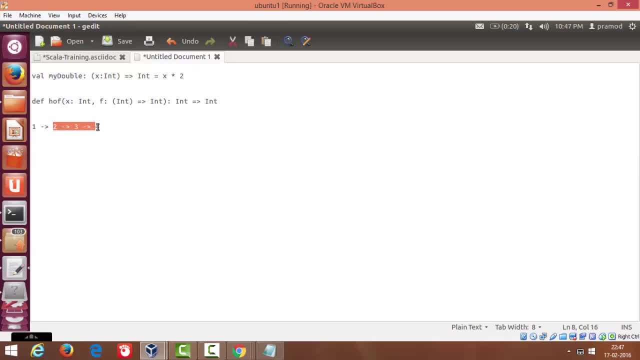 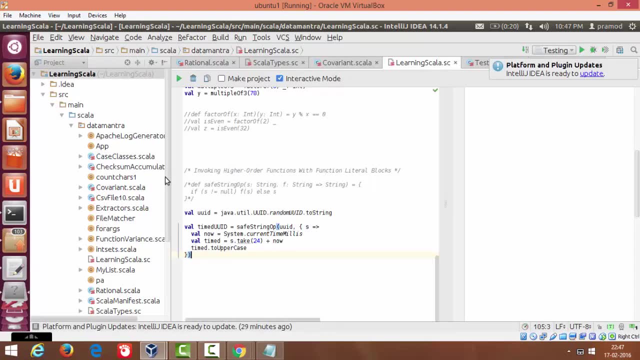 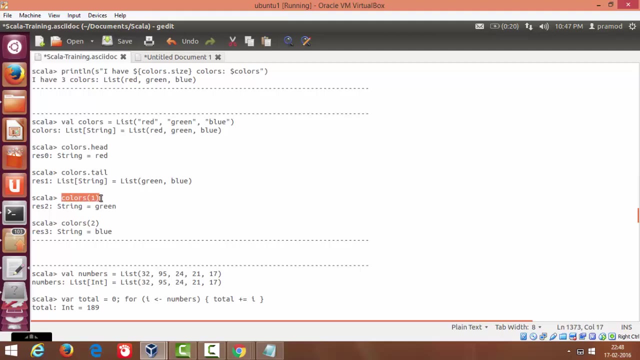 The list dot tail. rest of the elements will be returned as a collection, again as a list here. So this: You can access The elements of the func of the list using open bracket and close bracket. usually we access the list with Square brackets, but if you, if you have paid some attention. 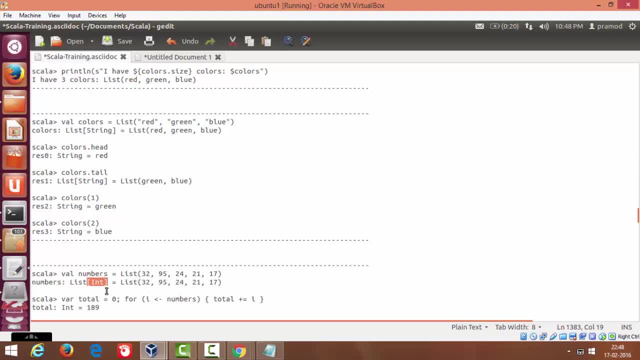 The square brackets is always used for data types, to specify the data types here. open bracket and close bracket is used to access the elements of the function and in fact it is. There is an apply method in the list That function is called actually here It is not a direct. 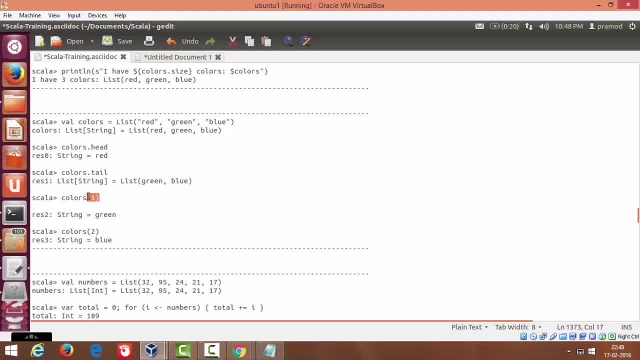 access as an index, but apply method is called, so always an apply method can be Ignored. while calling that function, you need not specify the apply. This is actually colors dot apply one. This function is called, but you can always keep writing this function in Scala. 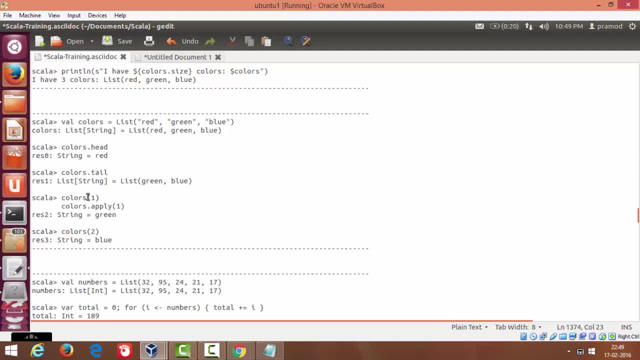 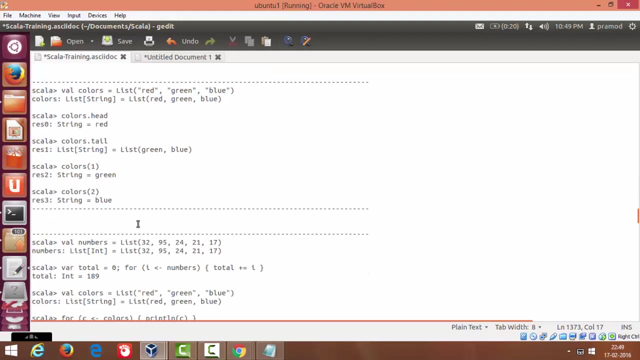 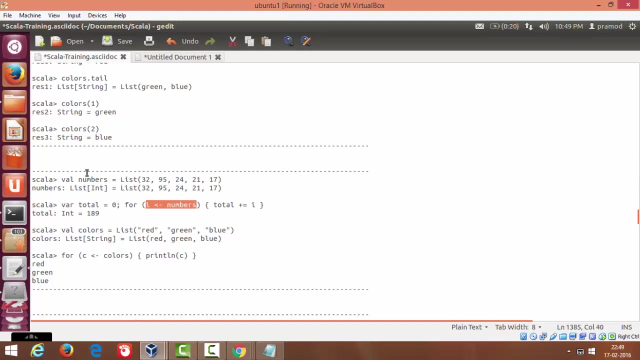 This is not a syntax. This is not like operator Indexing. actually this is a function being called on colors. object: colors is a collection here. Yeah, we can loop on the collections. We saw that for comprehensions. we need an iterator on the right hand side. 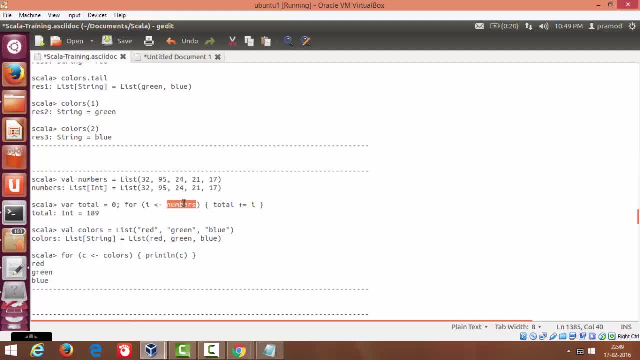 So the iterator is nothing but our collection. So it will iterate and generate the variables and it will be stored here and this is the result we are getting. We are just adding all the data in the list. This is simple for comprehension. Similarly, we have for comprehension: 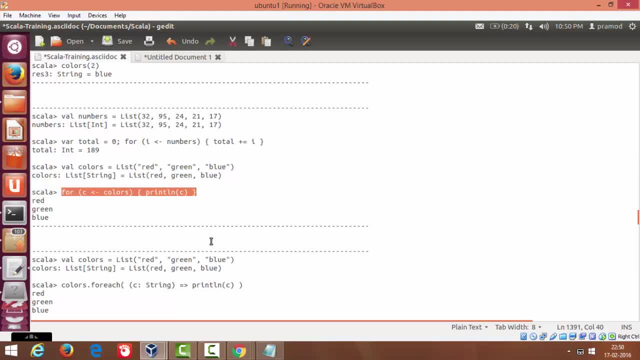 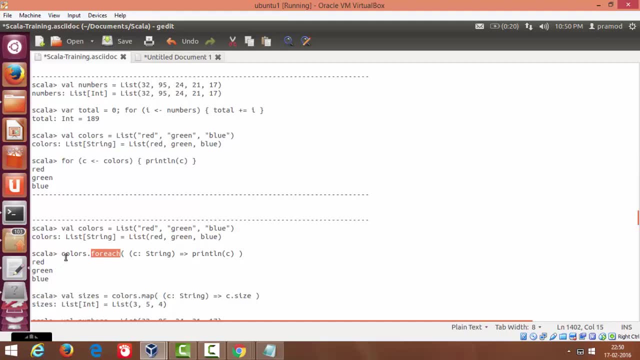 and printing the data For each is again a higher order function which is written on the collection The data type of the function. higher order function means it has to take a function as a parameter or written as a function, But in this case we are taking function. 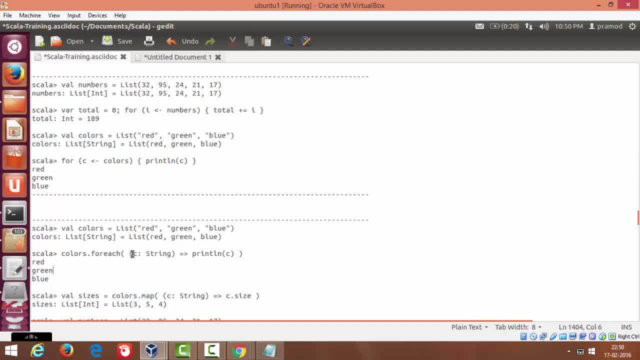 as a parameter. So we are taking function as a parameter. So we are taking function as a parameter And that function takes any data type based on the collection and returns a unit For each, always take some data type as an input and returns unit as the return type. That. 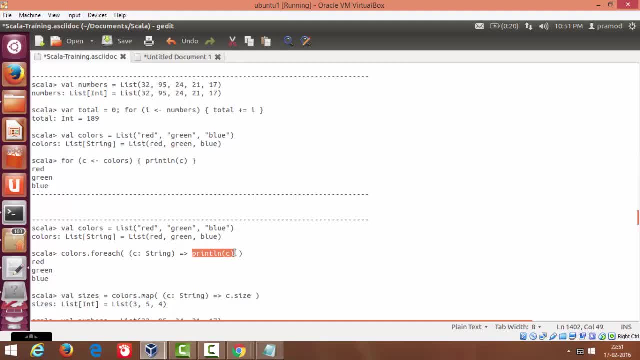 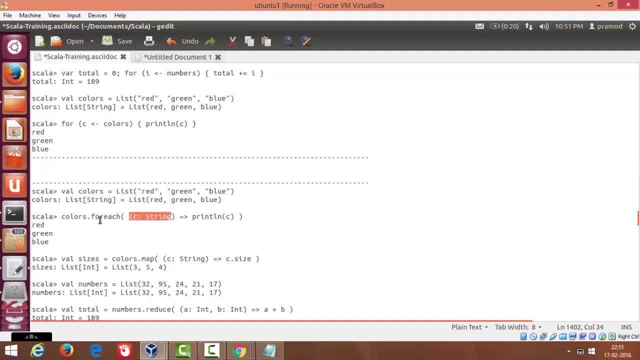 is the for each syntax. If you see, here it is taking this function as a parameter and this higher order function is being called on the colors collection And for each value of the collection we are printing the value. That is what we are doing. So map also What? 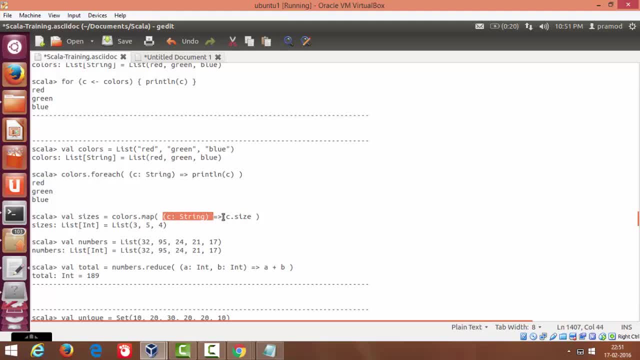 is map, It also takes a. So map also. What is map? It also takes a. It is also a higher order function. Higher order function here in the sense it takes a function as a parameter And that function takes some data as an argument. and it is like: 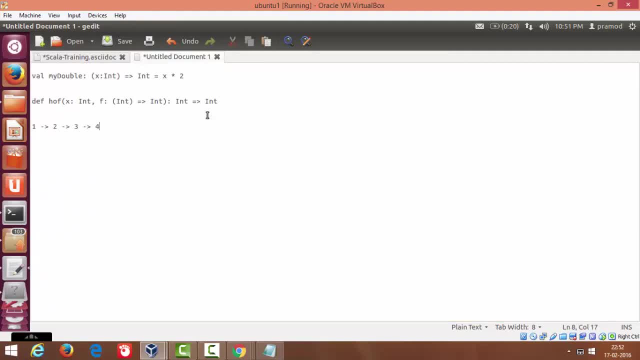 map is a transformer. It transforms. If you have seen, If you have learnt about set theory in mathematics, you will have set one, then f of x and then the next set. How do I say that If we had a blackboard, that would have been good One second. 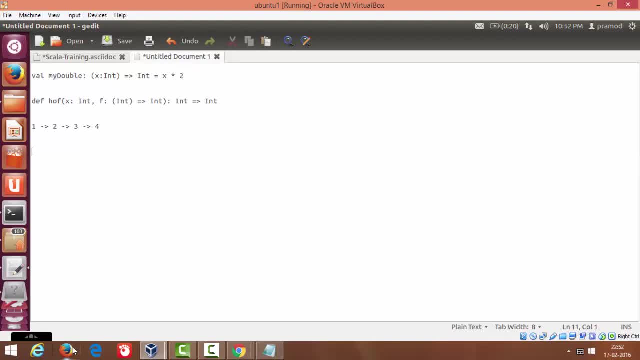 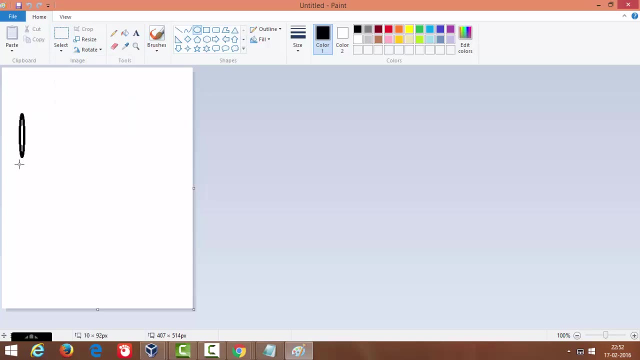 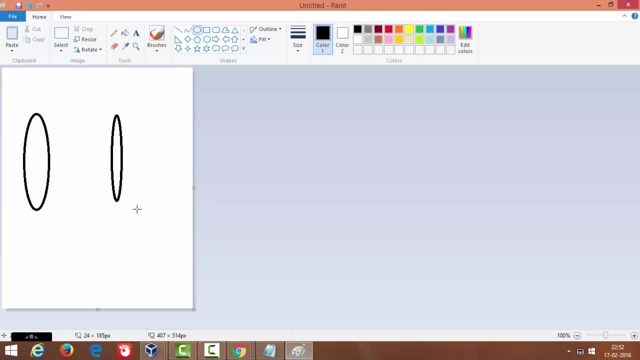 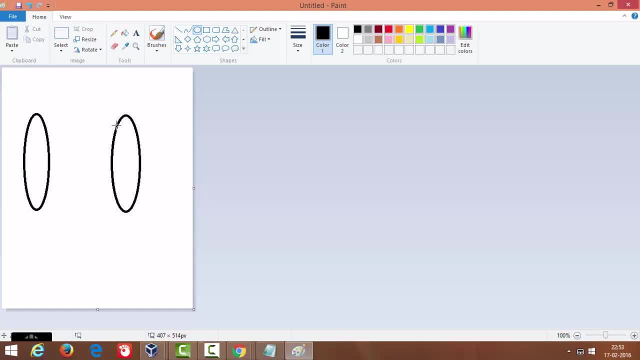 takes each element in this collection and transform into some other value in the collection. so that is what we defined in the set theory. in mathematics, like f of X based on what is the definition of f of X map is similar to that. it it works on a collection and transform each element from the source. 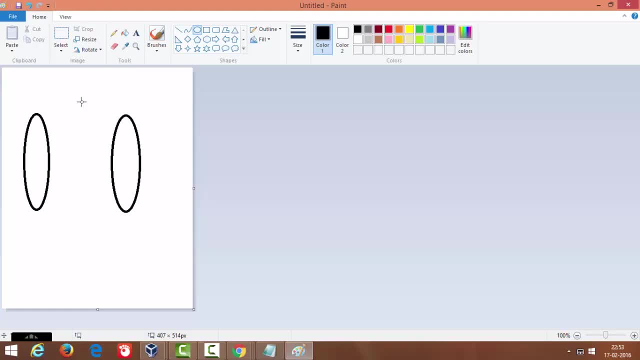 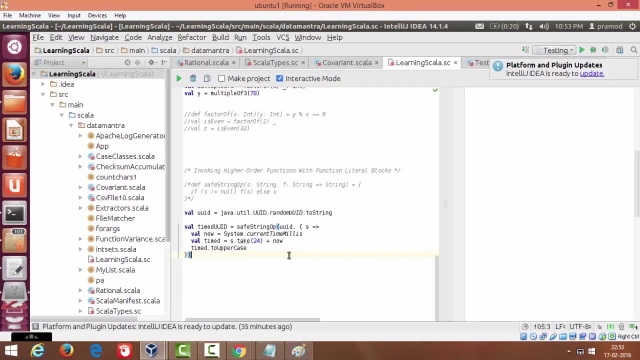 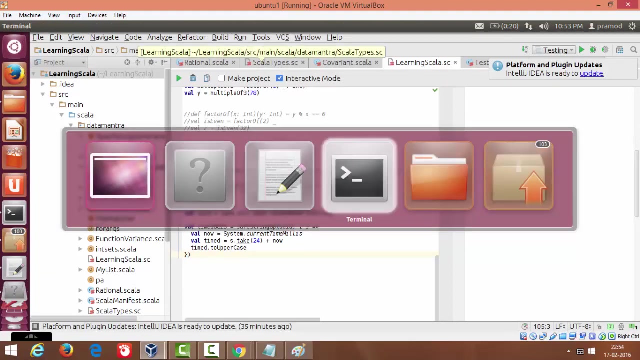 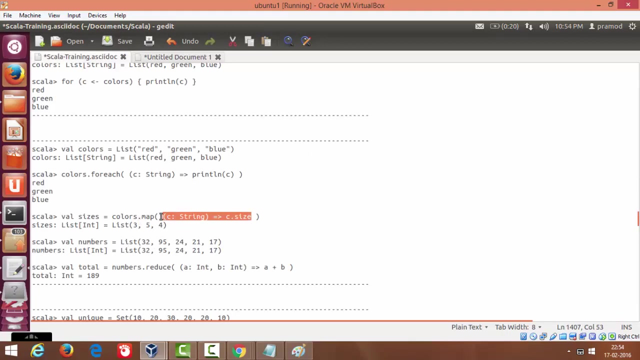 collection into some other, some other value element in the other collection means it returns a collection. the only difference between for each and map is for each takes it. it works on each element of a collection and returns nothing. but a map works on each collection and returns a collection, and we transform. 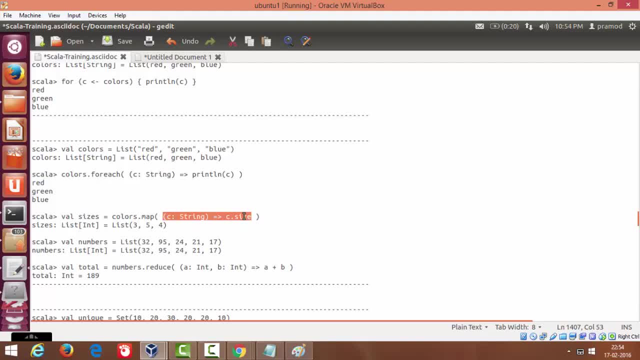 each element of the source collection into some other element. what we are transforming here? we are taking c dot string. what is colors? for each element of the colors we are providing the size of the color, so it returns a list. it takes a collection and returns a collection. that's what is map and the difference between. 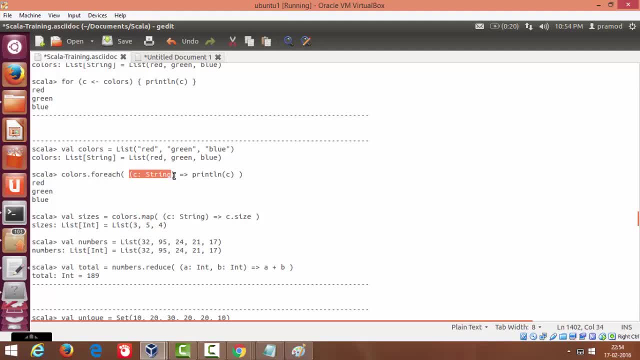 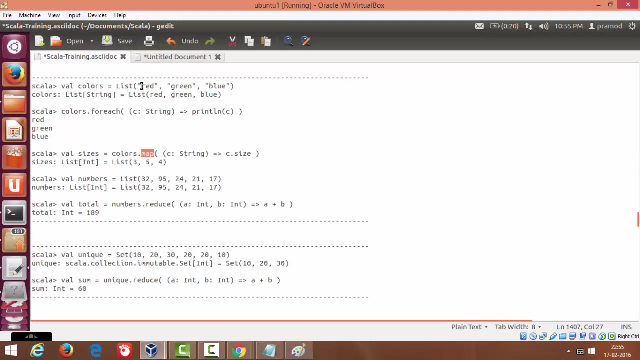 for each. and map is: it takes a collection- iterator in the sense- and returns nothing. it returns unit. void means unit. the map is: takes a collection, returns a collection, but transforms each element in one collection to some other element in the other collection. that's what we are transforming for each, for comprehension. 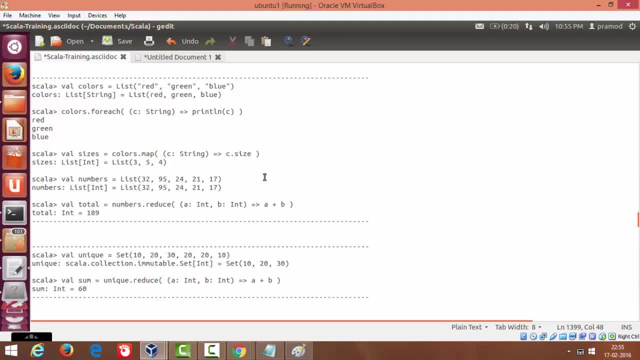 for comprehension- Yeah, that's what I was saying, For comprehension is not a simple for loop in any other language. Internally, it is implemented using these maps and filters- higher order functions. That's the reason we can do it the same thing with the for comprehension and yield, because internally, 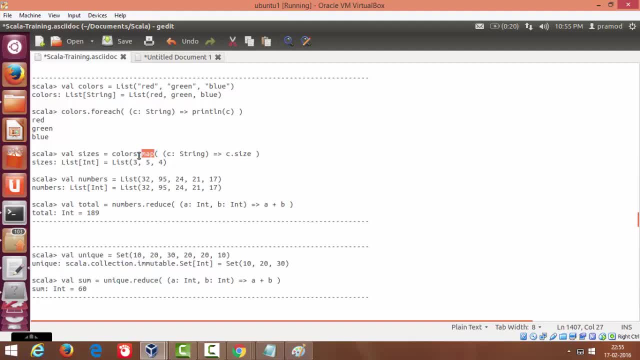 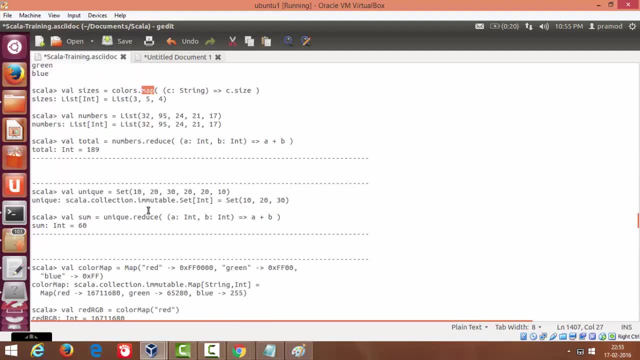 it is the same thing. map filters are being used to implement the for comprehension. Yeah, similar as we have map, similar to the, to that we have reduce. What reduce takes is a. reduce is again a higher order function which has to take a function as the parameter. 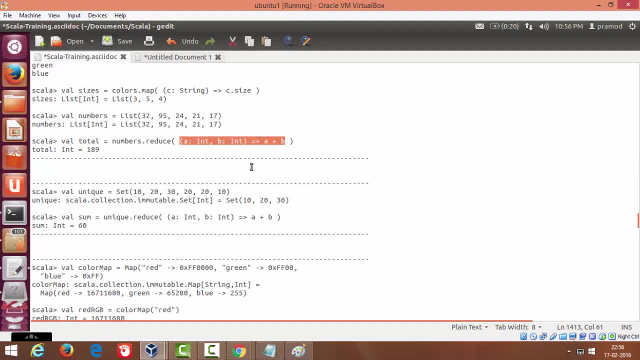 This is the function to the higher order function. What that function takes is it takes two arguments and returns. here the definition is we are adding those arguments. So what reduce does is it takes a collection and returns a single element from that collection. It reduces all the elements of the collection into a single. 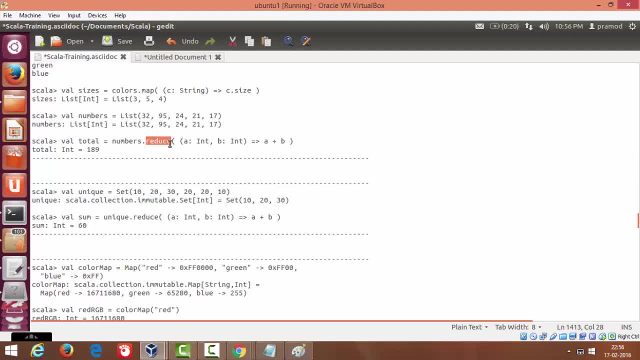 value and that value is returned here. So what actually happens is this: the first argument is called as can be called as an accumulator, and the second argument can be called as a iterator. So the accumulator will be initialized with the first value of the list, Here numbers. 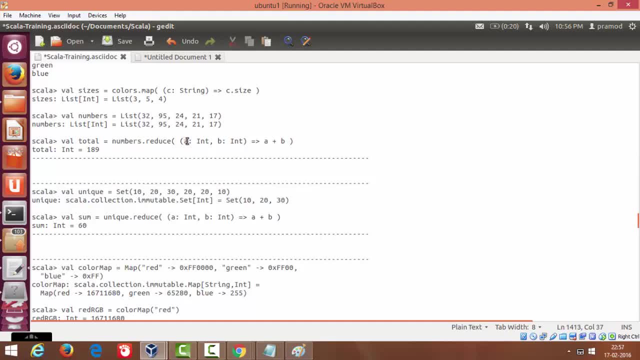 is the list Accumulator will be assigned, initialized with the first value of the list, and B is a iterator on the list, So B will be starting from the second value of the list. So what it does is it adds first and the second value and since A is the accumulator, the result will be accumulated in the first. 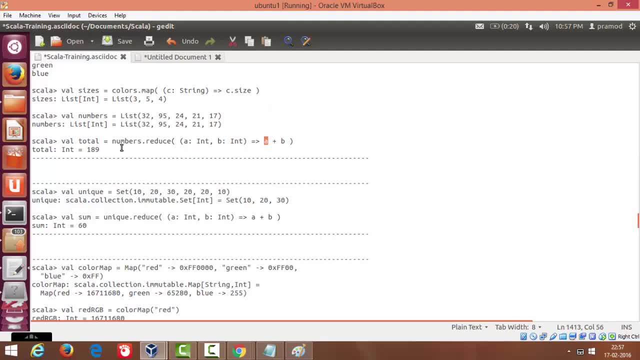 parameter, and this will go on till it does a plus here. First it will calculate 32 plus 95. And the result will be stored in A accumulator. Now B will iterate from 95 to 24.. Now 24 and the previous accumulated. 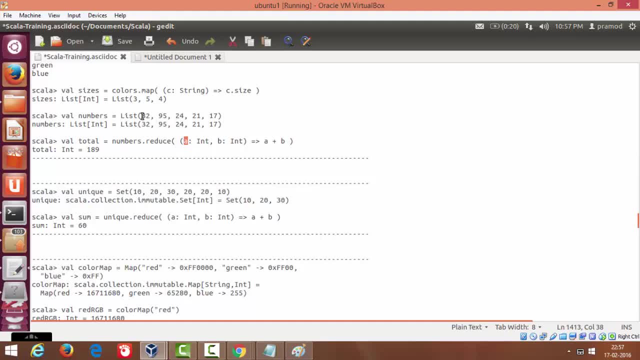 value will be added 24 plus the result of these two. So and it will go on till the whole elements in the list are done. So reduce takes in two parameters as arguments and returns a single element. Reduce: the name itself says that take something as a collection and reduce it to single element. 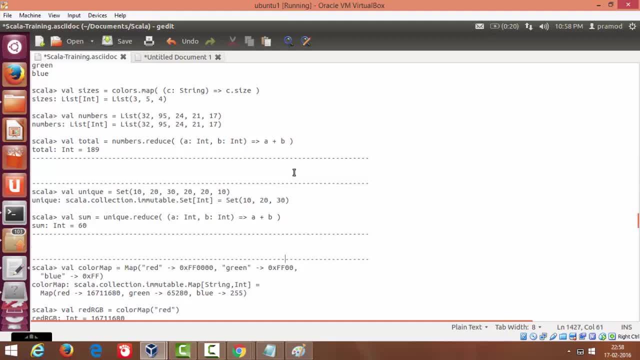 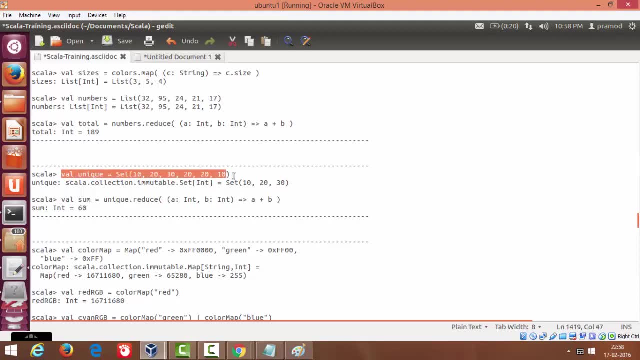 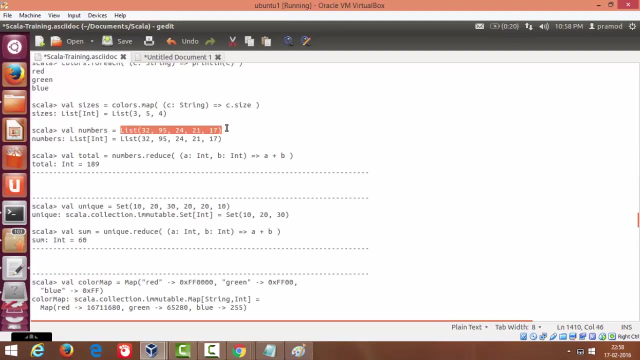 That's what is all about reduce. Next, we have set. Set is nothing, but it is also a collection. but it has unique values And also it is not Ordered collection. Like list is a ordered collection, It means you can access it by indexing. We saw, we accessed. 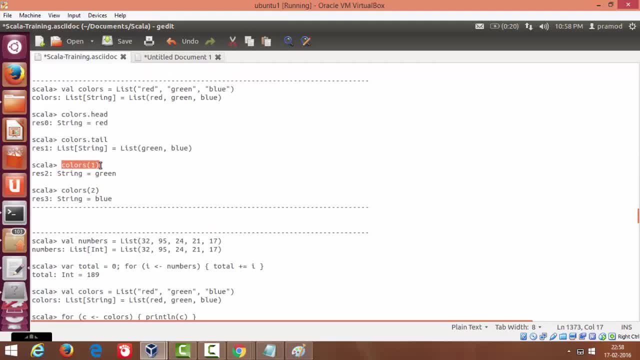 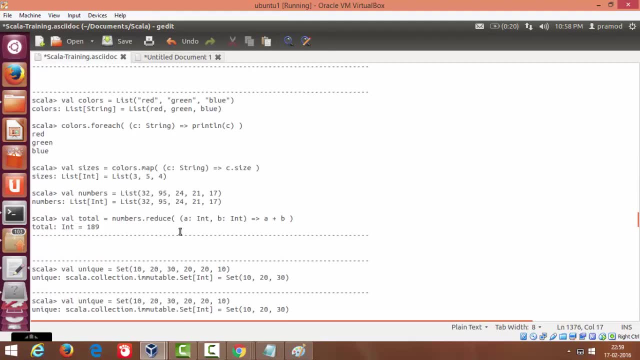 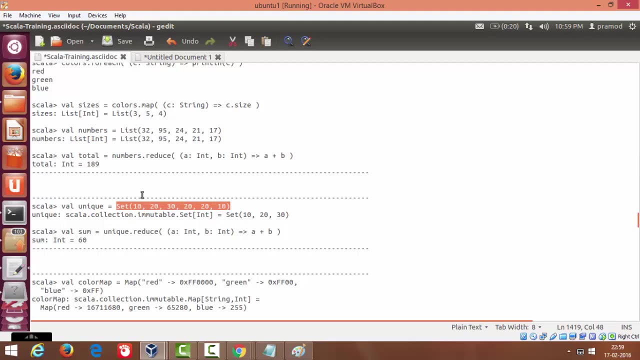 it by like indexing. Colours of zero, colours of two. it means list is an ordered collection, but set is not a ordered collection. You cannot access it by indexing. it has like contains is exist kind of function, not an accessing by index. that's because it is an unordered collection and also all the elements. 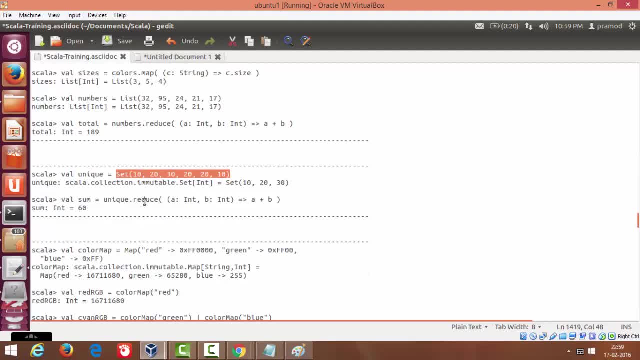 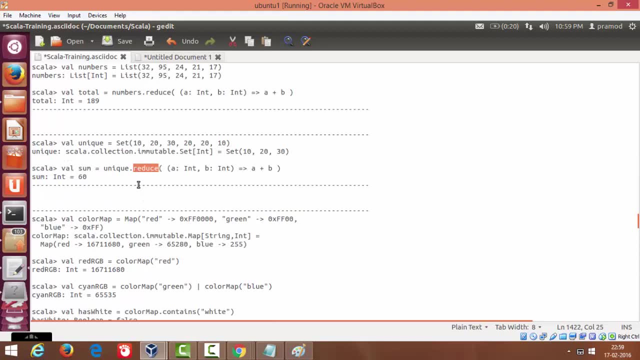 are distinct elements in the set. that's the property of a set. we can have all the same higher order function, some of the higher order function defined on set. so now most of the higher order functions are defined on the collections. first we saw functions, then we saw function. 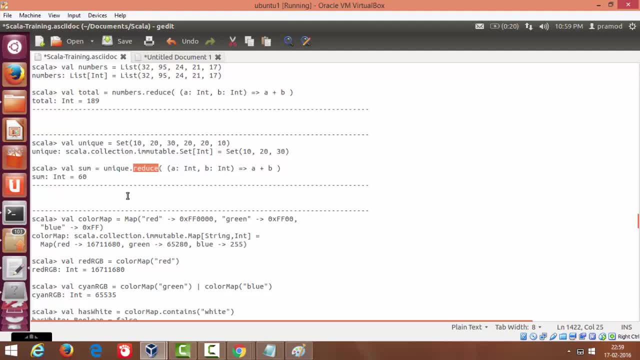 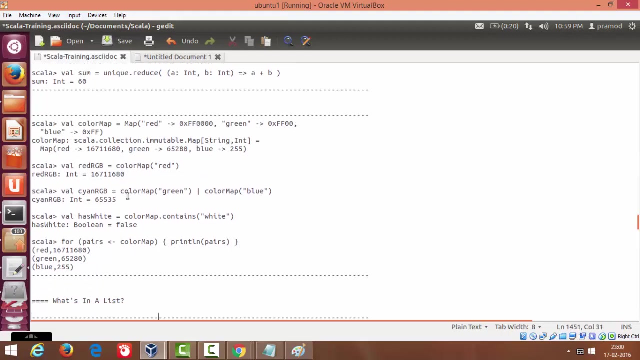 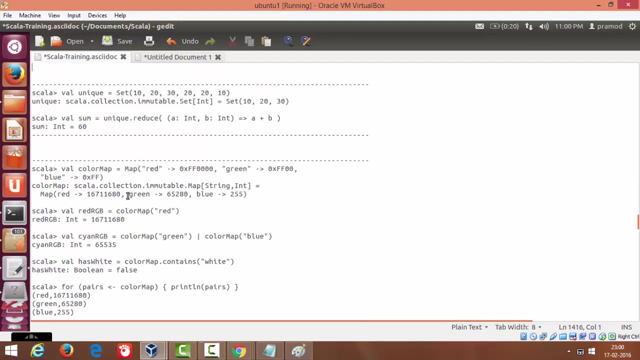 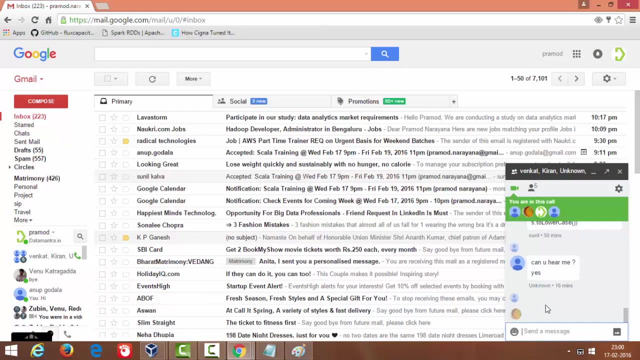 variables. then we saw higher order functions to which function was passed as an argument. then we are seeing higher order function defined on the collections. so this makes more functionality in Scala collection and less to code. yeah, tell me, okay, your voice is echoing. probably you can type. I think we'll stop it here.